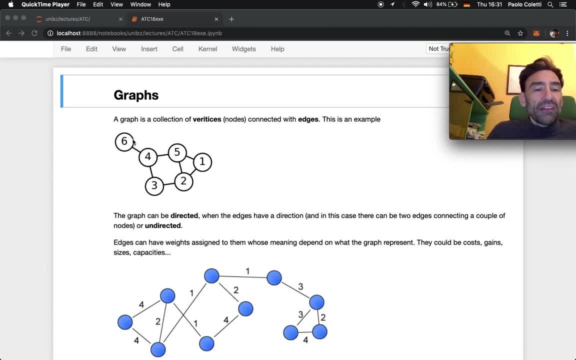 This is an example. A graph can be undirected as this one, So it means that each edge doesn't have any particular direction. So we take it for granted that there is a connection between four edges, Between four and six And between six and four, Or a graph can be directed. In this case. you will see some arrows here. For example, if there is here, there is a connection between four and six, But not between six and four. 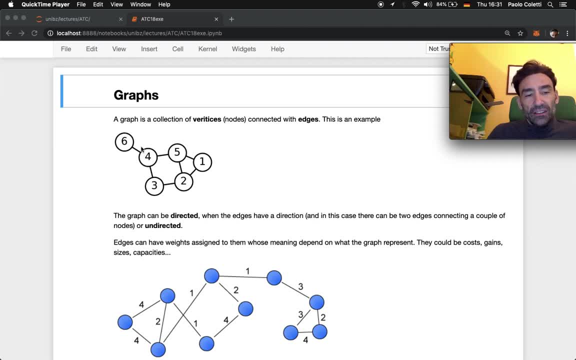 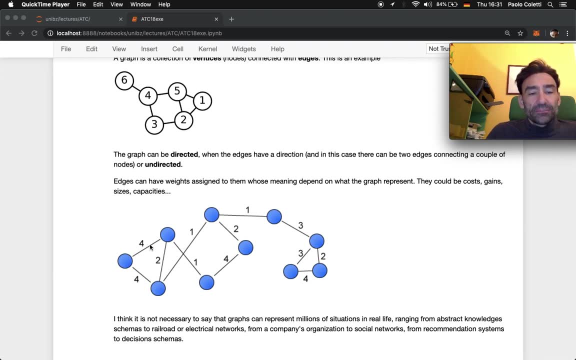 If there is also a connection between six and four, you will see another arrow going in the other direction. Sometimes edges have weights. What do these weights represent? depends On what your graph represents. The weights may be a cost, A distance, Maybe a gain, A size, A capacity of the edge Can be really a lot of things. 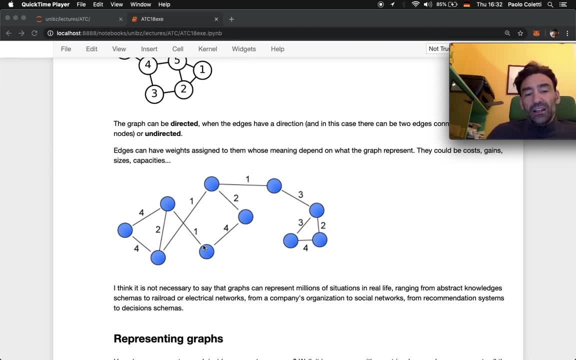 Well, again, it's not necessary that I tell you that a graph can be a data structure which is able to represent millions of real life situations. For example, abstract knowledge, Schemas, Railroads, Electrical networks, A company, A company organization, A social network- It's nothing else but a graph. 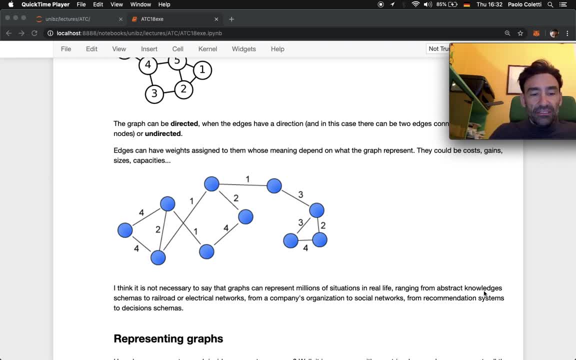 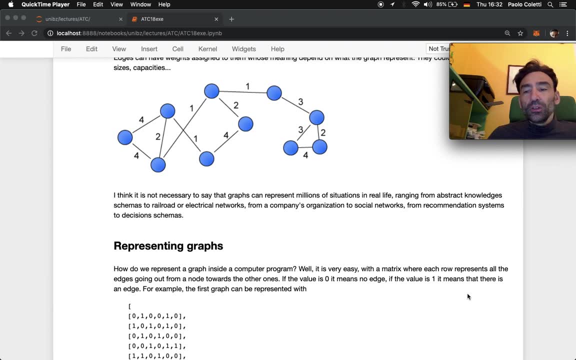 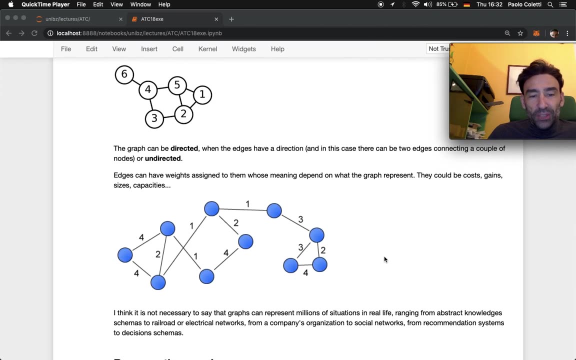 Recommendation of systems, That is, a directed graph, Decision of schemas, Whatever. So a graph can have tons and tons of practical application. How do we represent a graph in a computer algorithm? Well, unfortunately, we cannot have a graph, a picture, a pictorial data structure. 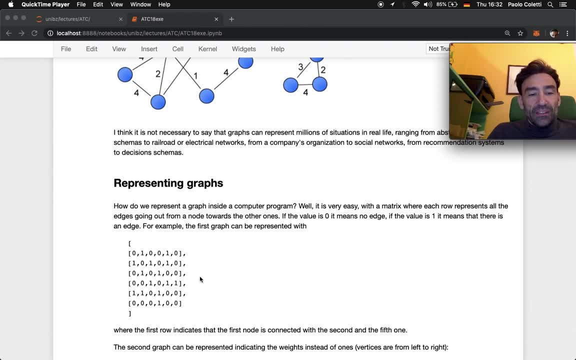 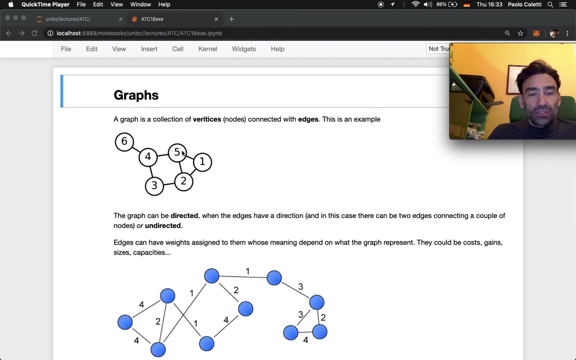 We represent a graph in a very simple way With a matrix Like this: A matrix containing zero, and one Zero means that this row represents the vertices to which the first vertex is connected. So, for example, the first vertex here is connected to the second one and to the fifth. 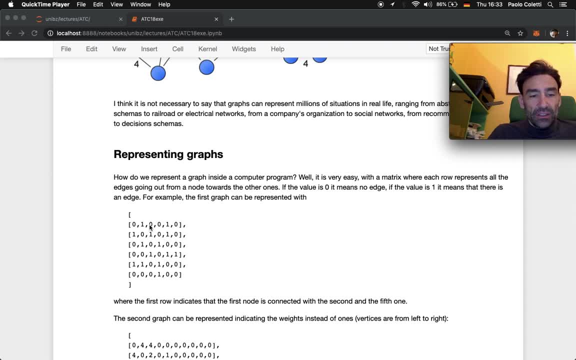 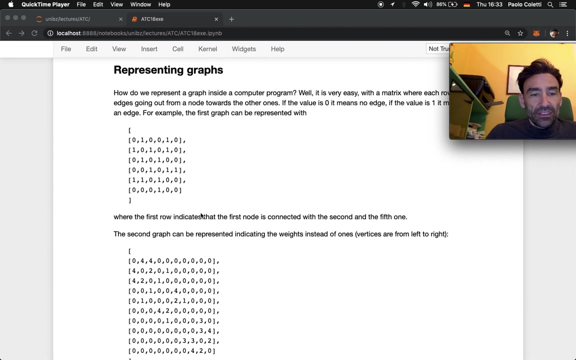 So the first vertex is connected to the second, one, third, fourth, fifth. So there is a one Then at the index i, j, where i is the current vertex and j is the vertex to which it is connected. Here it is the second vertex connected to one, three and five. 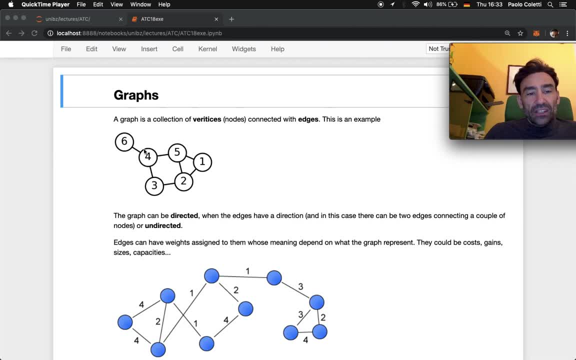 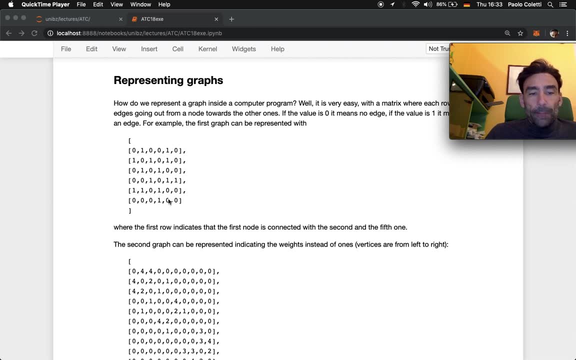 For example, the sixth vertex is connected only to four. So the sixth vertex here is connected only to four. So the sixth vertex here is connected only to four. You see, Right, That's important. OK, OK. So this is a matrix. 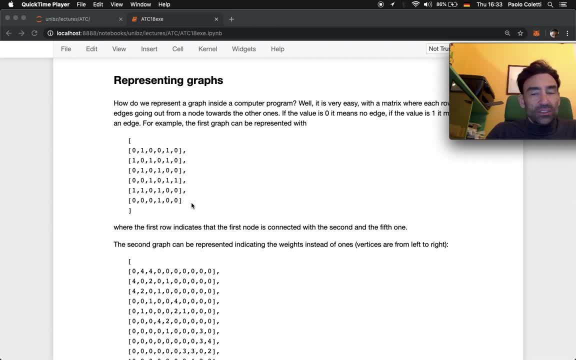 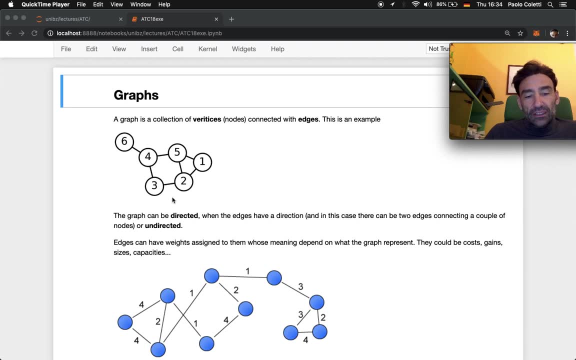 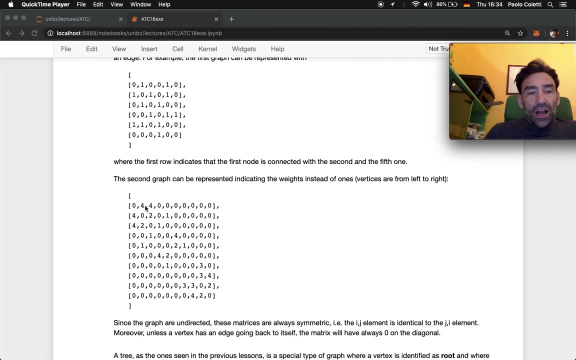 This completely represents a graph. So with a matrix you have full information of the graph. If your graph has weights, It is simple. You can see here: Instead of zero and one, you insert zero when there is no connection. Otherwise you insert the weight of the connection. 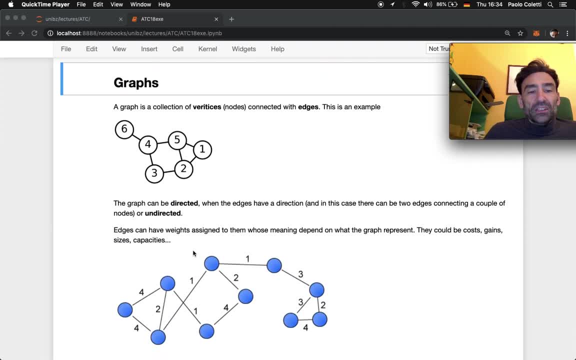 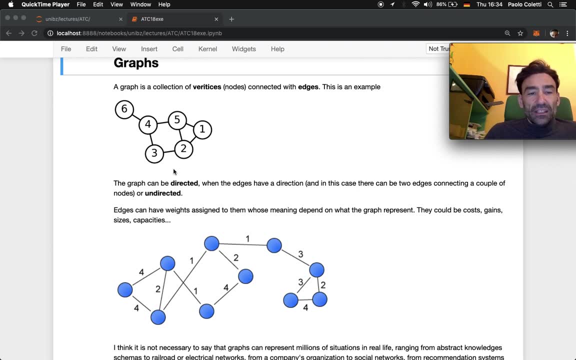 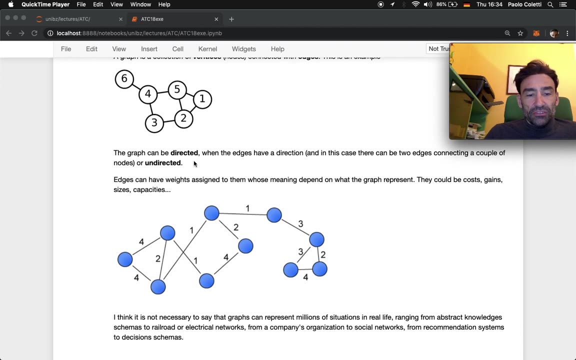 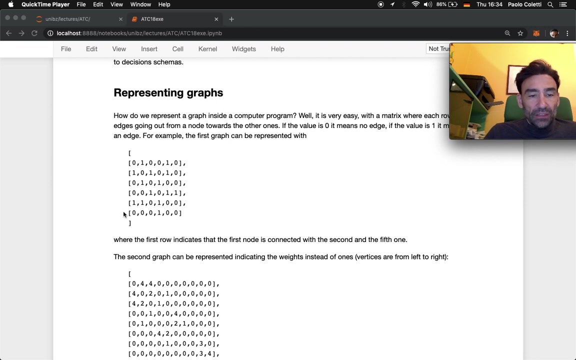 OK. Please note that if your graph is undirected, the matrix is symmetric. So, for example, there is a connection between 4 and 6, and automatically there is also a connection between 6 and 4.. So here there is 4, between 4 and 6, here the 1, and automatically between 6 and 4,. 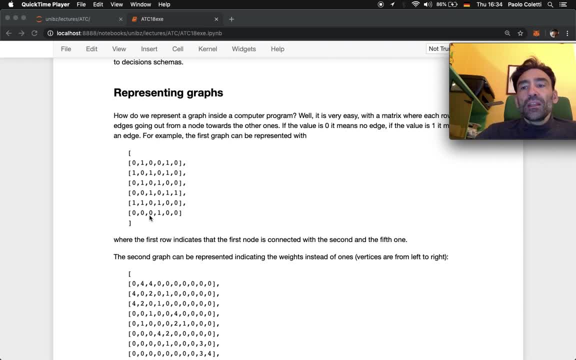 here the 1.. So for graphs which are undirected, the matrix is symmetric. If, instead, your graph is erected, the matrix will not be symmetric. Moreover, please note that on the diagonal, this diagonal, you have all zeros, zero, zero. 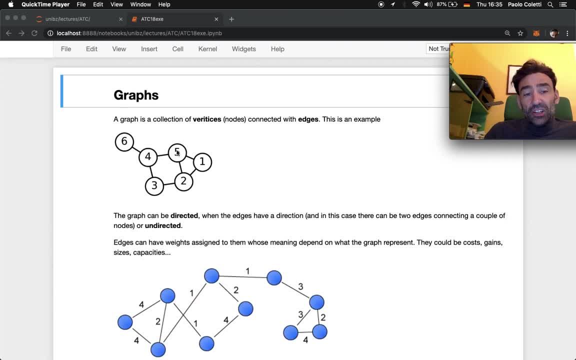 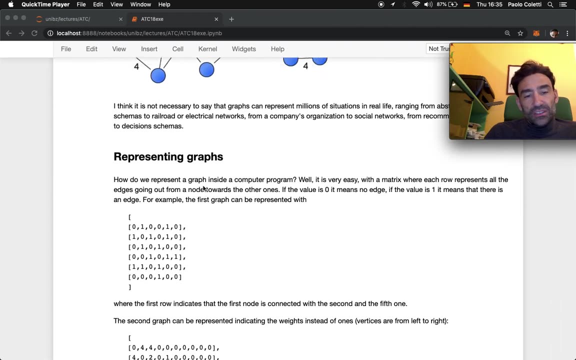 zero, zero, zero, because a vertex is never connected to itself, unless you have particular graphs which have sometimes the connection from starting from 5, going here and going back to 5. In this case you don't have zeros, but otherwise you have always zeros. 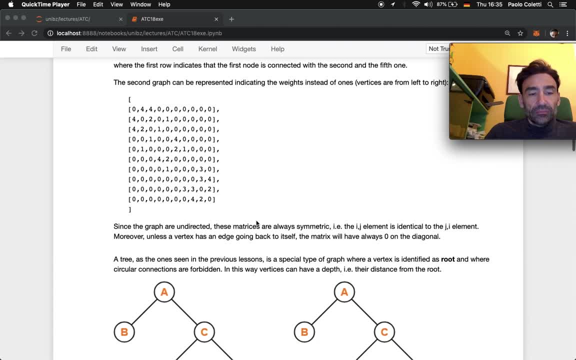 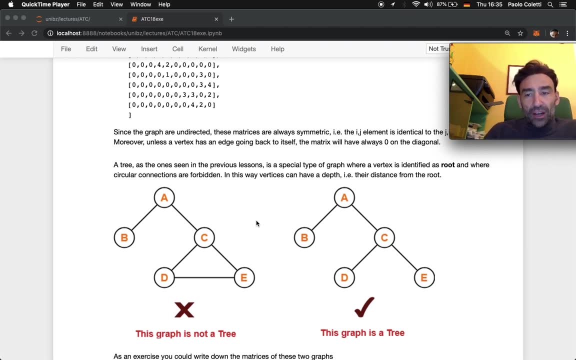 In most of the graphs, you have always zeros on the diagonal. OK, A tree. something we have seen before is a special type of graph. a special type of graph in which, first of all, you identify one of the vertices and call it root, and 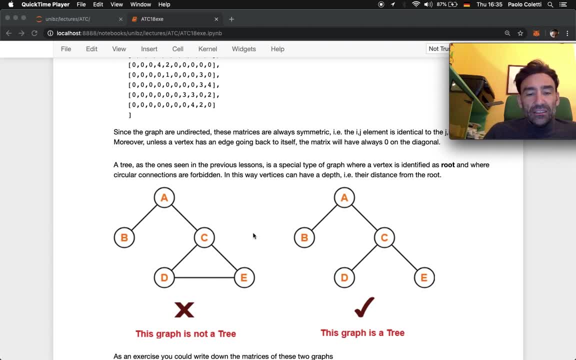 you never have this thing here. cycles, So loops, circular connection. So if C is connected to D and C is connected to E, it's not possible that D is connected to E. So you never have a circular connection in a tree. That's the only difference between a graph and a tree, So a tree does have a circular connection. Moreover, in a tree, usually you identify a vertex as the root, and thus you can talk about the depth. The depth is how many connections. 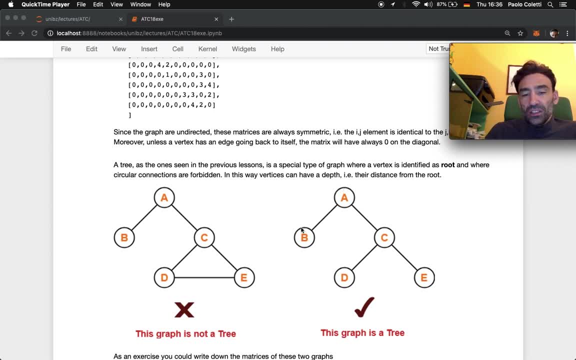 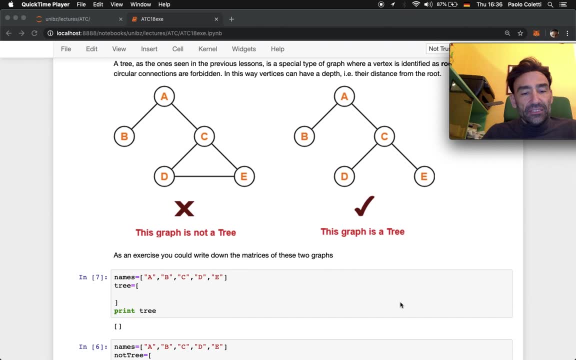 OK, What connection do you need to reach the root? So these are at depth 1, these are at depth 2.. OK, Now, just as an exercise, let's write the matrices of these two graphs here, First of all of the tree. OK, so Alt 5 on the Mac, comma A is connected, not to itself. 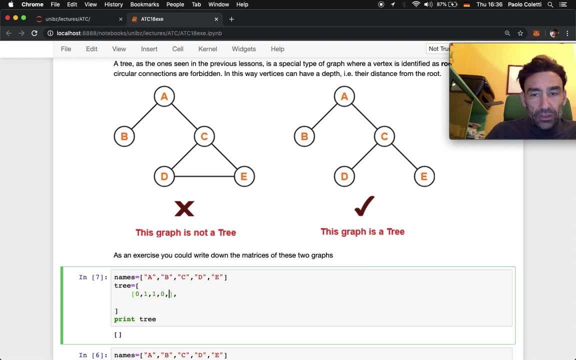 is connected to B. So C is just connected to the C, Not to D, and to C, Not to D, Not to E. Let me take it So: B is connected to A, Not to itself, Not to anything else. C is connected to A. 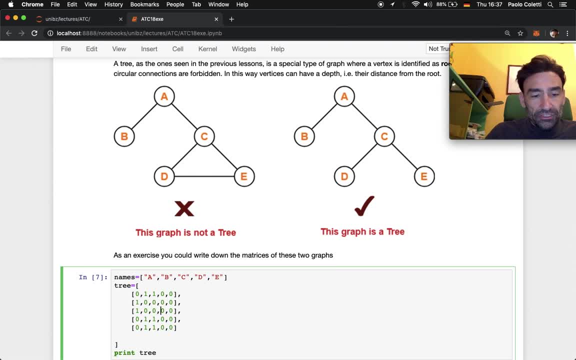 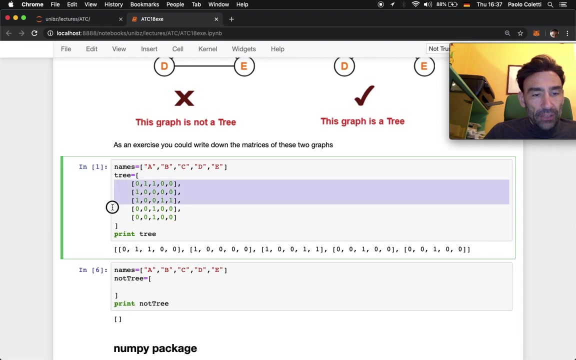 Not to B, Not to itself, To D and to E. If D is connected to A, not to B, commercial, it means that the K by D from today's your day connected to C, and that's it. E is connected to C, that's it. okay, I am lazy. 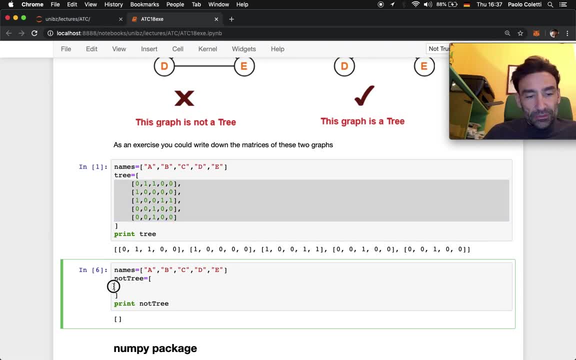 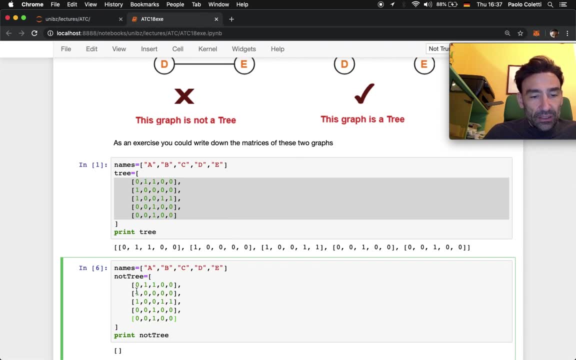 so I copy this one, I just add the missing connection. let's add: the missing connection is between D and E. so A, B, C, D and E here one, but also between E, and D. so easy: A, B, C, D, matrix, and sycrache C이랑 gente metas catalogs, a metric. 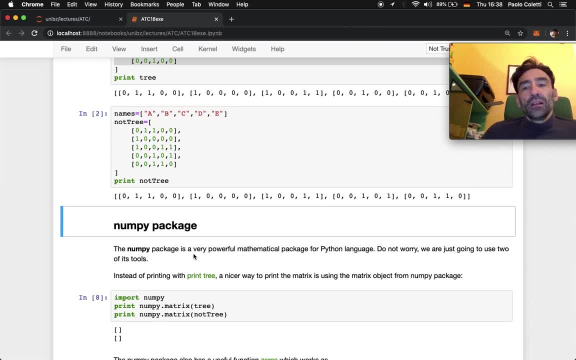 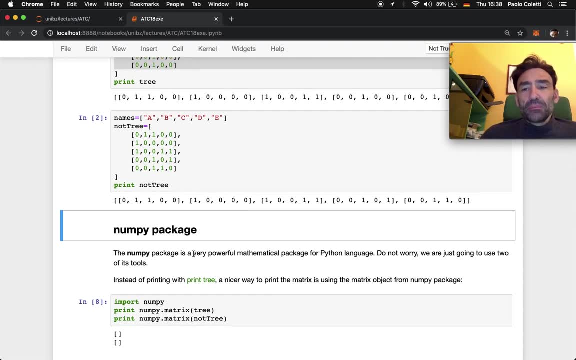 okay, sometimes you need to create a matrix, sometimes you need to create a matrix full of zeros or do things like that. it may come handy to use truth functions from the NumPy package. The NumPy package is a very, very famous and powerful mathematical package for Python language. 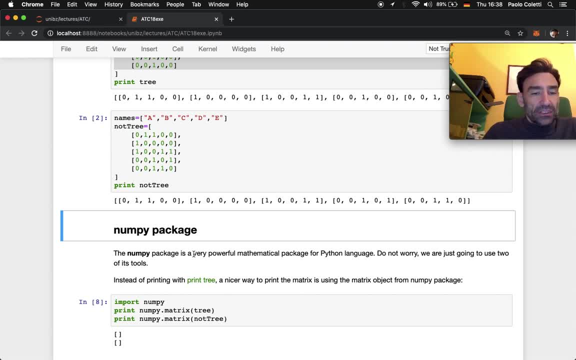 In particular, it contains the matrix object, because these things here that we call matrixes are not real. matrix are lists of lists. A list of lists is in practice a matrix, but in theory it's a list of lists. The NumPy package contains the real matrixes. Don't worry, we will just use two little tools from it. 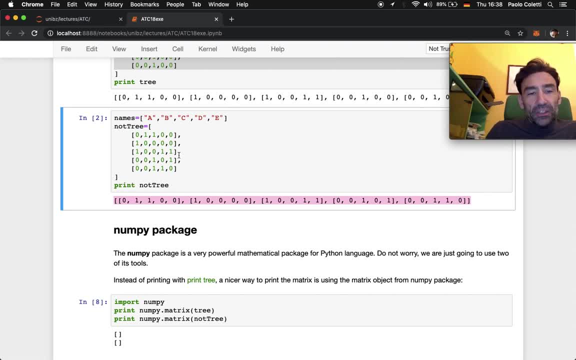 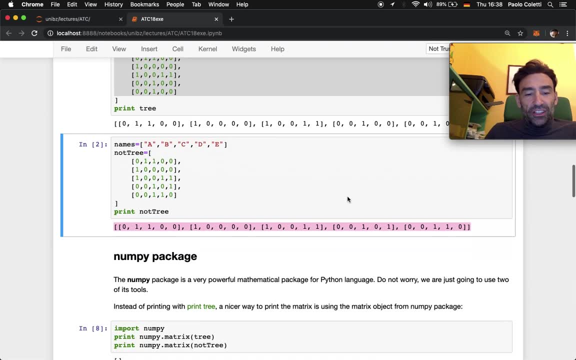 The first one is: you can see, when you print the matrix, you don't see it in a matrix format, you see it in this format, which is not very user-friendly. If instead you import NumPy and you print numpy.3 and the name of your matrix. 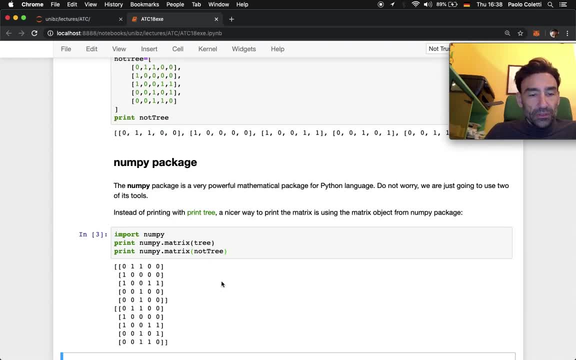 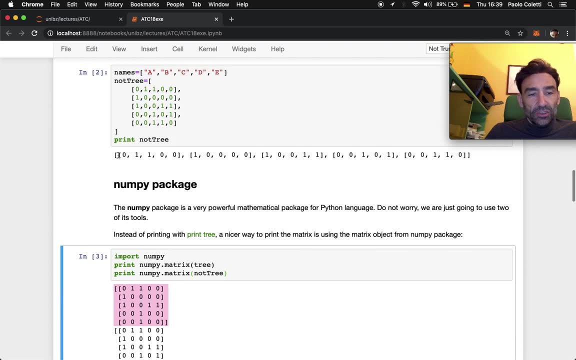 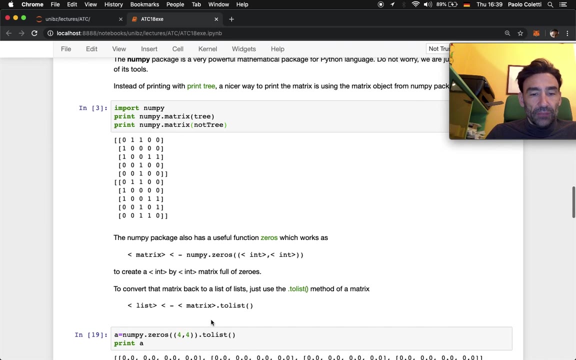 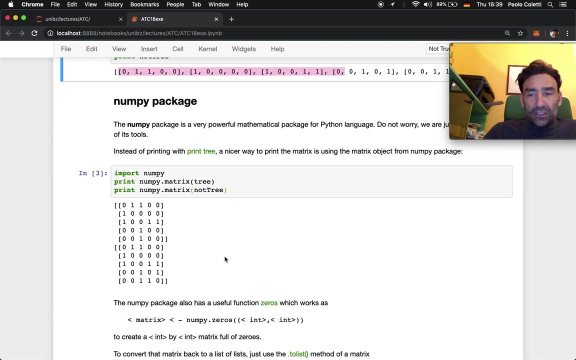 you will see it in a more user-friendly way, Much more user-friendly to see it like this than to see it like this. So the first thing- it's not required, but it may be helpful for you. Then the NumPy is also useful whenever you have to create a matrix full of zeros. 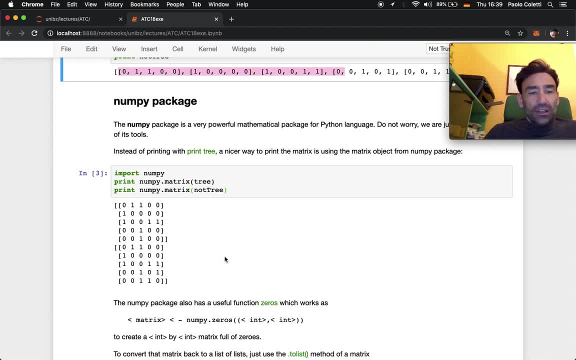 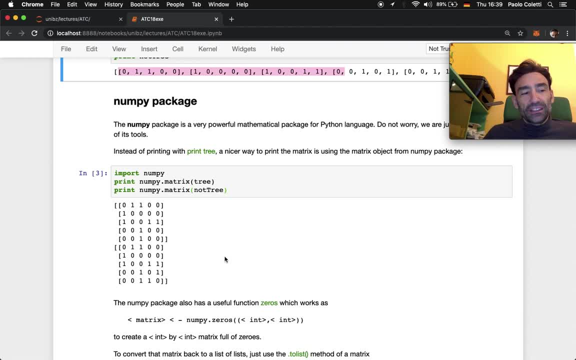 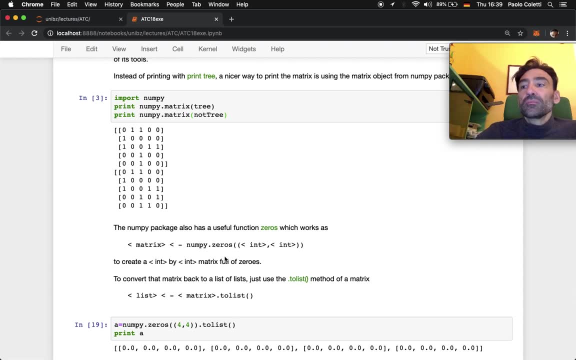 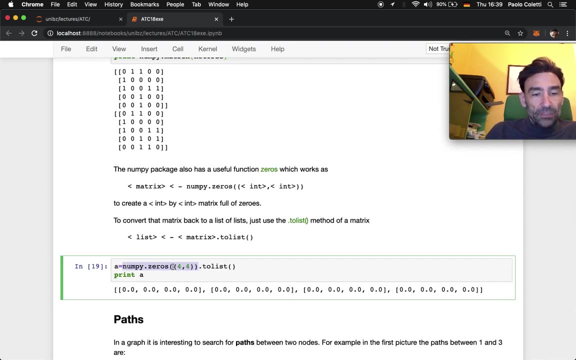 If you have a matrix 20 by 20, you start to have to type at least 20 zeros and copy them 19 times. So let's see how to create with NumPy zeros. Pay attention to the double round parentheses. Open parentheses- open another one. 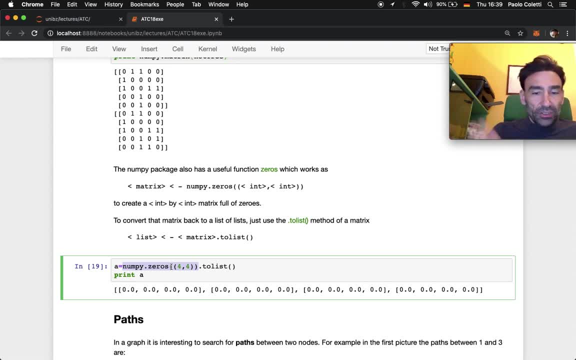 For technical reasons which are beyond the scope of this course. Okay, NumPyzeros, This creates a matrix. okay, a matrix. four by four in this case, but you can have 40 by 40 if you want. full of zeros, only zeros inside. 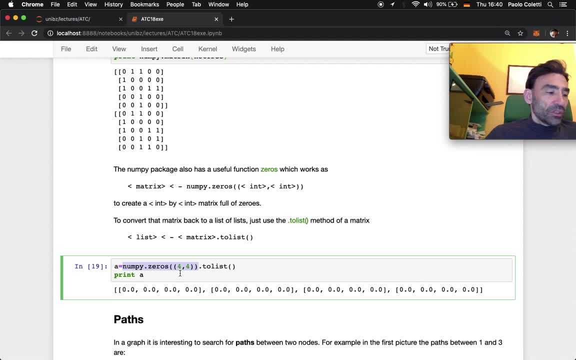 But since we don't use matrixes, we use lists. this method, the method dotToList, converts your matrix into a list. Okay, as you can see. Okay, If you instead remove the dotToList, you have a matrix. can you see? 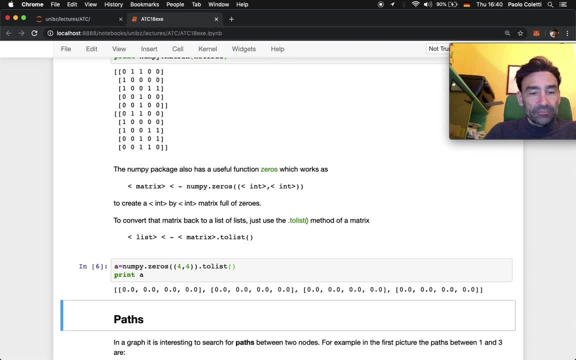 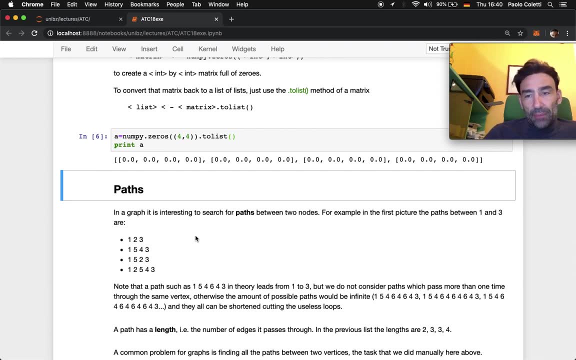 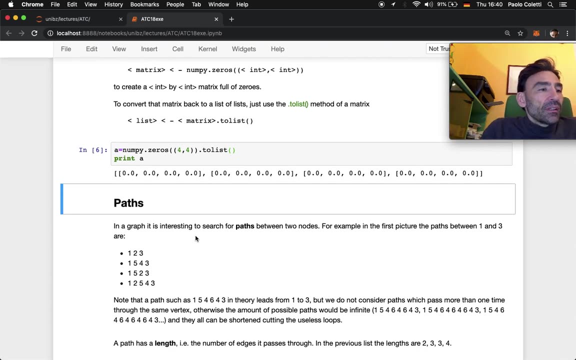 dotToList open. Okay, In theory, in all these algorithms you can work also with a NumPy matrix, but since we started the course using the list of lists, that's fine. Okay, path Inside the graph. it's very interesting, or better. 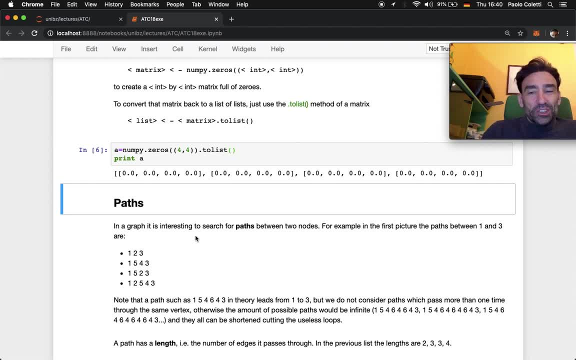 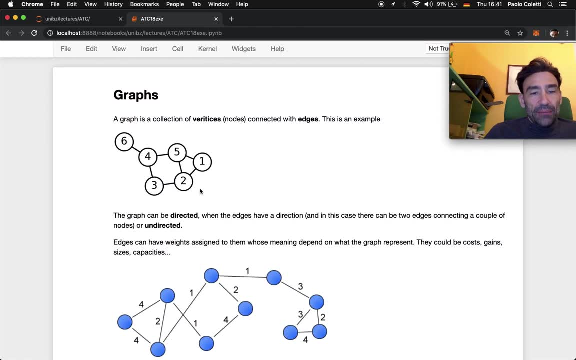 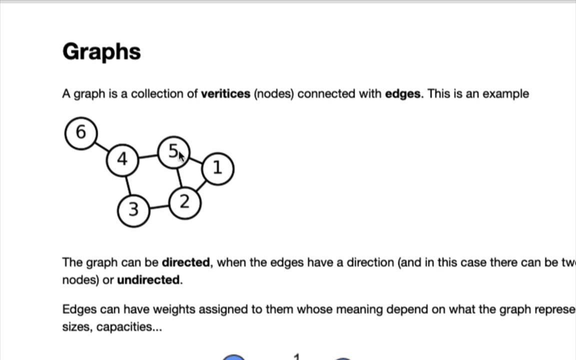 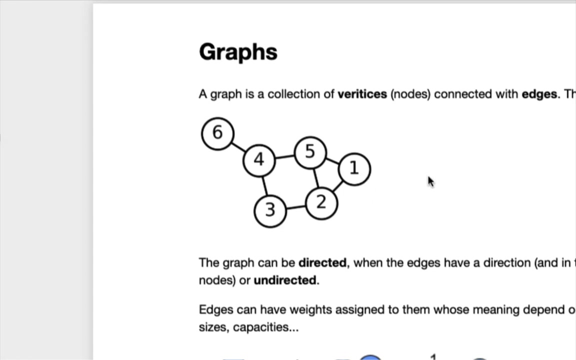 several applications require that you search for paths between two nodes. For example here, Suppose, I ask you, tell me all the paths between node one and node three. So the paths between node one and node three, let's try to find them manually. 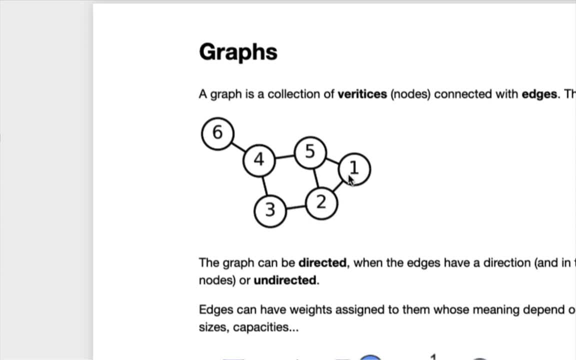 One, two, three, But also one, five, four, five. One, five, four, three, But also one, five, two, three. Let me see whether there are other ones. Ah, there's also one, two, five, four, three. 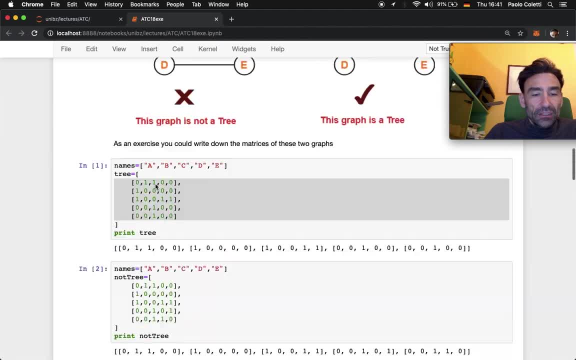 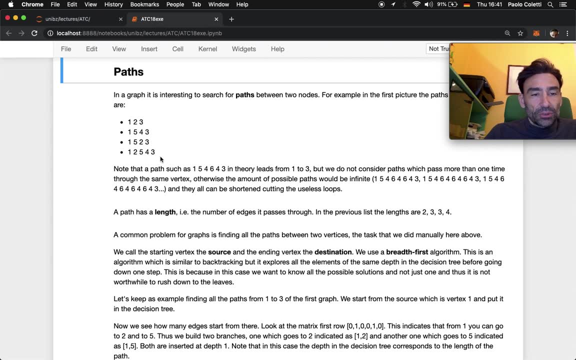 I think these are all the paths from one to three. Let's see my solution here: One, two, three. One, five, four, three. One, five, two, three. One, two, five, four, three. 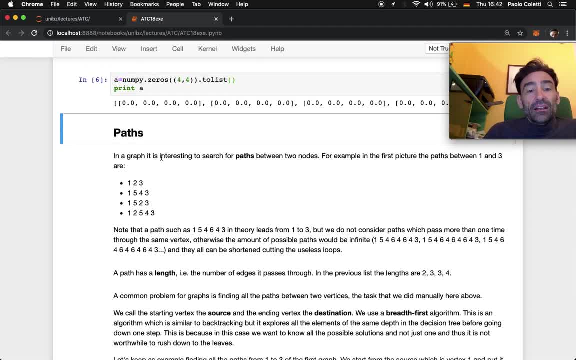 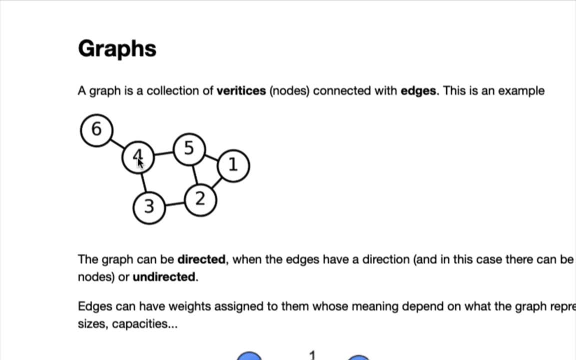 Okay, There are in theory other paths. For example, suppose you can have one, five, four, six, four, three. This path goes from one to three. The problem is that you pass two times through number four. We do not accept paths like this. 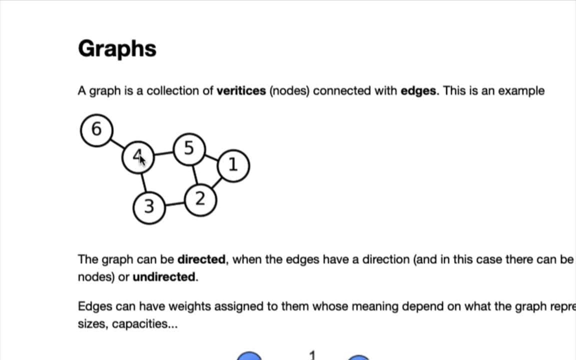 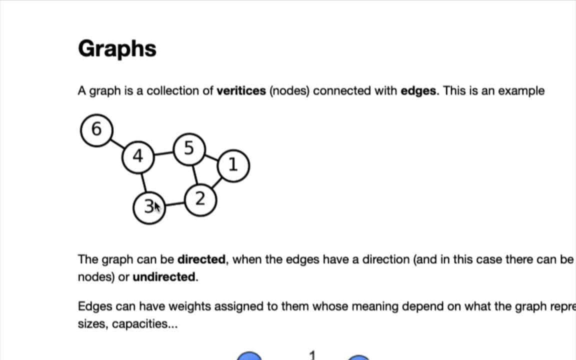 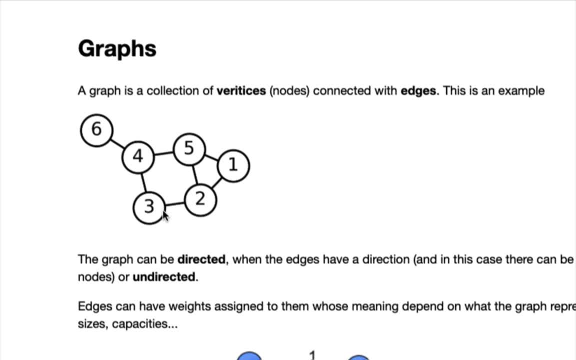 One, two, one, two, one, two, three. So we exclude, we don't call a path a path which passes two times through the same vertex, First of all because otherwise we'll have an infinite amount of paths, But also because that path can be shortened. 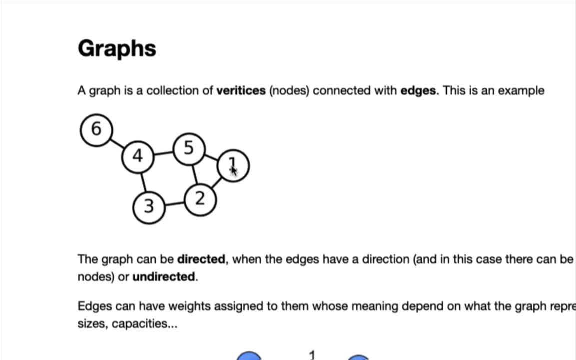 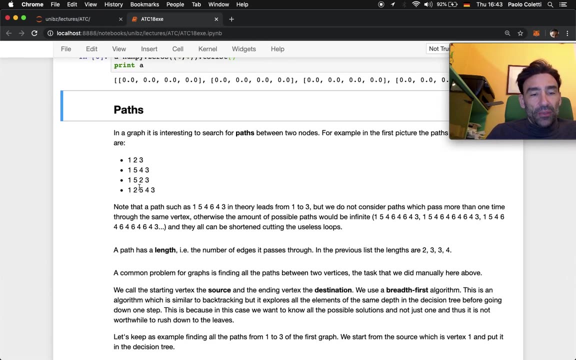 cutting the loop. So paths which make loops are not considered. Also, for example, one, five, two, one not considered. So these are the paths which connect one with three. The path has always a length. This is length two. 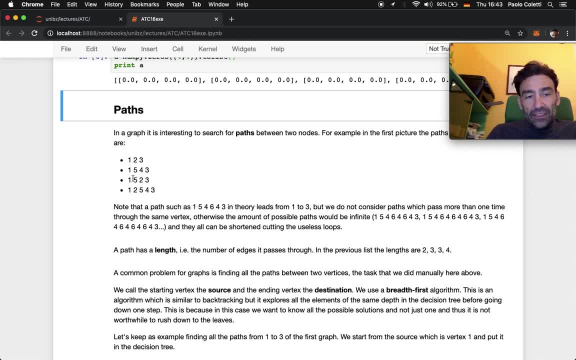 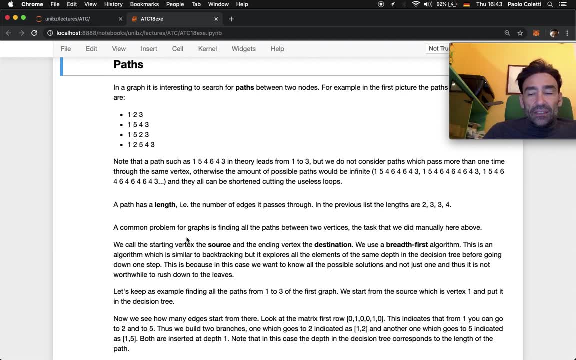 You count the edges, not the vertexes: Length three, length, three. length four. OK, A common task that you find in several applications is finding all. and pay attention, because this time I say all, not one, not the best all. 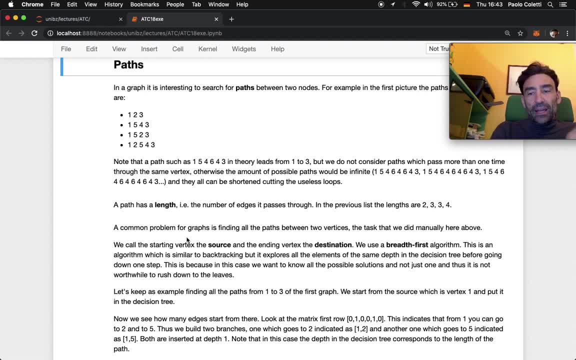 In usually problems, you either have to find the best, the best, or just one solution, or all the solutions. In this case, all. So, find all the paths which start from a source and end in a destination. OK, Let's see. 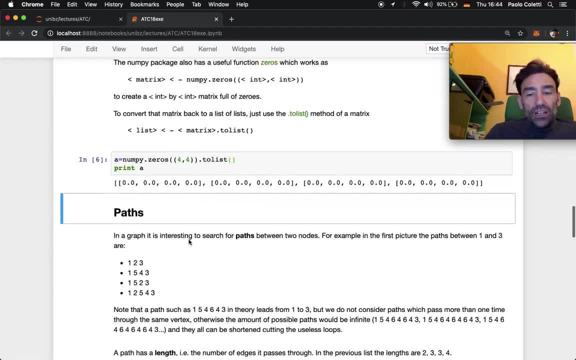 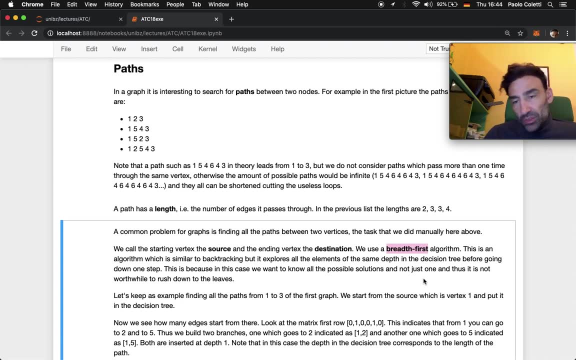 Which kind of algorithm do we use? We use an algorithm which is called breath first. We have seen another algorithm for backtracking which was: we used the backtracking algorithm, which is an algorithm which is an algorithm with depth first, because it's an algorithm which has to find one solution. 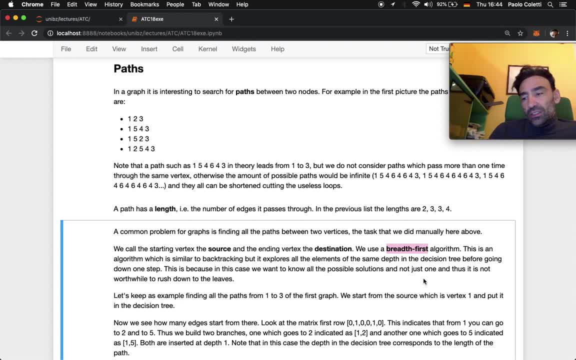 So it goes deep down to search for an immediate solution, and then, in case it goes up, so backtracking This algorithm here, the one which finds all the paths inside a tree, it's breath first, because this one doesn't have to find one solution. 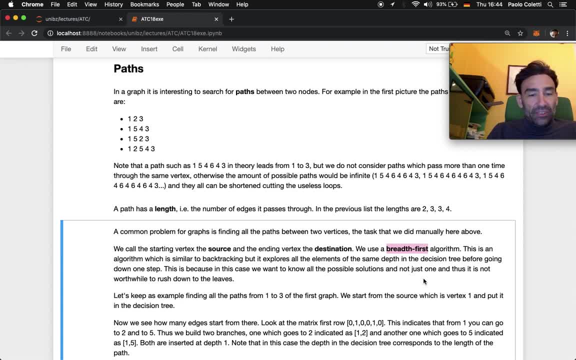 it must find all of them, So there is no way it will have to explore everything. So, before going down into the decision three, it will explore everything. So while the backtracking explores always the deepest solution, the branch and bound explores always the best solution. 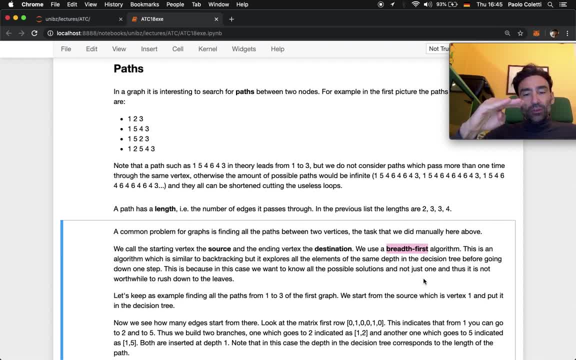 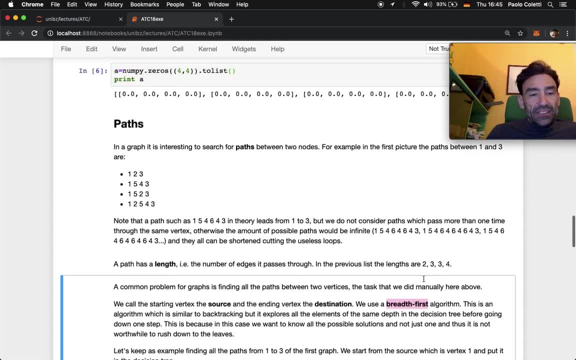 this, one must find all the solutions. so, before going down one level, one depth level explores all the solutions. OK, Let's keep this example. so the path from one to three. OK, And let's see how the algorithm works. 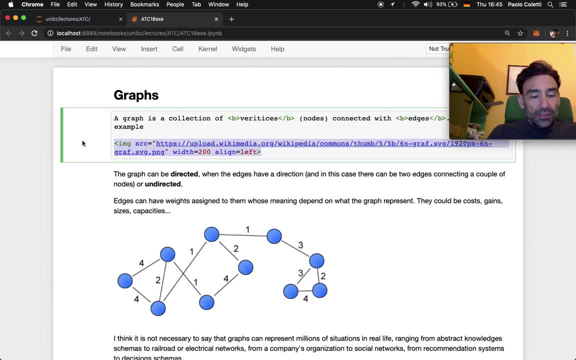 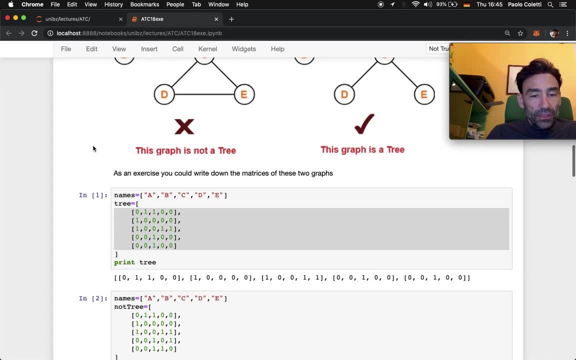 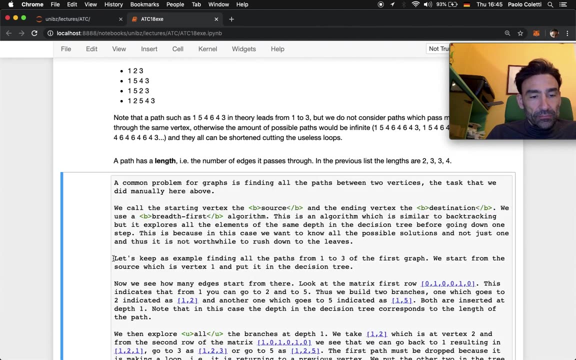 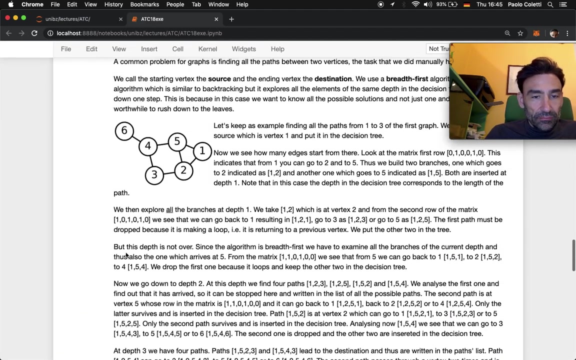 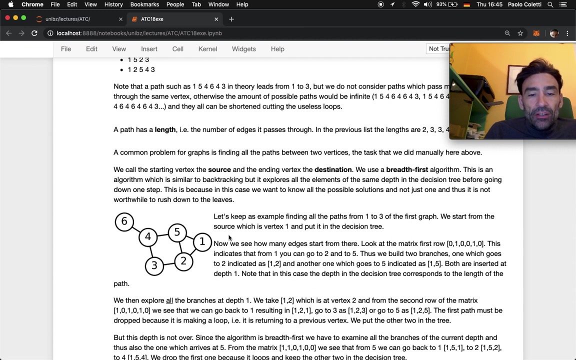 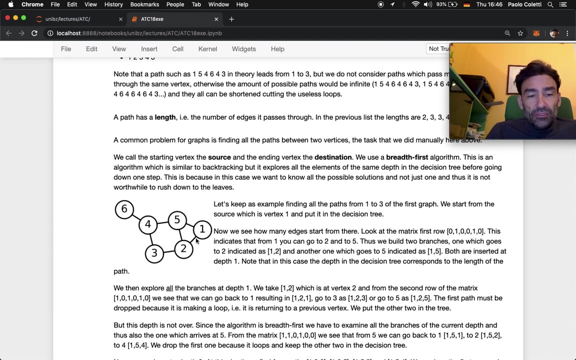 By the way, let me take this thing, Come and see And copy it here because I need it, OK, OK. so first of all we start from one, So from one to three. First of all we start from one. 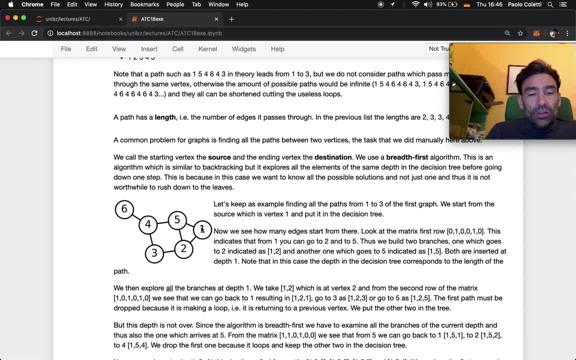 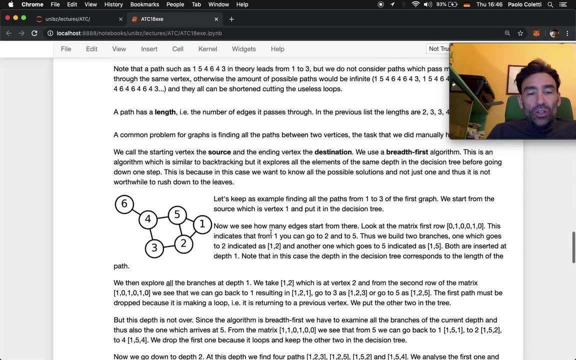 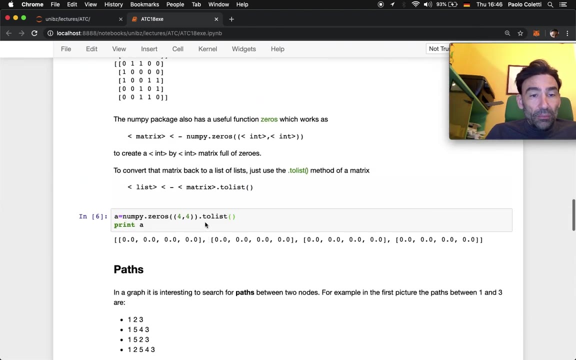 OK, Now our algorithm wants to know. so the path currently is one, Nothing else. I am in one, nothing else. It's here mean one, nothing else. the path now wants to know to which other vertices is vertex one connected. how do we know? well, we go above looking at the matrix here. 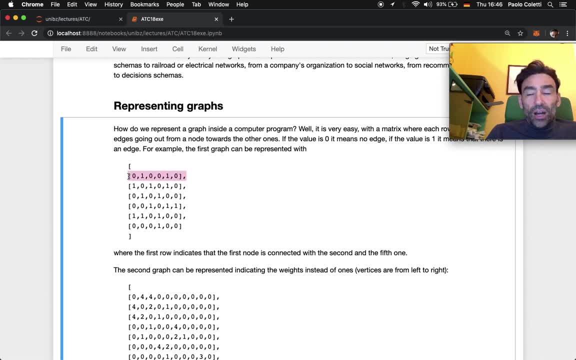 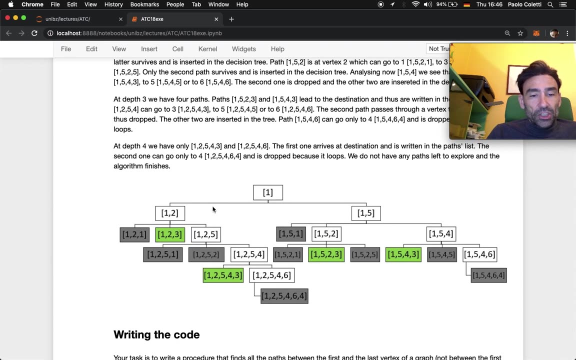 from the matrix, from the first row, because you are currently in node one but the first row- you can see that node one is connected to node two and to node five. so here we branch and we take two paths: one which starts from one and goes to two, another one which starts from one and goes to five. ok, now we go down one. 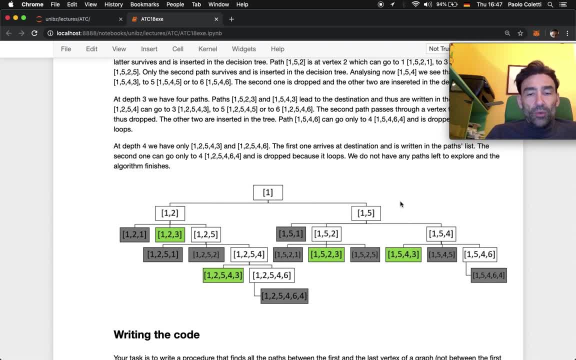 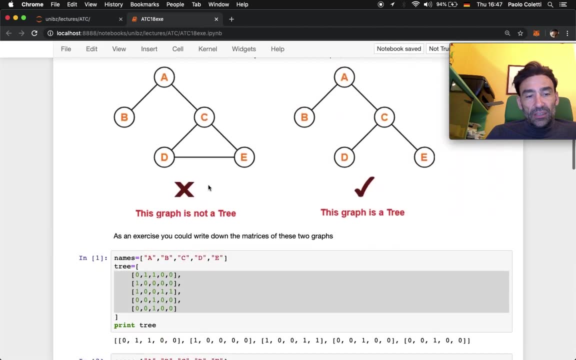 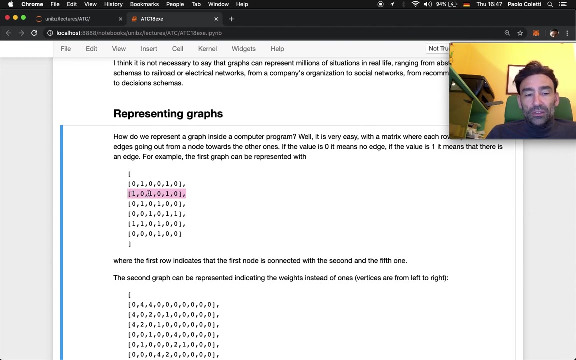 depth level. ok, we are here at depth one and we consider this to path one. two, from node two. where can we go? well, from the picture, from node 2 we can go back to 1 to 3 and to 5. this is equivalently written in the matrix. from node 2, you can go to node 1 to node 3, to. 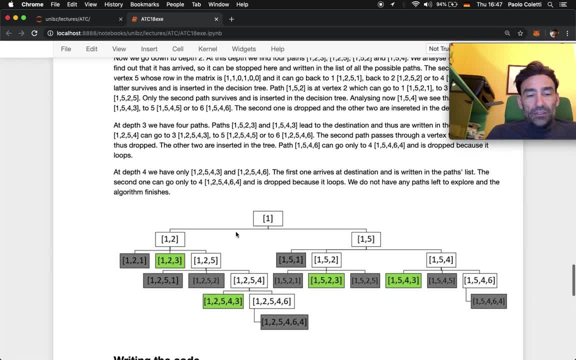 node 5 and here from node 2 you can go to node 1, to node 3 and to node 5. but pay attention, because you cannot really go to node 1, because you can see 1 to 1, it's a loop, you pass two times to the same node. so whenever you have you, 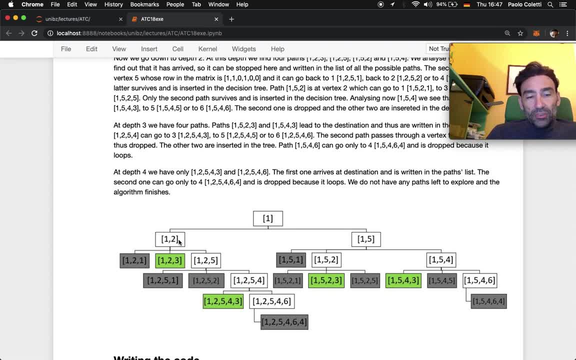 insert a number which is already contained in the previous part of the path. don't insert it, so this one will not even be inserted inside. so we can go only to 1 to 1, to 3 with 1 to 3 or to 5 with 1 to 5: 1- 5. where can 1: 5 go? 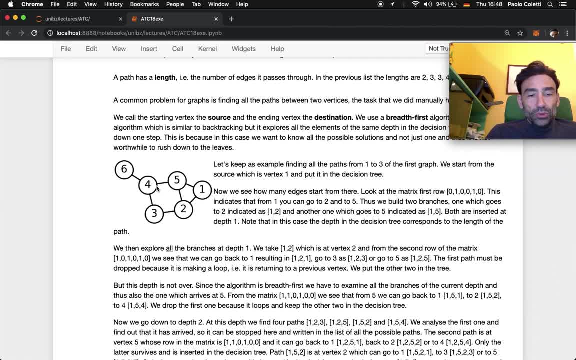 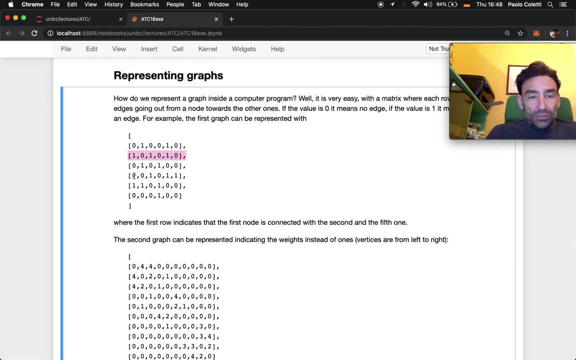 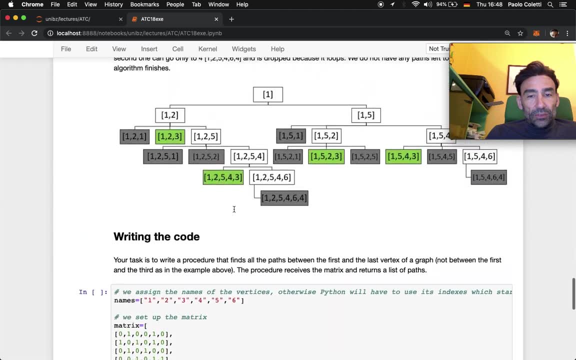 can see it also from the matrix above: so one, two, three, four, five. matrix above: so one, two, three, four, five. matrix above: so one, two, three, four, five, five can go to 1 to 2 or to 4, so to 1. five can go to 1 to 2 or to 4, so to 1. 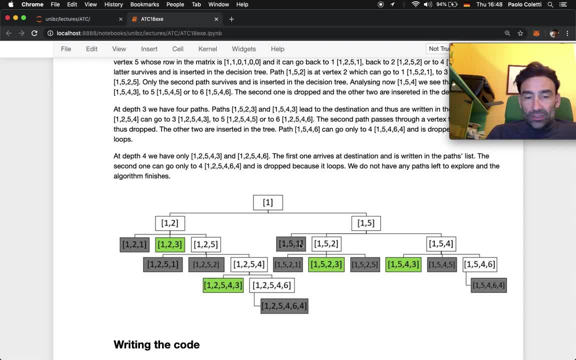 five can go to 1 to 2 or to 4, so to 1: same thing. 1 5 1. it's not good because same thing 1 5 1. it's not good because same thing 1 5 1. it's not good because you are going to a vertex which you 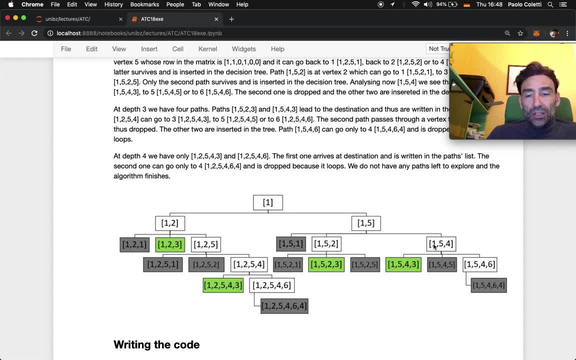 you are going to a vertex which you you are going to a vertex which you have already passed through: 1, 5, 2 and 1, 5 have already passed through 1, 5, 2 and 1, 5 have already passed through 1, 5, 2 and 1, 5, 4. okay, so we have four branches open. 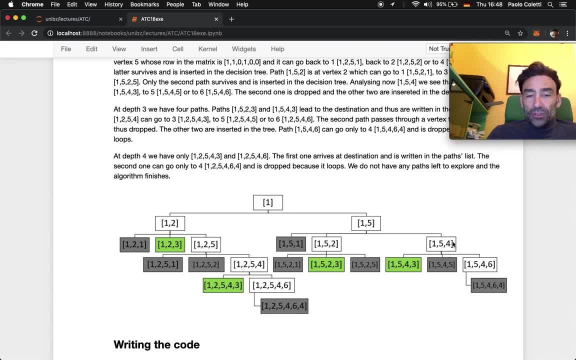 4. okay, so we have four branches open: 4- okay, so we have four branches open: 1 2, 3, 1, 2, 5, 1 5, 2 and 1 5, 4. now we can. 1 2, 3, 1 2, 5, 1 5, 2 and 1 5, 4. now we can. 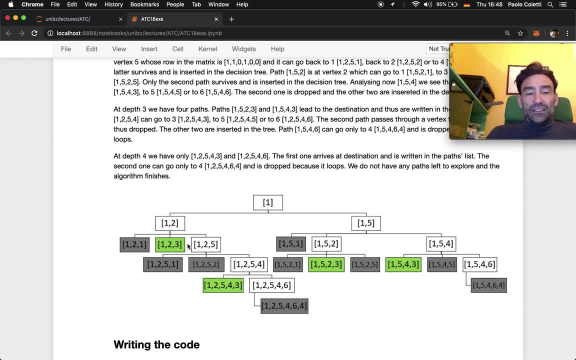 1, 2, 3, 1 2, 5, 1 5 2 and 1 5 4. now we can. you see why it's called breath first. you see why it's called breath first. you see why it's called breath first, because it doesn't go down and down and 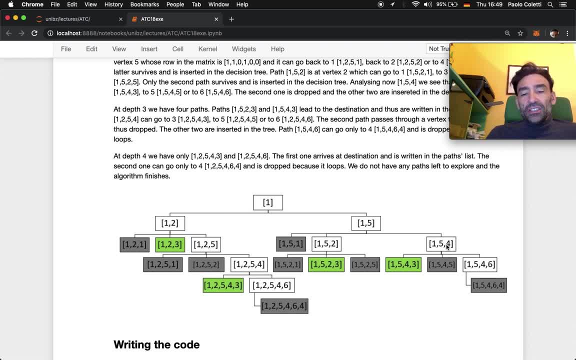 because it doesn't go down and down, and because it doesn't go down and down and down and down, it tries to open all the down and down and down. it tries to open all the down and down. it tries to open all the branches here, before going down one step. 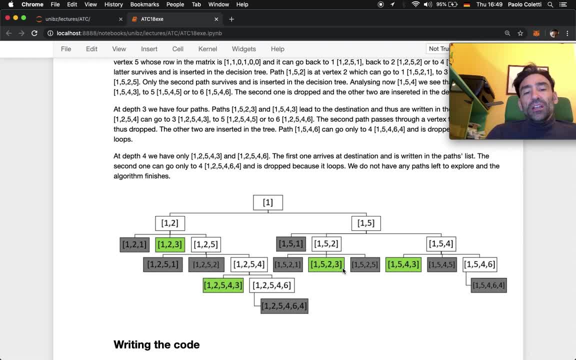 branches here before going down one step. branches here before going down one step: this kind of I go. it's a pretty. this kind of I go. it's a pretty. this kind of I go, it's a pretty dangerous because if you have several dangerous because if you have several. 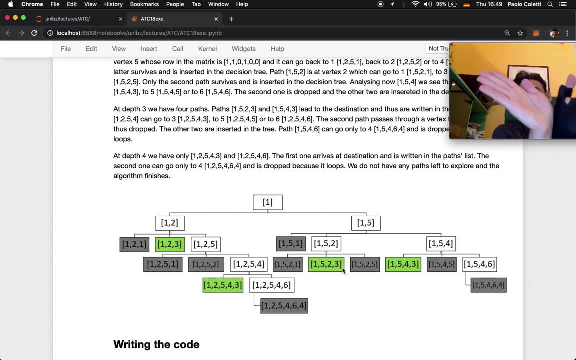 dangerous because if you have several branches, well, very soon, your your tree branches. well, very soon your your tree branches- well, very soon, your your tree become extremely wide and you will never become extremely wide and you will never become extremely wide and you will never be able to go down quickly. however, this 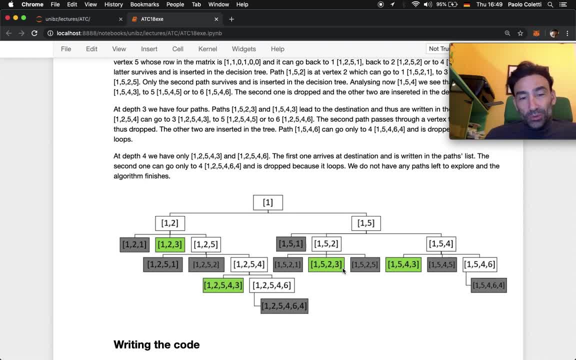 be able to go down quickly. however, this, be able to go down quickly. however, this the disadvantage of whenever you have to. the disadvantage of whenever you have to. the disadvantage of whenever you have to find all the solutions. okay, now let's find all the solutions. okay, now let's. 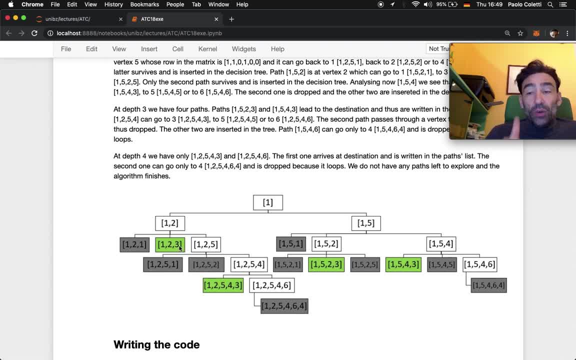 find all the solutions. okay, now let's analyze these four branches: 1, 2, 3. 1, 2, 3. analyze these four branches: 1, 2, 3. 1, 2, 3. analyze these four branches: 1, 2, 3. 1, 2, 3. pay attention, the last node is our. 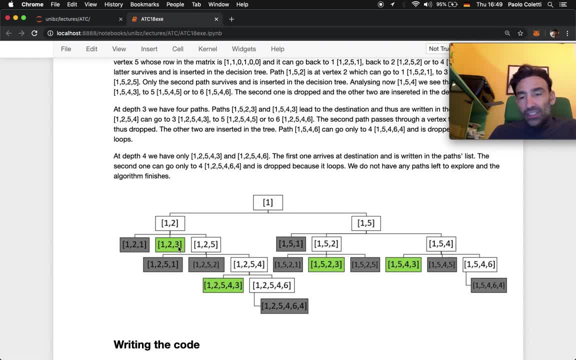 pay attention. the last node is our pay attention. the last node is our destination, so we stop. 1, 2, 3 is a destination, so we stop. 1, 2, 3 is a destination, so we stop. 1, 2, 3 is a solution. we take it and put it inside. 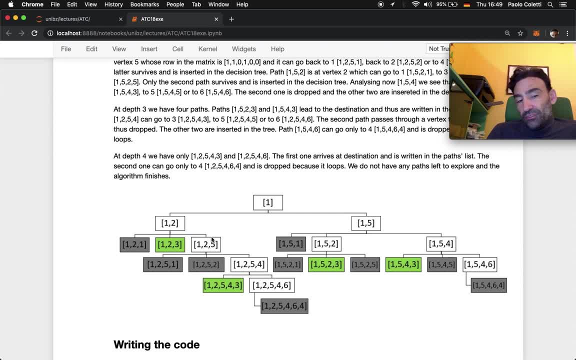 solution: we take it and put it inside solution: we take it and put it inside the solution: 1 2, 5, 5 is not our. the solution 1 2, 5, 5 is not our. the solution 1 2, 5, 5 is not our destination. so we see where can we go. 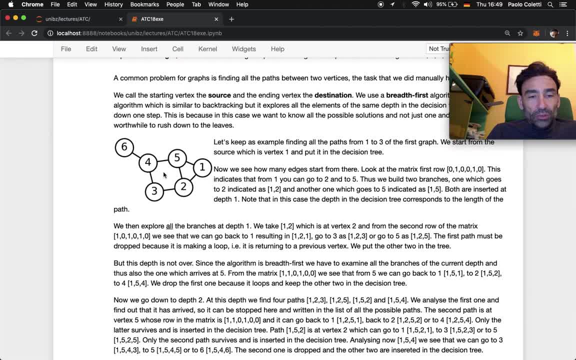 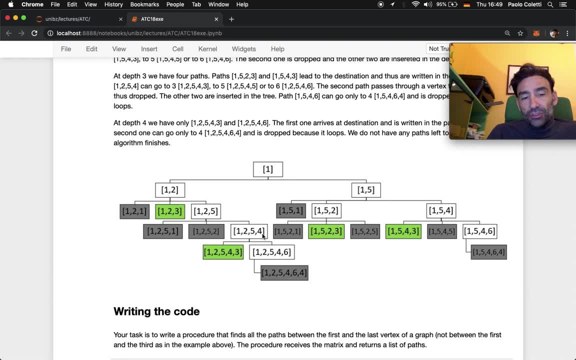 destination. so we see where can we go. destination, so we see where can we go from 5. from 5 we can go to 1 to 2 and to from 5. from 5 we can go to 1 to 2 and to. from 5 we can go to 1 to 2 and to 4. so 1 2, 5. 1, 1, 2, 5, 2, 1, 2, 5, 4, this one. 4, so 1, 2, 5. 1, 1, 2, 5, 2, 1, 2, 5, 4. this one: 4, so 1 2 5. 1, 1, 1, 2, 5, 2, 1, 2, 5, 4. this one passes to a node and or a to our. 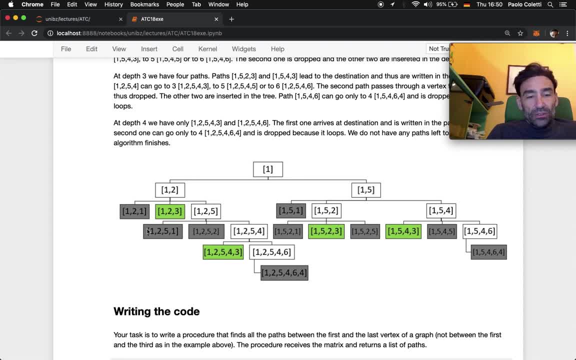 passes to a node and or a to our passes to a node and or a to our vertex that we have already examined this vertex, that we have already examined this vertex, that we have already examined this. one same thing. so we don't even insert. one same thing. so we don't even insert. 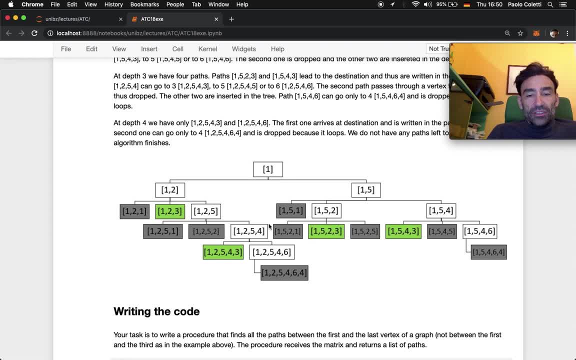 one same thing, so we don't even insert them. 1 2 5 4 is the only one which them 1 2 5 4 is the only one which them 1 2 5 4 is the only one which survives. 1 5 2. 1 5 2 from 2. where can we? 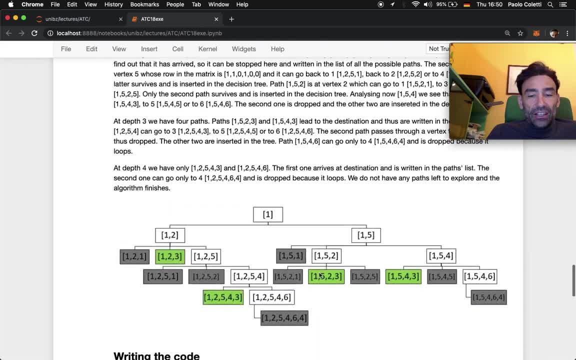 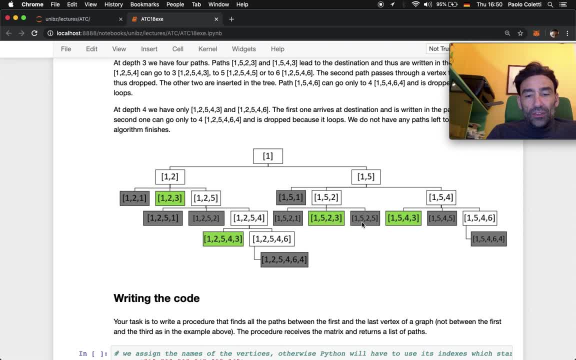 go from 2 to 1 to 3 and 2, 5. 1. go from 2 to 1 to 3 and 2. 5. 1, 2, 1, 5, 2. 1, 1, 5, 2, 3, 1, 5, 2, 5. this one and this. 2 1 1, 5, 2 1, 1, 5, 2, 3, 1, 5, 2, 5. this one and this: 2 1 1 5, 2. 1, 1, 5, 2, 3, 1, 5, 2, 5. this one and this one must be dropped because you. 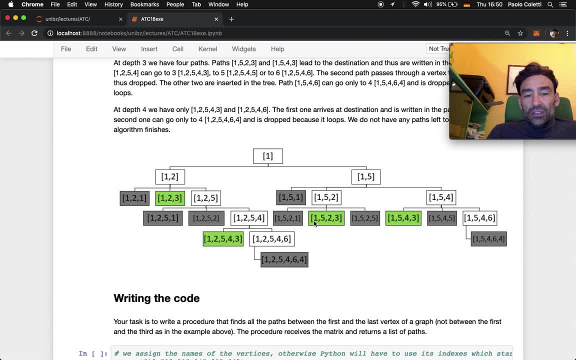 one must be dropped because you. one must be dropped because you passed to a node which is already considered. passed to a node which is already considered. passed to a node which is already considered until the remaining one is 1, 5, 2. until the remaining one is 1, 5, 2. 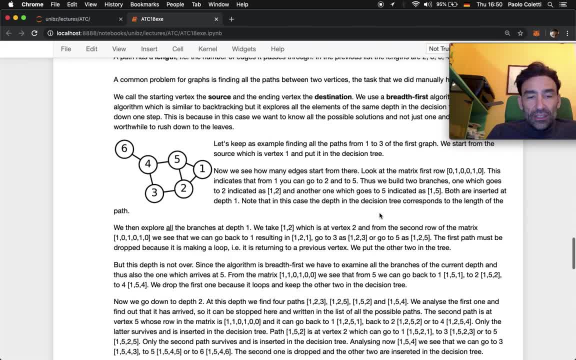 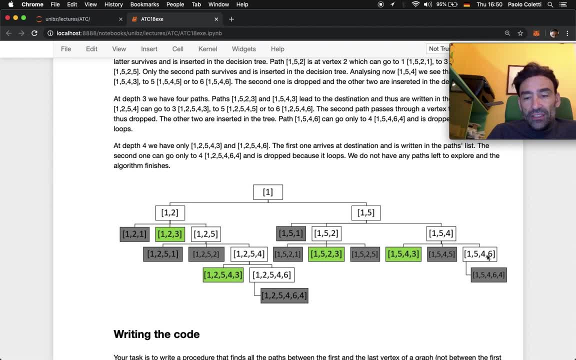 until the remaining one is 1, 5, 2, 3, 1, 5, 4. let's see, from 4 you can go to 3, 3, 5 and 6, 3, 5 and 6, 5. drop it, so we have. 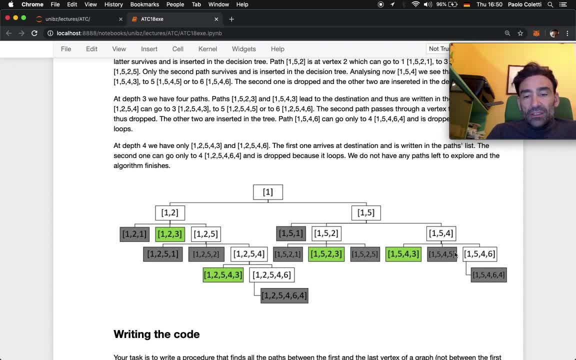 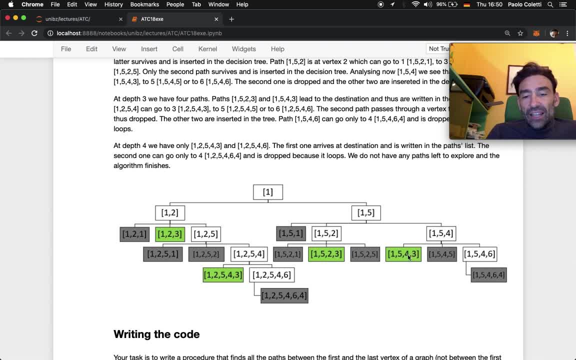 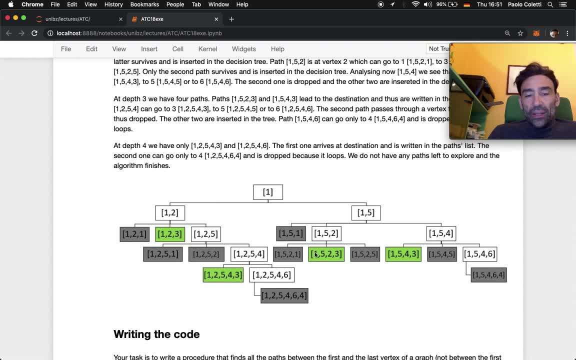 they go this to go into the solution, they go this to go into the solution Lister- okay, so we have open only this Lister. okay, so we have open only this Lister. okay, so we have open only this shoe. so I found three solutions. shoe. so I found three solutions. 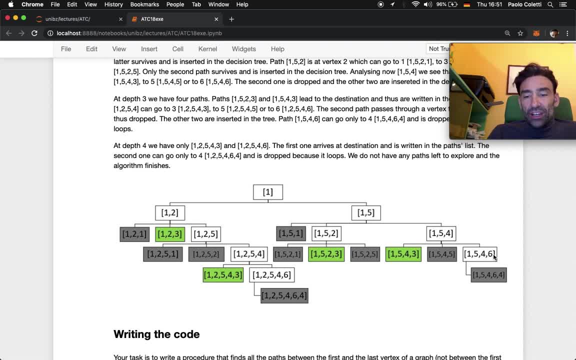 shoe. so I found three solutions currently and open: 1 2, 5, 4 and 1 5 4, 6. currently and open: 1 2, 5, 4 and 1 5 4 6. currently and open: 1 2, 5, 4 and 1 5 4, 6. okay, 1 2, 5, 4 from 4. where can we go we? 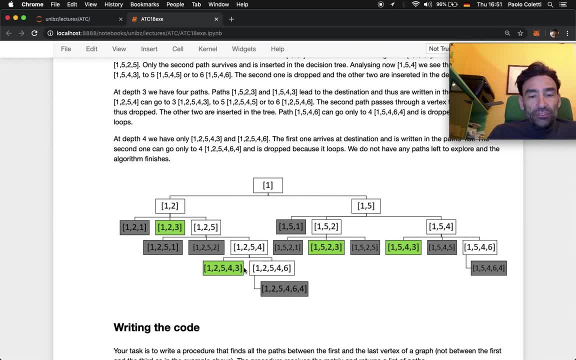 okay, 1, 2, 5, 4 from 4. where can we go? we okay, 1, 2, 5, 4 from 4. where can we go? we can go to 3 to 5 into 6- oops, I forgot to. can go to 3 to 5 into 6- oops, I forgot to. 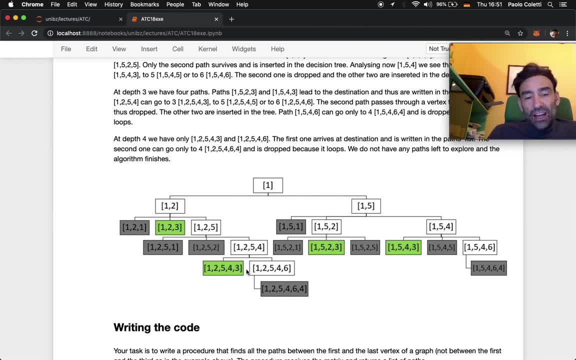 can go to 3 to 5 into 6. oops, I forgot to go to 5. so we can go to 3 to 5, which I go to 5. so we can go to 3 to 5, which I go to 5. so we can go to 3 to 5, which I forgot. but doesn't matter because it. 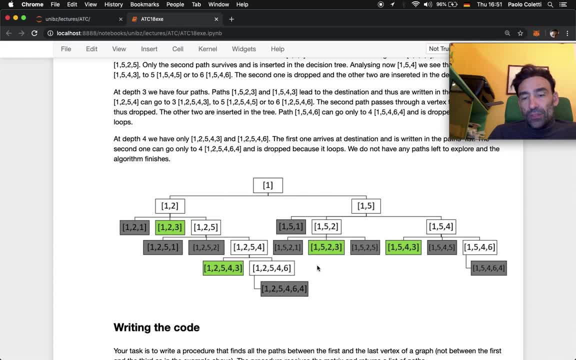 forgot, but doesn't matter, because it forgot, but doesn't matter because it would have been dropped. or to 6 and 1, 5 would have been dropped, or to 6 and 1, 5 would have been dropped, or to 6 and 1, 5, 4, 6. where can it go? well, once you are in. 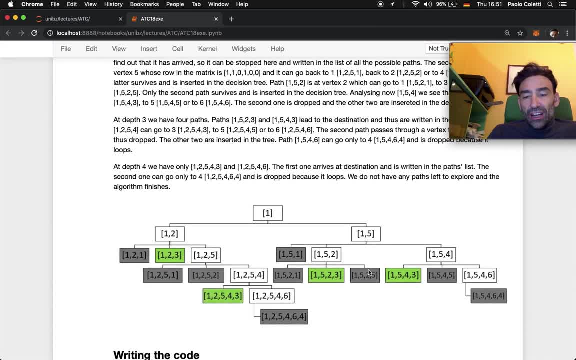 4, 6. where can it go well once you are in 4, 6. where can it go well once you are in 6? you can only go back to 4, so 1, 5, 4, 6, 4, 6. you can only go back to 4, so 1, 5, 4, 6, 4. 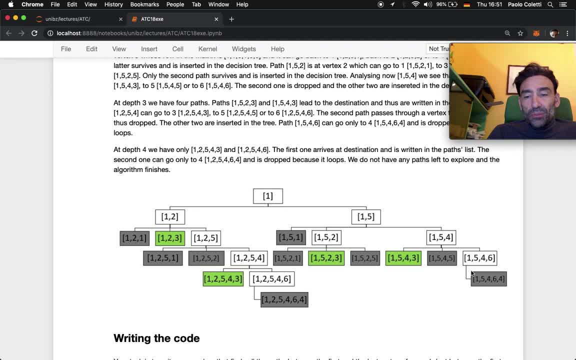 6. you can only go back to 4. so 1, 5, 4, 6, 4, the one which is not written here and the one which is not written here and the one which is not written here- and this one will be missed- will be dropped. 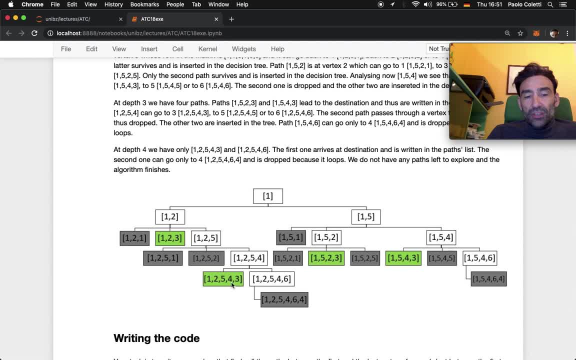 this one will be missed, will be dropped. this one will be missed, will be dropped, and we have only two remaining of these, and we have only two remaining of these, and we have only two remaining of these. two: this one is evidently a solution. two: this one is evidently a solution. 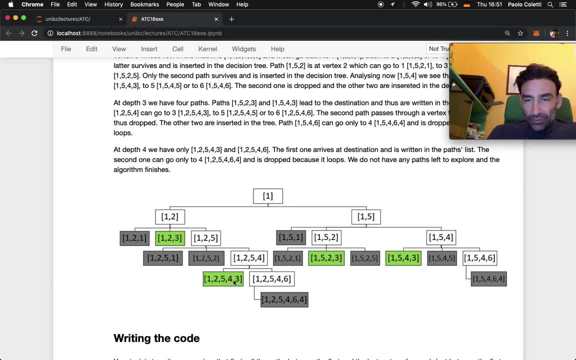 two. this one is evidently a solution because it arrives at node 3. because it arrives at node 3, because it arrives at node 3, very well, and we'll go into the solution very well, and we'll go into the solution very well and we'll go into the solution list and this one is the only one open. 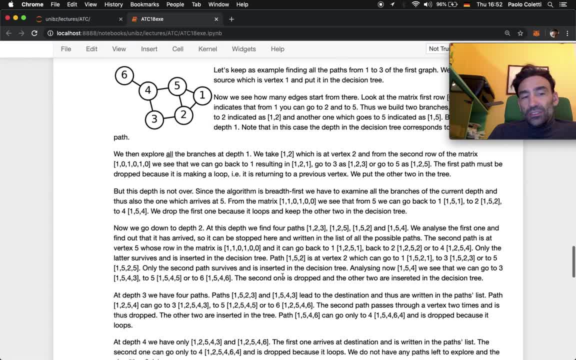 list, and this one is the only one open list, and this one is the only one open. from six you can go only to four. from six, you can go only to four. from six, you can go only to four. and so one, two, five, four, six, four. and so one, two, five, four, six, four. 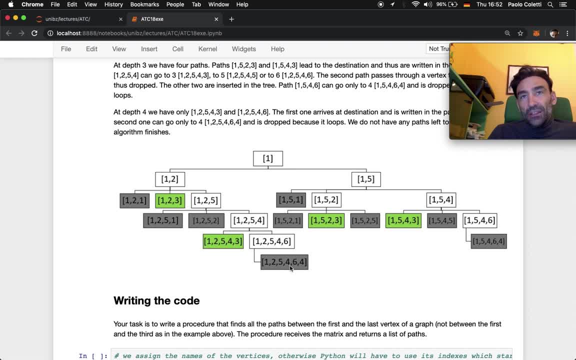 and so one, two, five, four, six, four, but we go to a place in which you have, but we go to a place in which you have, but we go to a place in which you have already been, already been, already been, and so goodbye, this one is cancelled. now we have no. 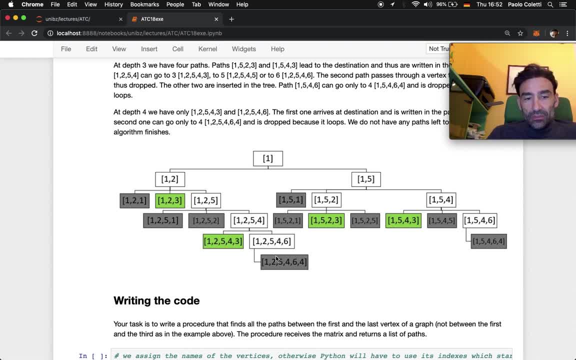 goodbye, this one is cancelled. now we have no. goodbye, this one is cancelled. now we have no branch open and the algorithm stops. branch open and the algorithm stops. branch open and the algorithm stops. okay, pay attention that, while the okay pay attention that, while the okay pay attention that, while the branch and bound and the other the. 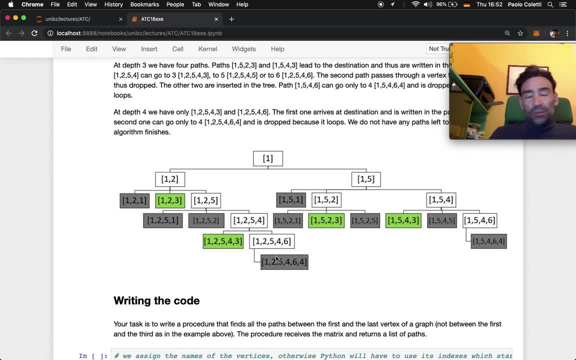 branch and bound and the other the branch and bound and the other the backtracking. stop as soon as they find backtracking. stop as soon as they find backtracking. stop as soon as they find one solution or the best solution. this one solution or the best solution, this. 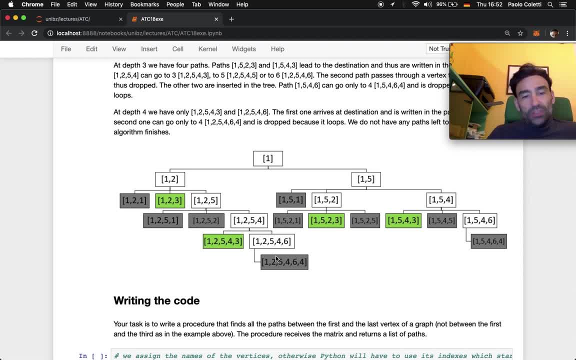 one solution or the best solution. this one must stop when it doesn't have one must stop when it doesn't have. one must stop when it doesn't have anything to do anymore. because it must anything to do anymore, because it must anything to do anymore, because it must find all the solutions. 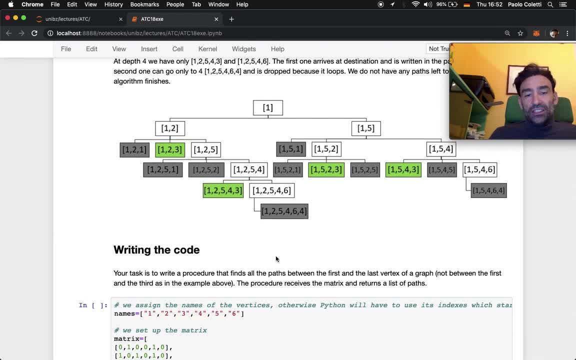 find all the solutions. find all the solutions, okay. if it is not clear for you, i suggest okay. if it is not clear for you, i suggest okay. if it is not clear for you, i suggest you, to you, to you, to listen it, listen to it again. let's go on. 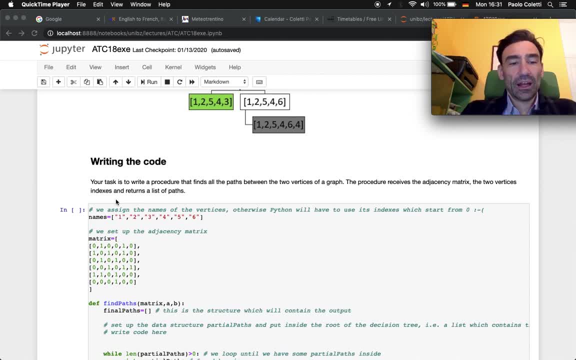 listen it. listen to it again. let's go on. listen it. listen to it again. let's go on. now it's your task to write the code. now it's your task to write the code. now it's your task to write the code. okay, i ask you to write a code which: 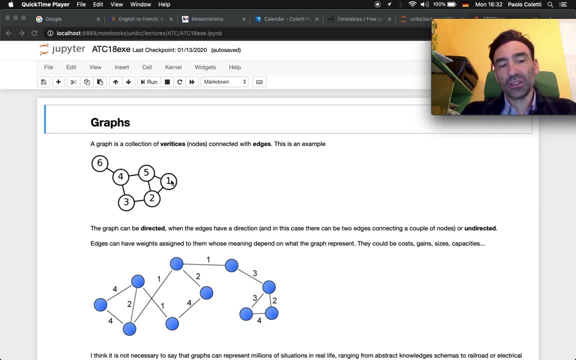 okay, i ask you to write a code which. okay, i ask you to write a code which finds all the path between finds, all the path between finds, all the path between a node and another one. so just two a node and another one. so just two a node and another one. so just two generic node which will be specified. 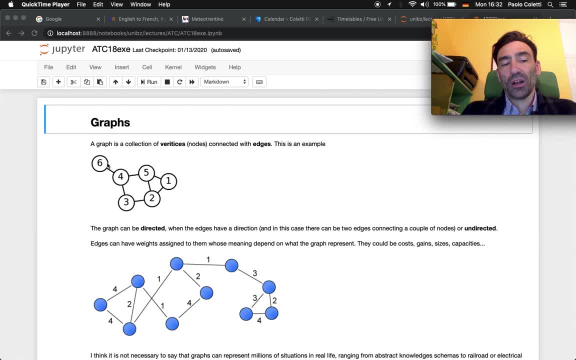 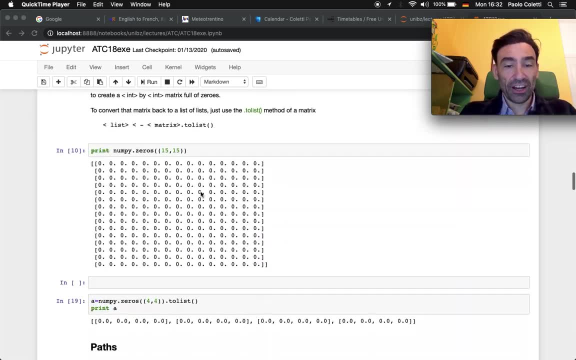 generic node, which will be specified. generic node, which will be specified the code. so you specify two nodes. the code. so you specify two nodes. the code. so you specify two nodes. the code will have to find all the path. the code will have to find all the path. 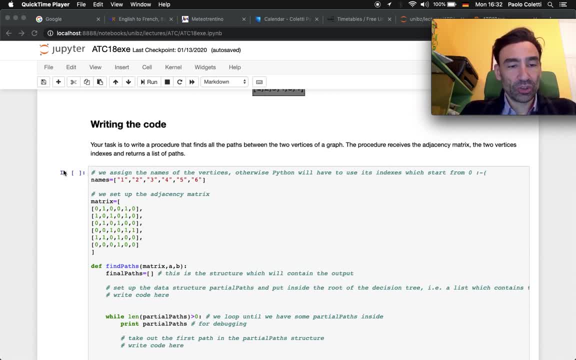 the code will have to find all the path here, here, here, i, as usual, i gave you some indications. i, as usual, i gave you some indications. i, as usual, i gave you some indications here, here, here, first of all, if you don't mind, oh, i've first of all. if you don't mind, oh, i've. 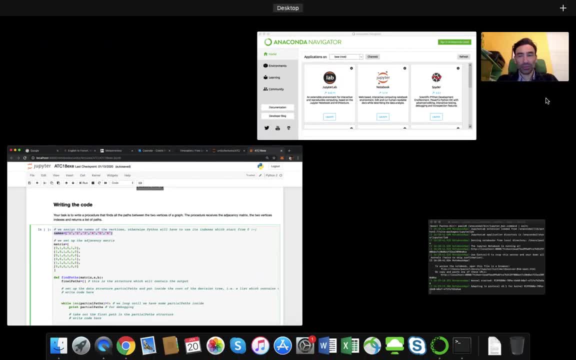 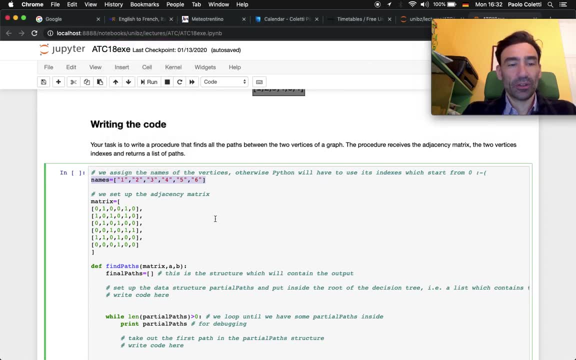 first of all, if you don't mind, oh, i've disappeared, disappeared, disappeared, i disappear. my face float on top, float on top. float on top. okay, oh, now i stay okay. okay, oh, now i stay okay, okay, oh, now i stay okay. first of all, if you don't mind, i set 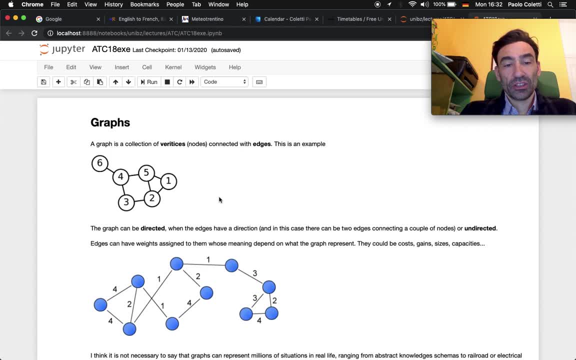 first of all, if you don't mind, i set first of all, if you don't mind, i set here the names, here the names, here the names, because python will use zero one, because python will use zero one, because python will use zero one, two, three, four, five. so, if you don't set, two, three, four, five. so if you don't set two, three, four, five, so if you don't set, i write here the names because at the i write here the names, because at the i write here the names, because at the end i want you, end i want you. 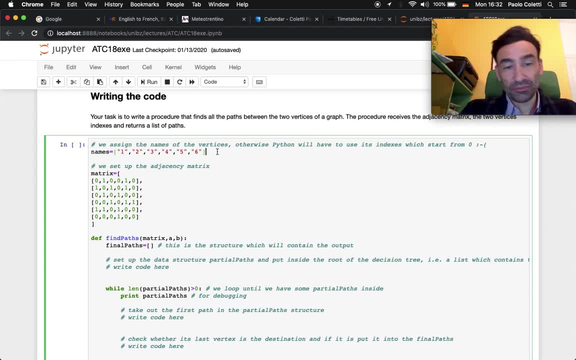 end. i want you to use the english names, not the. to use the english names, not the. to use the english names, not the pythonic names. first of all pythonic names, first of all pythonic names. first of all. second thing, because these names now are. second thing, because these names now are. 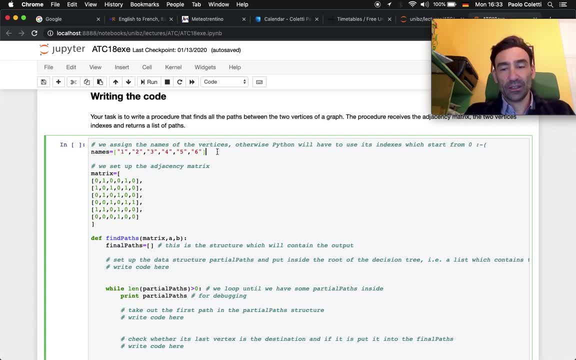 second thing, because these names now are one, two, three, four, five, six, but they may one, two, three, four, five, six. but they may one, two, three, four, five, six, but they may be towns, be towns, be towns. uh stages of your production level letters. uh, stages of your production level letters. 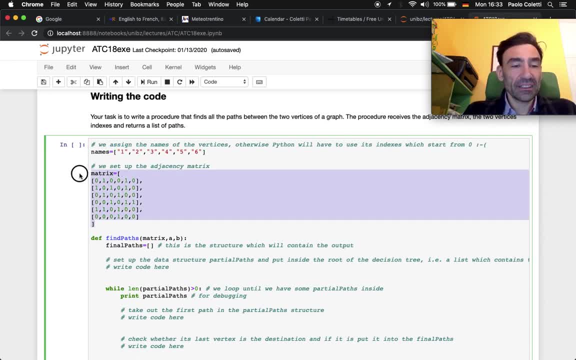 uh, stages of your production level, letters, whatever, whatever, whatever. okay, the adjacent symmetrics. i have, okay, the adjacent symmetrics. i have. okay, the adjacent symmetrics. i have kindly written it for you as you can see, kindly written it for you, as you can see, kindly written it for you, as you can see, zeros on the diagonal because there is. 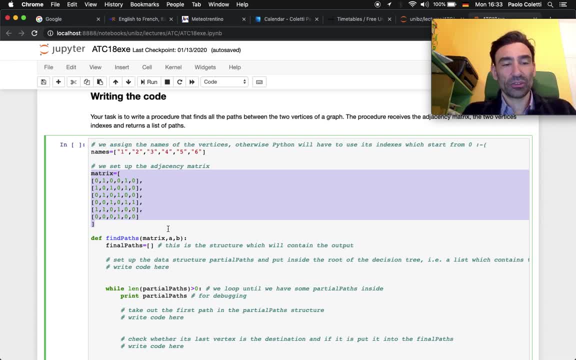 zeros on the diagonal, because there is zeros on the diagonal, because there is no, no, no, uh, no vertex which returns to itself. uh, no vertex which returns to itself. uh, no vertex which returns to itself. and the symmetric and the symmetric and the symmetric. okay, then, your task. 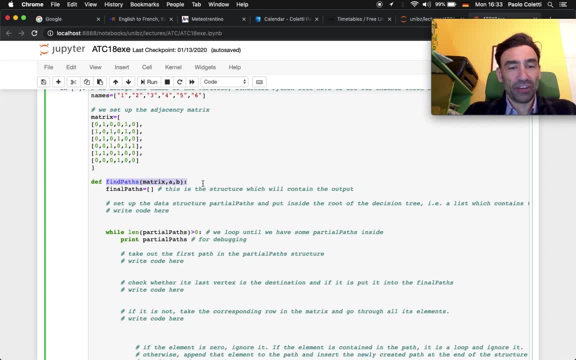 okay, then your task. okay, then your task: find path. so you are required to build find path. so you are required to build find path. so you are required to build the procedure find path, the procedure find path. the procedure find path receives as input edges and symmetrics. 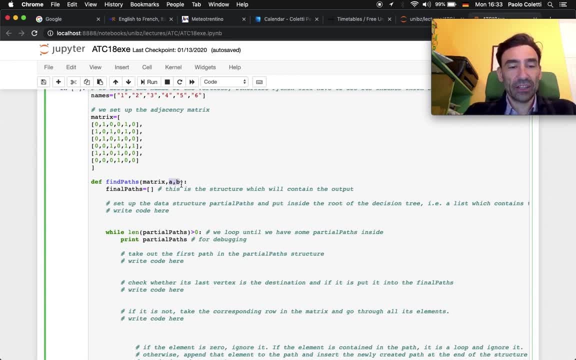 receives as input: edges and symmetrics. receives as input: edges and symmetrics. and the starting and ending vertex, so. and the starting and ending vertex, so. and the starting and ending vertex, so: the source, the source, the source and the destination. okay, so a is the and the destination. okay, so a is the. 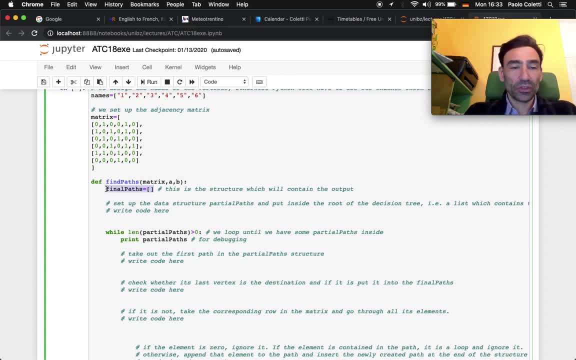 and the destination. okay, so a is the source, b is the destination, source b is the destination, source, b is the destination. okay, as usual, we use a data structure. okay, as usual, we use a data structure. okay, as usual, we use a data structure, which is a list. for the moment, it will. 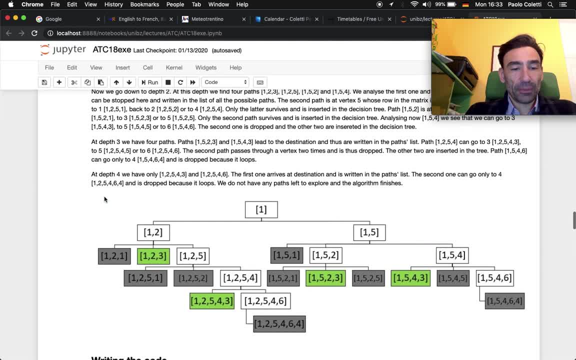 which is a list for the moment. it will, which is a list for the moment. it will be empty, be empty, be empty. it's a list of all the temporary paths. so it's a list of all the temporary paths. so it's a list of all the temporary paths. so, for example, you will store here one at. 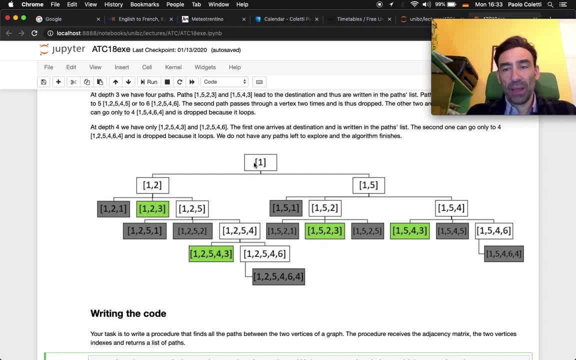 for example, you will store here one at. for example, you will store here one at the beginning, then you will pick one the beginning, then you will pick one the beginning, then you will pick one, expand it and store one, two, one, five. expand it and store one, two, one, five. 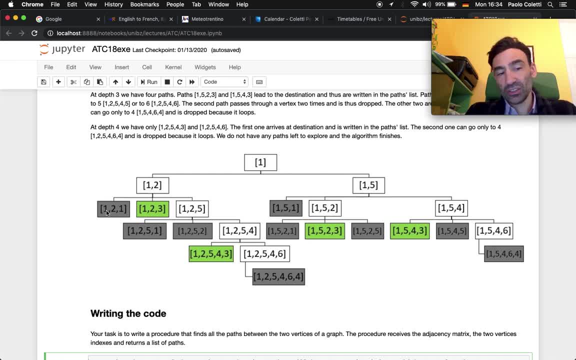 expand it and store one, two, one, five. then you will pick one, two, expand it. then you will pick one, two, expand it. then you will pick one, two, expand it and store well, not one, two, one which is. and store well, not one, two, one which is. and store well, not one, two, one which is forbidden, but one, two, three. one, two, five. 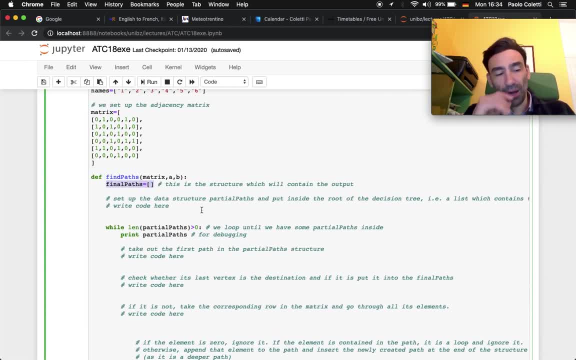 forbidden. but one, two, three, one, two, five forbidden. but one, two, three, one, two, five, et cetera, et cetera. so exactly like the, et cetera, et cetera. so exactly like the, et cetera, et cetera. so exactly like the branch and bound and backtracking. 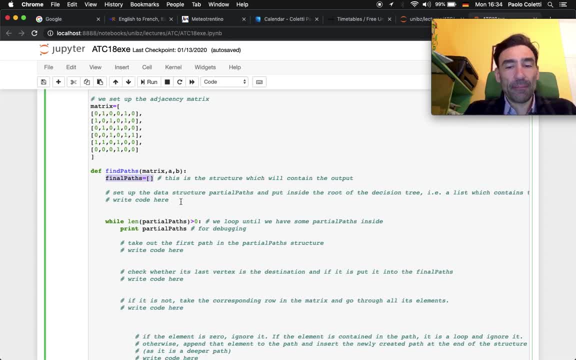 branch and bound and backtracking. branch and bound and backtracking structures- very similar structures, very similar structures, very similar. so starts empty. okay, i ask you to put inside the root of. okay, i ask you to put inside the root of. okay, i ask you to put inside the root of the decision three. 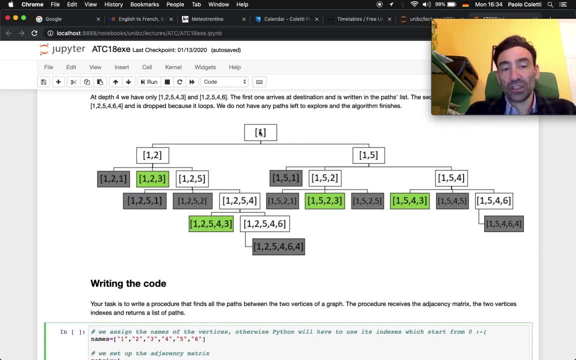 the decision three, the decision three. okay, so very simple, just this, so pay okay. so very simple, just this, so pay okay. so very simple, just this, so pay attention that here in the example one, attention that here in the example one, attention that here in the example one was the source. here the source is just a. 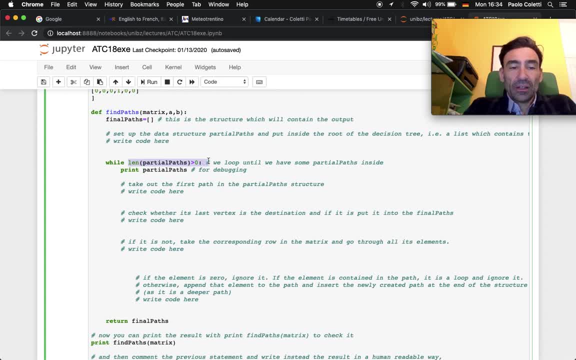 was the source? here, the source is just a. was the source here? the source is just a. okay, then you go on with the algorithm. okay, then you go on with the algorithm. okay, then you go on with the algorithm. remember that in this task, you have to remember that in this task, you have to. 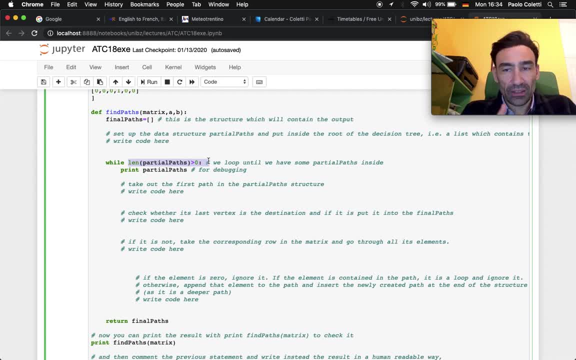 remember that in this task, you have to search for all the path, not for just one. search for all the path, not for just one. search for all the path, not for just one. not for the best, so you will go on until. not for the best, so you will go on until. 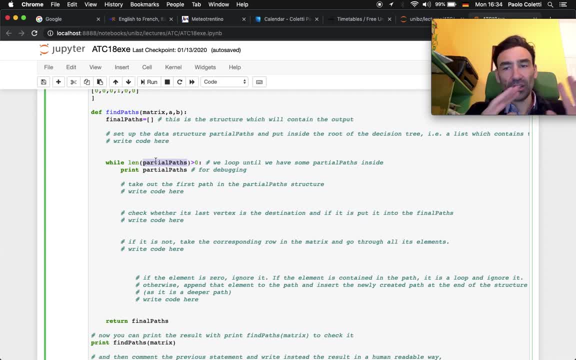 not for the best. so you will go on until you have partial paths which are open. so you have partial paths which are open, so you have partial paths which are open. so it will explore all the paths except the. it will explore all the paths except the. it will explore all the paths except the ones which are forbidden. clearly, 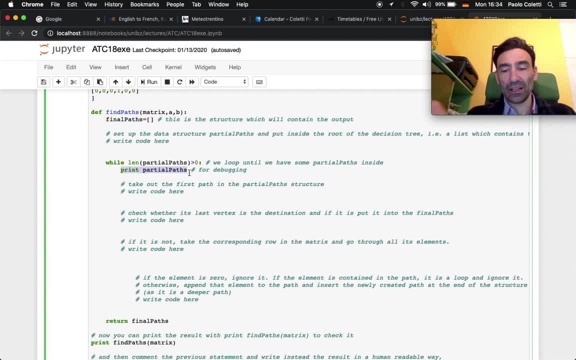 ones which are forbidden clearly. ones which are forbidden clearly. just for debugging purposes. i will print just for debugging purposes. i will print just for debugging purposes. i will print the list of the path currently in the, the list of the path currently in the. the list of the path currently in the variable. 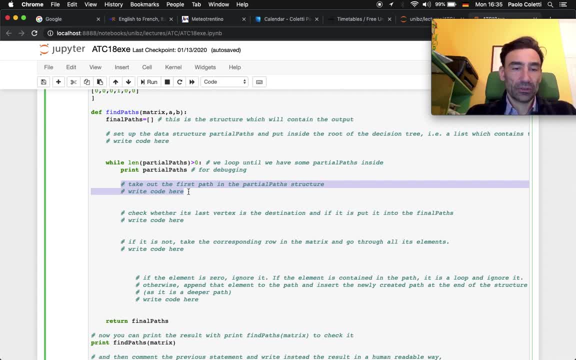 variable, variable. as usual. take out the first path. as usual. take out the first path as usual. take out the first path together with the structure, because the together with the structure, because the together with the structure, because the partial path will be kept. partial path will be kept. 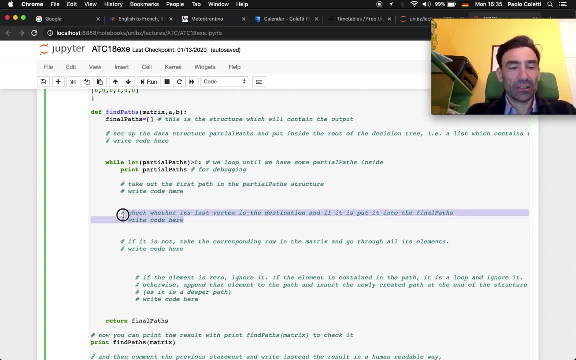 partial path will be kept in order. okay, you must check whether in order. okay, you must check whether in order. okay, you must check whether the last vertex of the path is a. the last vertex of the path is a. the last vertex of the path is a destination. 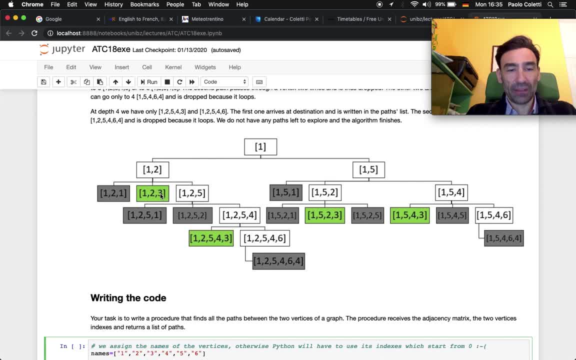 destination, destination. so whether this one, which is the last, so whether this one, which is the last, so whether this one, which is the last vertex of the path, vertex of the path, vertex of the path, is already our destination, it means that is already our destination. it means that 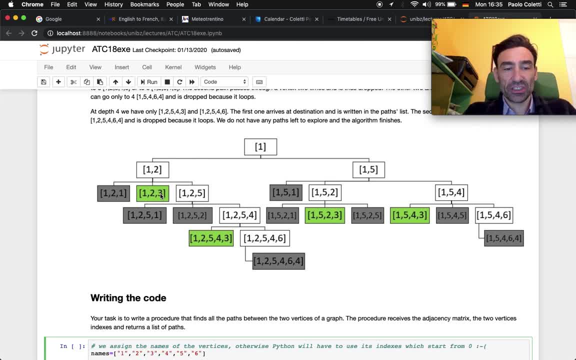 is already our destination. it means that you are analyzing, in this case, a path. you are analyzing, in this case, a path. you are analyzing, in this case, a path which has just reached its destination, which has just reached its destination, which has just reached its destination. in this case, this path will be put in a 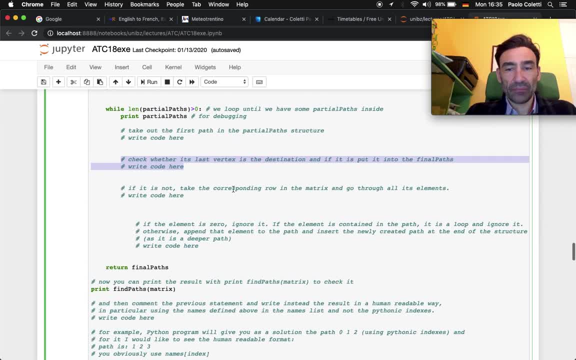 in this case, this path will be put in a. in this case, this path will be put in a list, list, list, which will be our output. okay, it will be, which will be our output. okay, it will be, which will be our output. okay, it will be put in a list called. 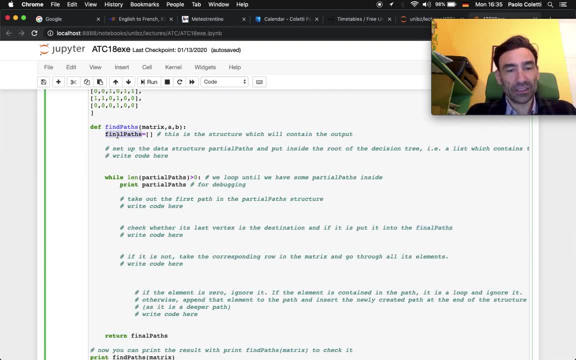 put in a list called. put in a list called final path which you have to set up. ah, final path which you have to set up, ah final path which you have to set up, ah, it's already set up here. it's already set up here. it's already set up here, no wait. 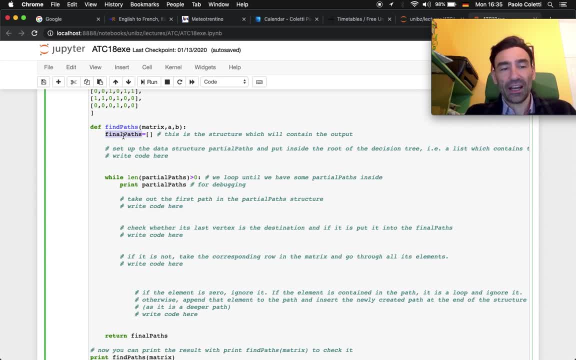 which will contain the output. okay, sorry, which will contain the output. okay, sorry, which will contain the output. okay, sorry. final path contains the output. and final path contains the output. and final path contains the output and partial paths which you have to set up. partial paths which you have to set up. 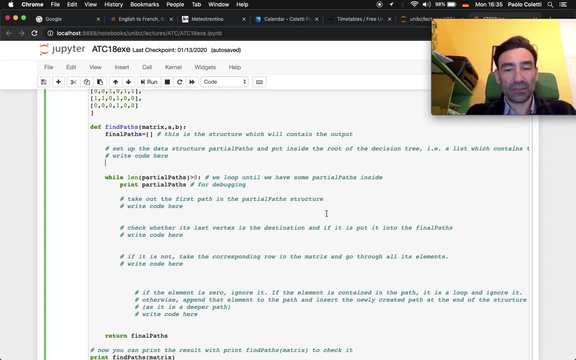 partial paths which you have to set up. here will contain all the open paths. so here will contain all the open paths. so here will contain all the open paths. so you put the path into the final path. you put the path into the final path. you put the path into the final path list. 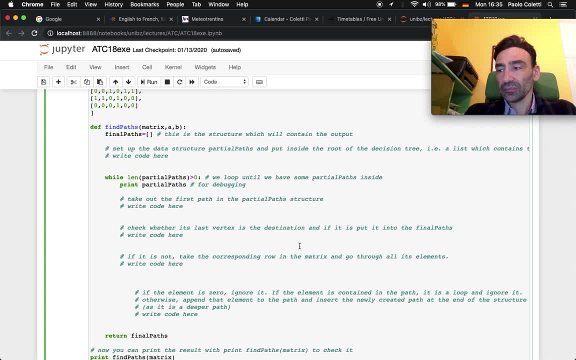 list: list. if it is not so. if the last. if it is not so. if the last. if it is not so. if the last element. if the last vertex of the path is element. if the last vertex of the path is element. if the last vertex of the path is not a destination. 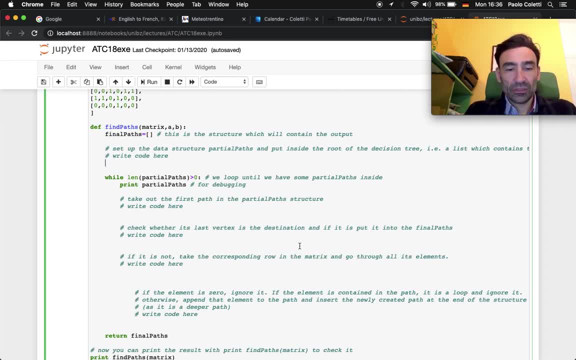 not a destination, not a destination, then what you have to do, you have to go, then what you have to do, you have to go, then what you have to do, you have to go on on, on. so you will have to take a look for. so you will have to take a look for. 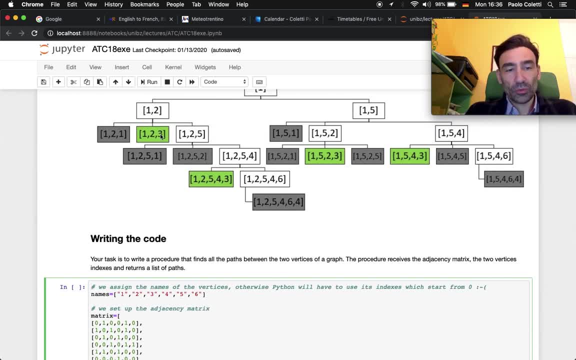 so you will have to take a look. for example, suppose you are here at two example. suppose you are here at two example, suppose you are here at two, which in pythonic is one, so this one. you, which in pythonic is one, so this one. you, which in pythonic is one, so this one, you have to take a look at the edges. 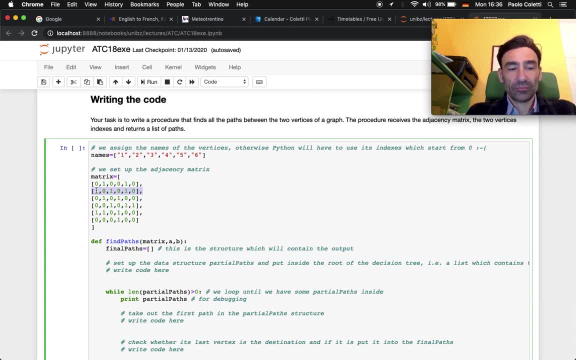 have to take a look at the edges, have to take a look at the edges- matrix row, matrix row, matrix row- and see where you can go, and see where you can go, and see where you can go. so you have to loop, so you have to loop, so you have to loop through these values here. 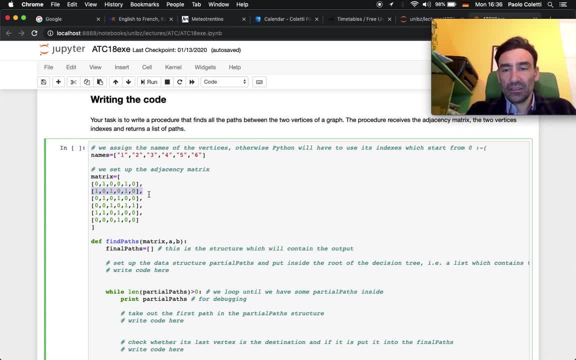 through these values here, through these values here, if you find that zero, it means that you, if you find that zero, it means that you, if you find that zero, it means that you can't go there, can't go there, can't go there, stop, stop, don't do anything. if you find a, 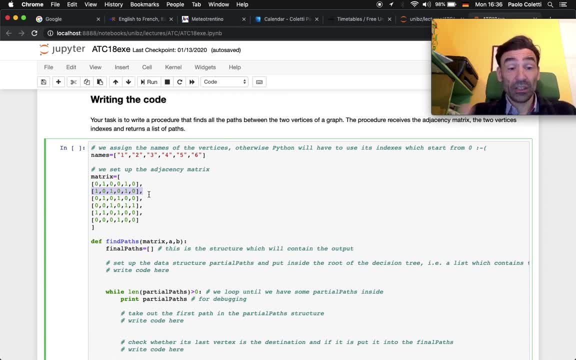 stop, stop, don't do anything if you find a stop, stop. don't do anything if you find a one, one one or in general, a value which is larger, or in general, a value which is larger, or, in general, a value which is larger than one because than one, because 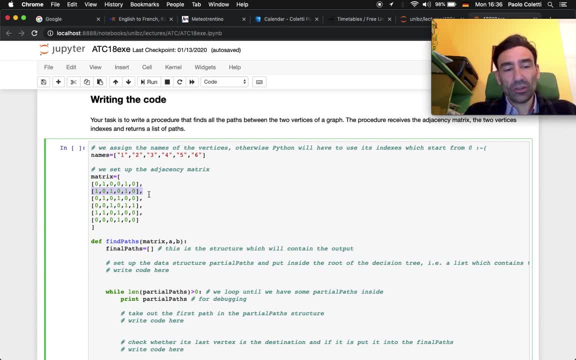 than one, because the the graph may be weighted. so if you, the the graph may be weighted. so if you, the the graph may be weighted. so if you find a one or a value which is larger, find a one or a value which is larger, find a one or a value which is larger than zero. anyway, 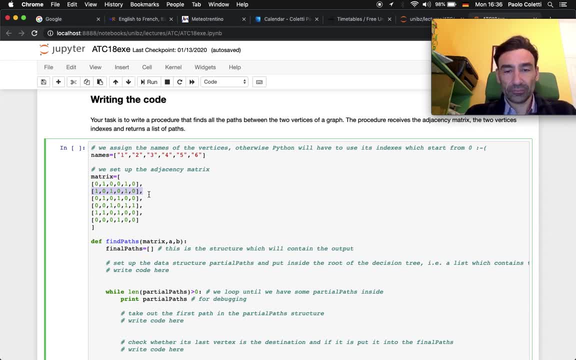 than zero, anyway, than zero, anyway. okay. in this case, it means that you can: okay. in this case, it means that you can okay. in this case, it means that you can go there, go there, go there. so you have to build the appropriate path, so you have to build the appropriate path. 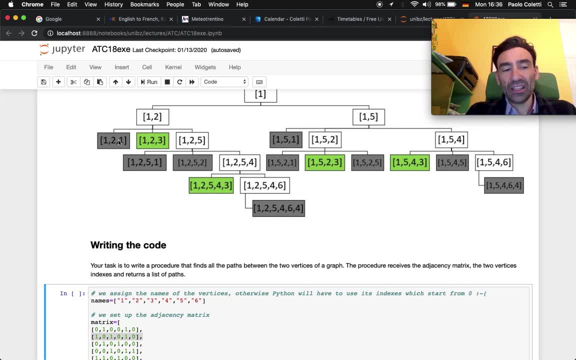 so you have to build the appropriate path now. where you are now is not contained now. where you are now is not contained now. where you are now is not contained in the rest of the path, in the rest of the path, in the rest of the path. because if the node where you are now is because if the node where you are now is because if the node where you are now is the vertex where you're now is the vertex where you're now is the vertex where you're now is containing the rest of the path, containing the rest of the path. 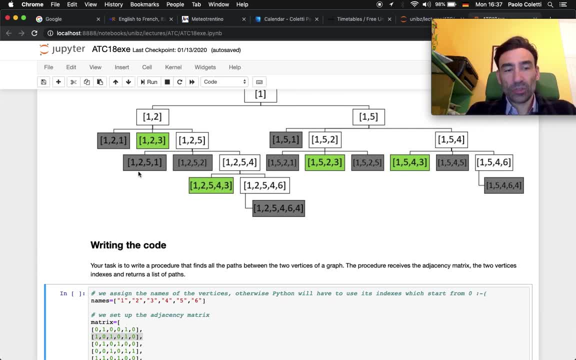 containing the rest of the path. this is not allowed, okay, this is not allowed, okay, this is not allowed, okay. so you have to go through, so you have to go through, so you have to go through the corresponding row of the agency's, the corresponding row of the agency's. 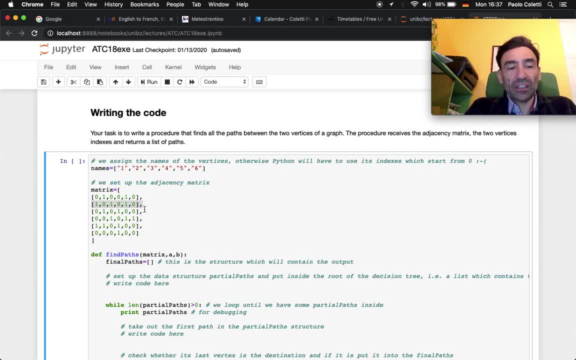 the corresponding row of the agency's matrix. if. if the value of. if. if the value of if. if the value of if the value is zero, skip that one. if the if the value is zero, skip that one. if the if the value is zero, skip that one if the value is not zero. okay. 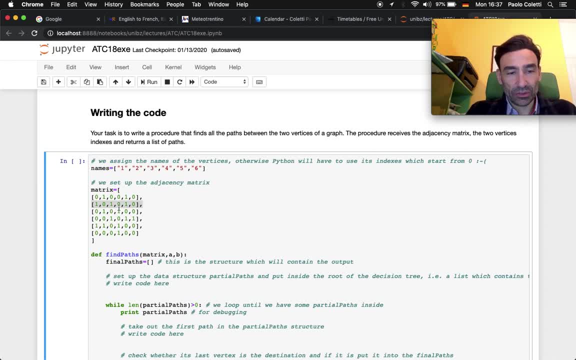 value is not zero. okay, value is not zero, okay, add that index so zero one, two, three. add that index so zero one, two, three. add that index so zero one, two, three, four, five, four, five, four, five to the path. but if that index is already to the path, but if that index is already. 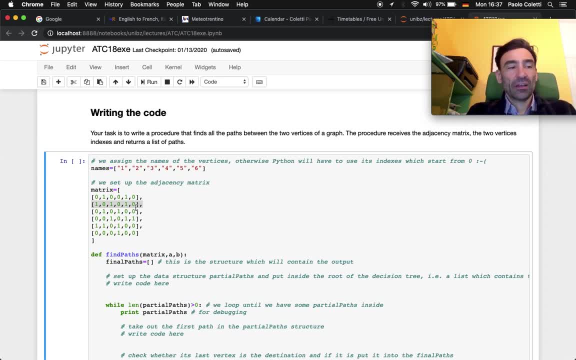 to the path, but if that index is already containing the path, containing the path, containing the path, ignore this path. so only if the ignore this path, so only if the ignore this path. so only if the corresponding value is not zero, corresponding value is not zero, corresponding value is not zero. and if that index is not already. 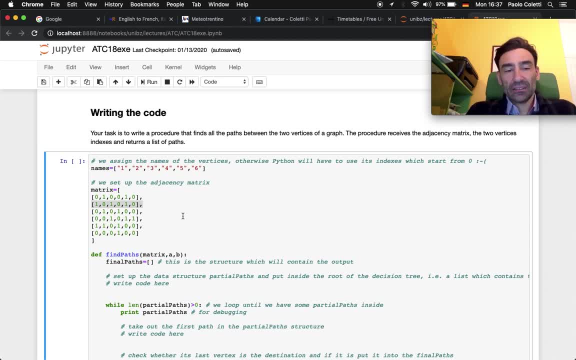 and if that index is not already, and if that index is not already containing the path, in that case containing the path. in that case containing the path. in that case, you add this partial path to the partial. you add this partial path to the partial. you add this partial path to the partial path list. 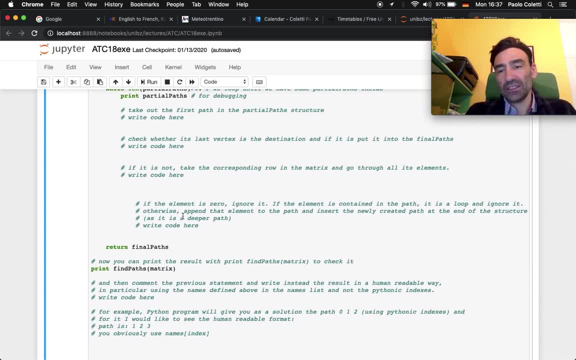 path list: path list: that's it. finish it will go alone. that's it finish. it will go alone. that's it finish. it will go alone itself, exactly like the other ones, itself, exactly like the other ones, itself, exactly like the other ones continue extracting, putting the results. 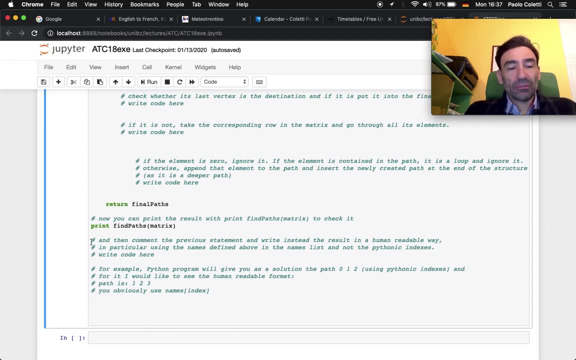 continue extracting, putting the results, continue extracting, putting the results away, away, away. okay, but it's not over. okay, but it's not over. okay, but it's not over. i ask you to write down the result in a. i ask you to write down the result in a. 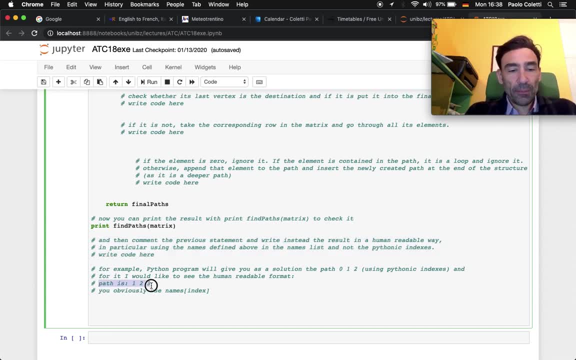 i ask you to write down the result in a human readable way. human readable way, human readable way. okay, for example, path is one, two, three. okay, for example, path is one, two, three. okay. for example, path is one, two, three. then below, path is one, two, five, four. 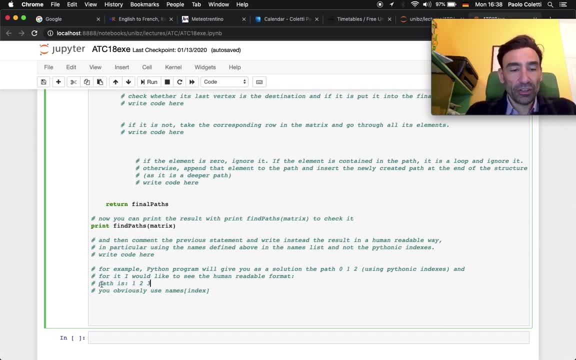 then below path is one, two, five, four. then below path is one, two, five, four, three. okay, so in this way. so first of three. okay, so in this way. so first of three. okay, so in this way. so first of all, all, all with the list of the path, one after the. 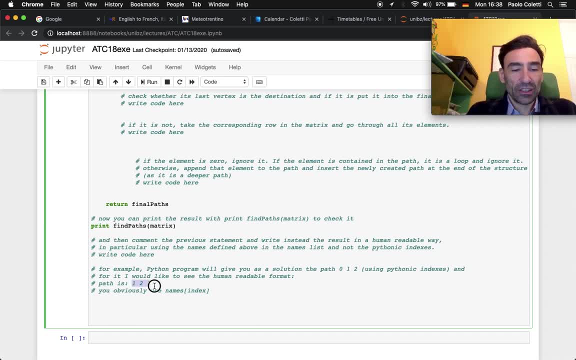 with the list of the path, one after the, with the list of the path one after the other, and not a mess other, and not a mess other and not a mess, and then using your english names, and, and then using your english names, and, and then using your english names and not pythonic names. 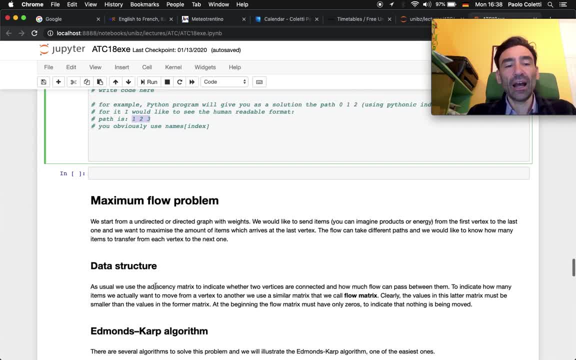 not pythonic names, not pythonic names. okay, these are your tasks. and now, okay, these are your tasks. and now, okay, these are your tasks. and now we go to a new topic, which is the maximum flow problem there, which is the maximum flow problem there, which is the maximum flow problem. there are tons and tons and tons of. 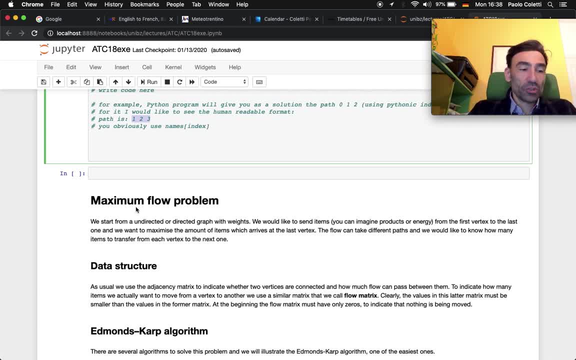 are tons and tons and tons of are tons and tons and tons of problems which can be. we start from here. problems which can be we start from here. problems which can be we start from here. which use find all the path in a. which use find all the path in a. 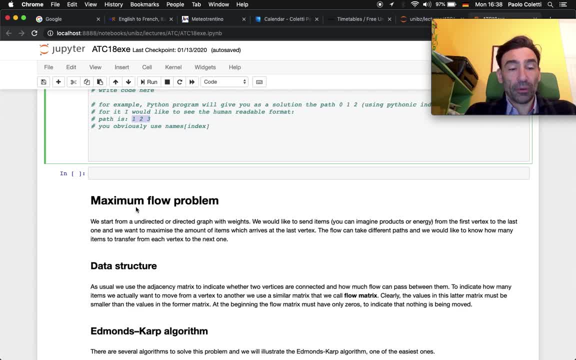 which use find all the path in a graph. one of them is the maximum flow graph. one of them is the maximum flow graph. one of them is the maximum flow problem. problem, problem. we start from a graph like this one for. we start from a graph like this one for. 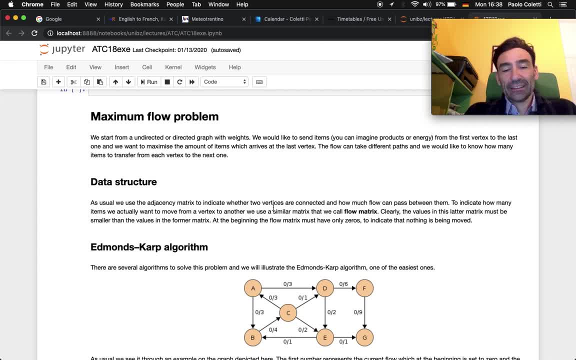 we start from a graph like this one, for example, example, example, which is a directed graph, which is a directed graph, which is a directed graph with weights. okay, you can imagine this with weights. okay, you can imagine this with weights. okay, you can imagine this one, for example, as a supply chain. 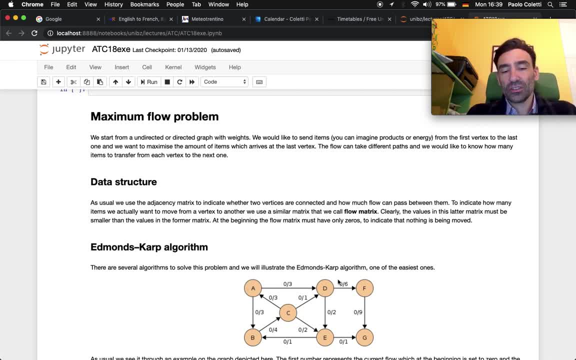 one, for example, as a supply chain. one, for example, as a supply chain or as a logistics system. you have several. or as a logistics system, you have several, or as a logistics system. you have several. towns, towns, towns. in each town, you have a driver with a van. 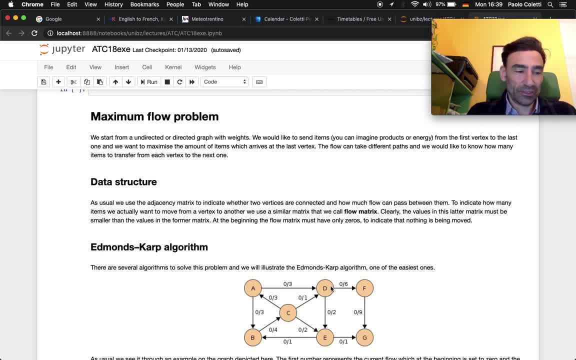 in each town you have a driver with a van. in each town, you have a driver with a van. okay, the driver with a van can carry. okay, the driver with a van can carry. okay, the driver with a van can carry only one item. well, okay, you can imagine. 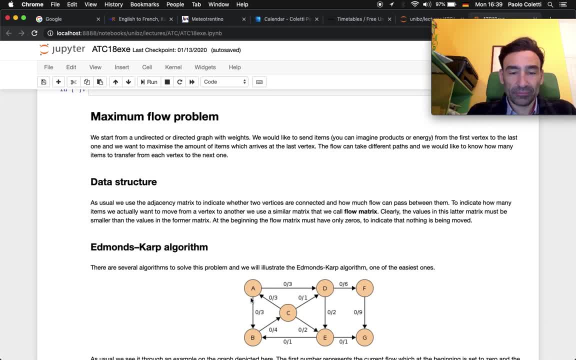 only one item. well, okay, you can imagine only one item. well, okay, you can imagine one big box of items, not one item. one big box of items, not one item. one big box of items, not one item. okay, for example, in this case you have. okay, for example, in this case you have. 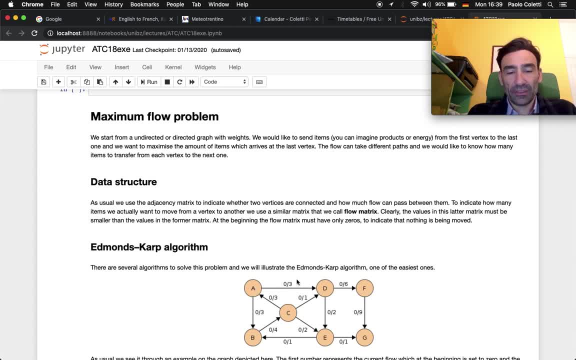 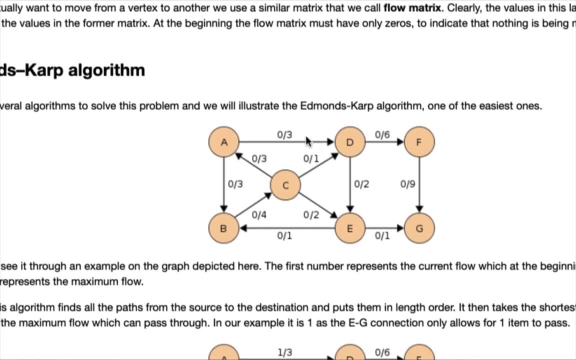 okay, for example, in this case you have, from from a to d: three available three. from from a to d: three available three. from from a to d: three available three. this number here: three available drivers. this number here: three available drivers. this number here: three available drivers carrying. 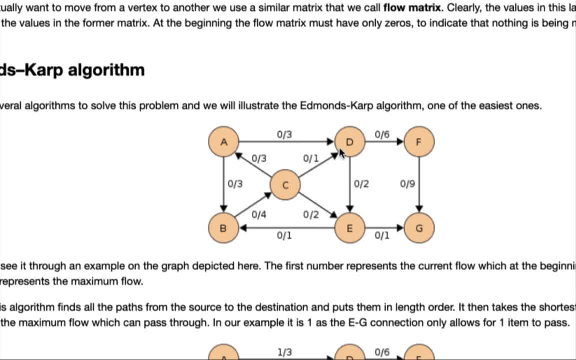 carrying carrying. which are able to carry one item once a which are able to carry one item once a. which are able to carry one item. once a driver arrives in d, he doesn't go back. driver arrives in d, he doesn't go back. driver arrives in d, he doesn't go back. well, it will go, but he will go back in. 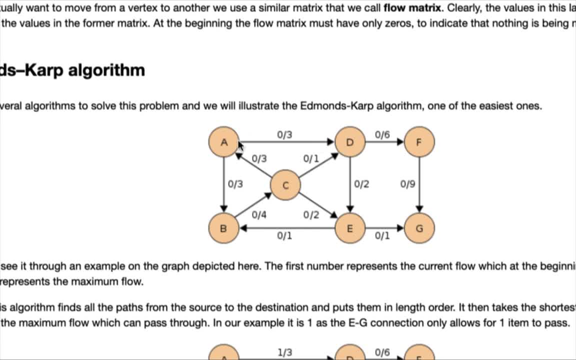 well, it will go, but he will go back in. well, it will go, but he will go back in the next day, the next day, the next day, but you can't use it anymore. okay so, but you can't use it anymore. okay so, but you can't use it anymore. okay, so, other three which go to b, so six. 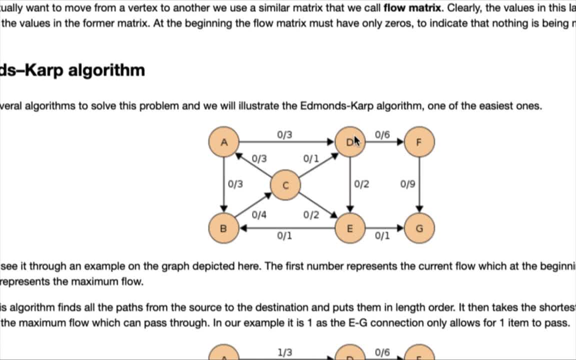 other three which go to b, so six other three which go to b, so six drivers in a, three which are ready to go, drivers in a, three which are ready to go, drivers in a three which are ready to go to b and three which are ready to go to. 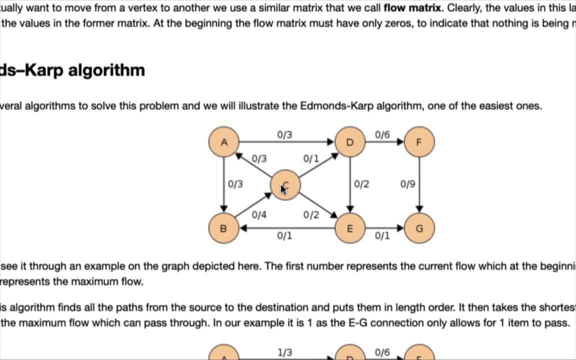 to b and three which are ready to go to to b and three which are ready to go to d. no one is ready to go to c on the d. no one is ready to go to c on the d. no one is ready to go to c. on the other hand, in c you have three drivers. 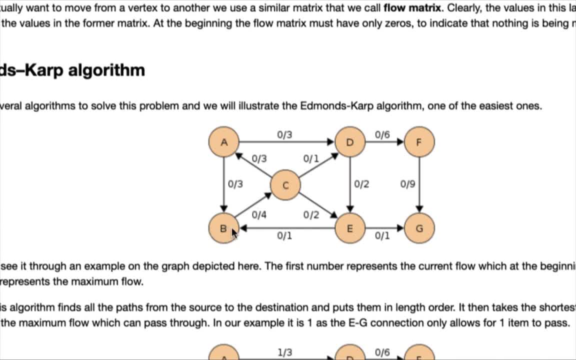 other hand, in c you have three drivers. other hand in c, you have three drivers ready to go back to a, ready to go back to a, ready to go back to a. four drivers in b ready to go to c. four drivers in b ready to go to c. 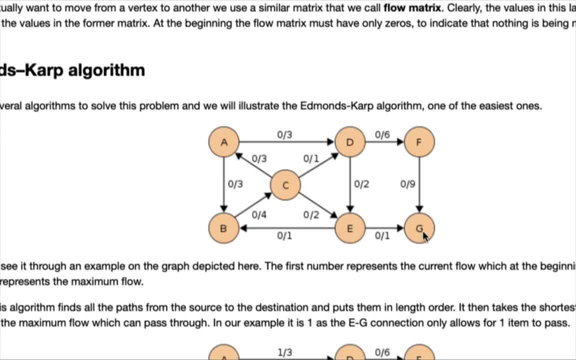 four drivers in b ready to go to c, one driver in e ready to go to b and one driver in e ready to go to b and one driver in e ready to go to b and another driver ready to go to g. another driver ready to go to g. 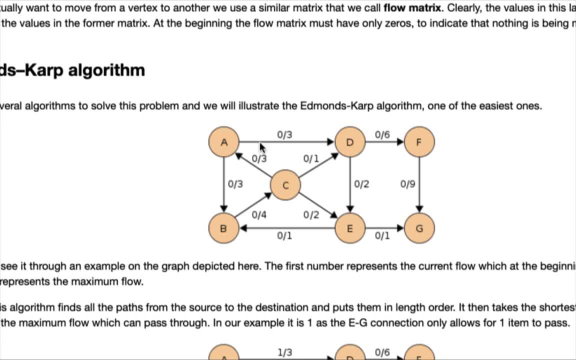 another driver ready to go to g, and that's your structure, and that's your structure, and that's your structure now you have a lot of items in a and you now you have a lot of items in a and you, now you have a lot of items in a and you have to send as much as possible. 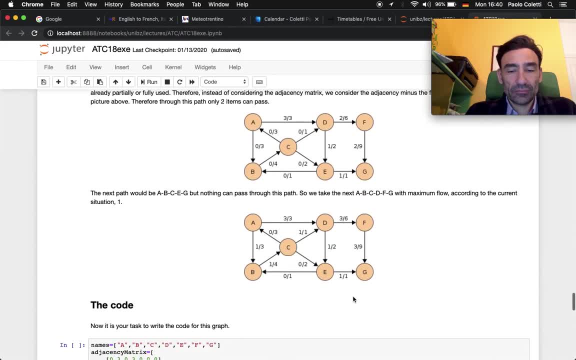 have to send as much as possible. have to send as much as possible through g. let me see whether the task is yeah. let me see whether the task is yeah. let me see whether the task is yeah. yes, so you have a lot of drivers in a. yes, so you have a lot of drivers in a. 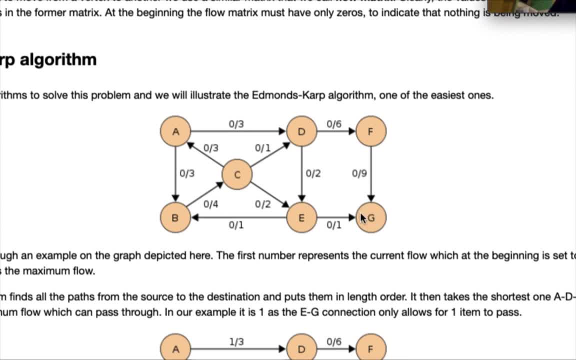 yes, so you have a lot of drivers in a and you have to send as much as possible, and you have to send as much as possible and you have to send as much as possible in g, in g, in g, okay, well, okay, well, okay, well, how? what is the algorithm to solve this? 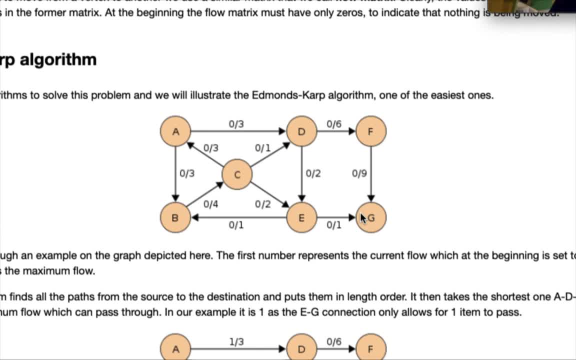 how? what is the algorithm to solve this? how? what is the algorithm to solve this problem? you can. you can use several paths. problem you can. you can use several paths. problem you can. you can use several paths. so you'll probably send some through. so you'll probably send some through. 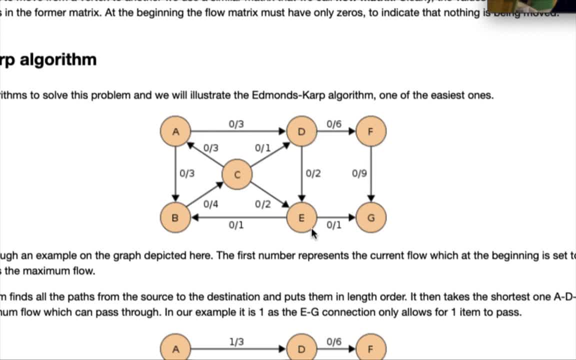 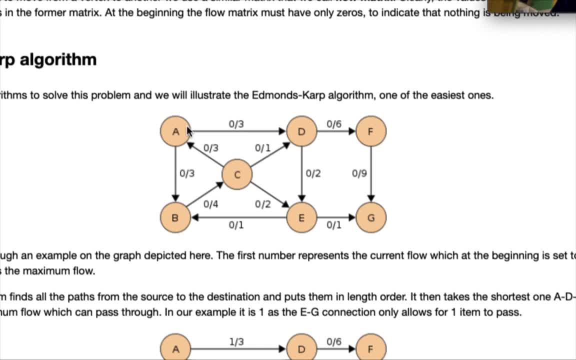 some to this path here, probably some to this path here, some to this path here, some to this path here, some some some tak tak, tak, tak. no, because once they're in b, tak tak, tak. no. because once they're in b, tak tak, tak. no, because once they're in b, tak tak, tak, no. 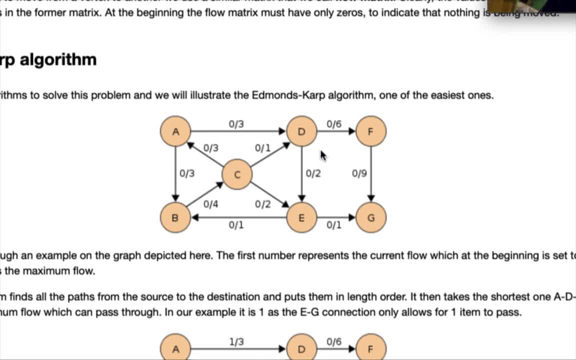 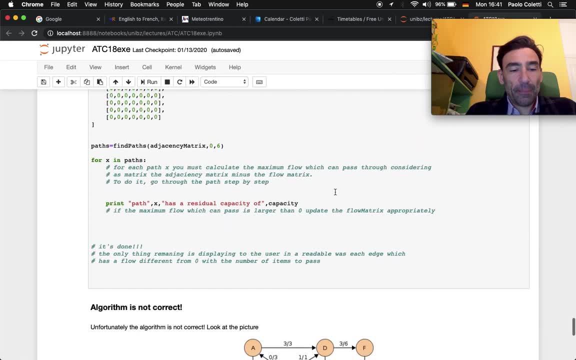 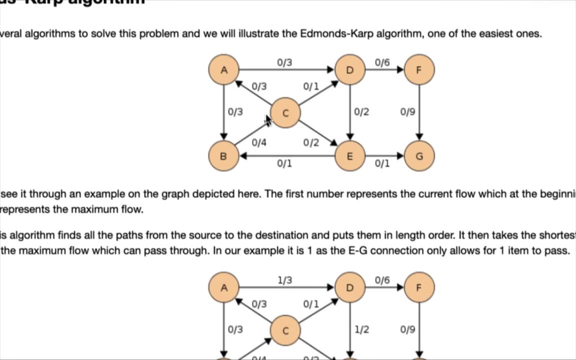 tak, tak, tak, no, tak, tak, tak. no, let's eat the algorithm. it's the edmunds carp algorithm. it's one. it's the edmunds carp algorithm. it's one. it's the edmunds carp algorithm. it's one of the easiest one to solve this problem. 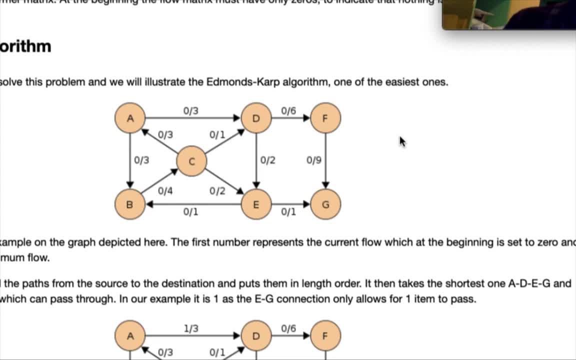 of the easiest one to solve this problem, of the easiest one to solve this problem, okay, first of all, first task. you have to. okay, first of all, first task. you have to. okay, first of all, first task: you have to find, find, find all the paths which lead from a 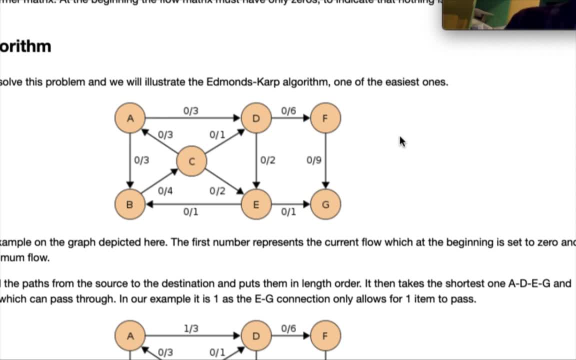 all the paths which lead from a, all the paths which lead from a to g, all of them to g, all of them to g, all of them second sort. the path in order of second sort. the path in order of second sort. the path in order of length. well, the algorithm that we have, 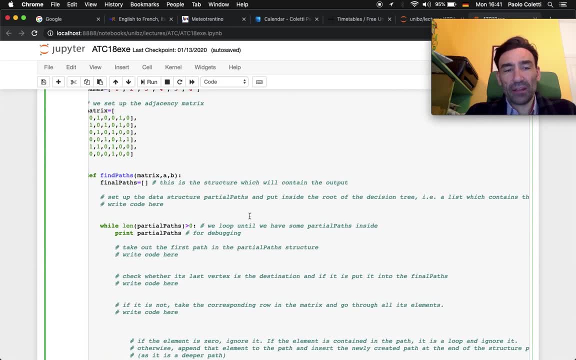 length. well, the algorithm that we have, length, well, the algorithm that we have seen here, this one automatically will seen here. this one automatically will seen here. this one automatically will give you the path in order of length. give you the path in order of length. give you the path in order of length because it's a breath first. so 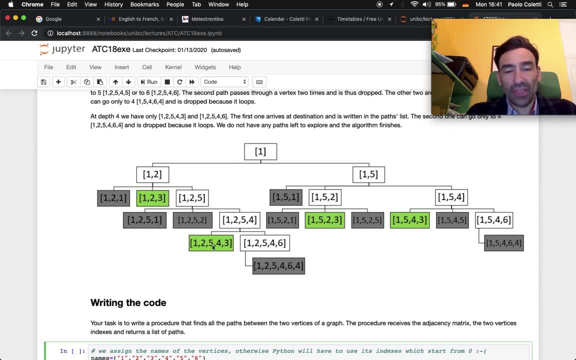 because it's a breath first, so because it's a breath first. so first it will give you this one, then this. first it will give you this one, then this. first it will give you this one, then this one and this one, and then this one. so one and this one and then this one. so 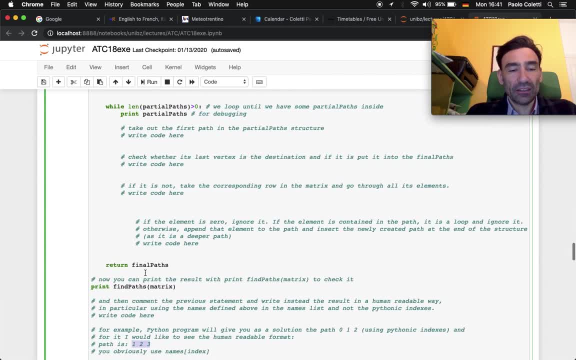 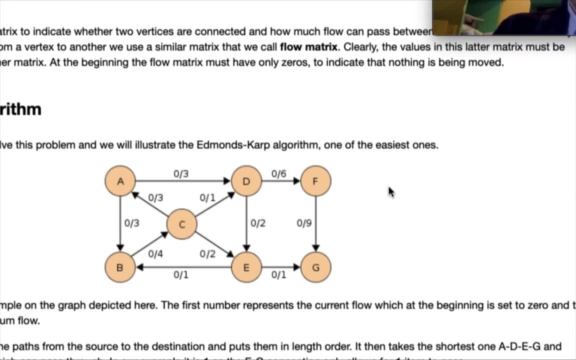 one and this one and then this one. so the path that you have here as output, the path that you have here as output, the path that you have here as output in final path, are already in length order in final path, are already in length order in final path, are already in length order. so fine, then take the first path. 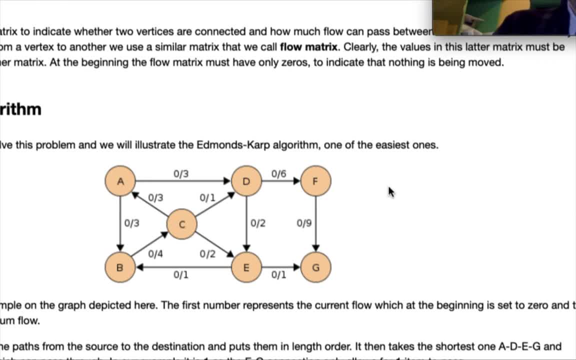 so fine, then take the first path. so fine, then take the first path and try to send through as much. and try to send through as much and try to send through as much items as possible. so a to d, d to f, items as possible. so a to d, d to f. 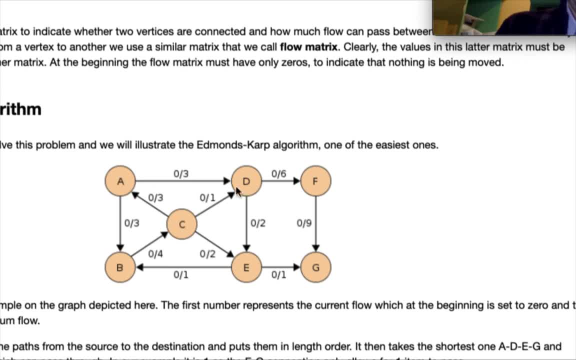 items as possible. so a to d, d to f, f to g and all sorry f to g and all sorry f to g and all sorry. here we take as first path a to d, d to e. here we take as first path a to d, d to e. 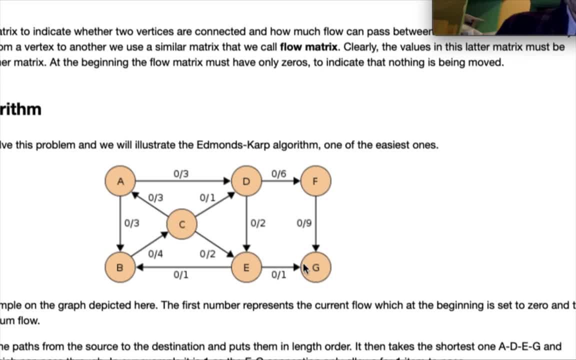 here we take as first path a to d, d to e and e to g. how many. what is the maximum? and e to g: how many? what is the maximum? and e to g: how many? what is the maximum number of items which you can send? number of items which you can send. 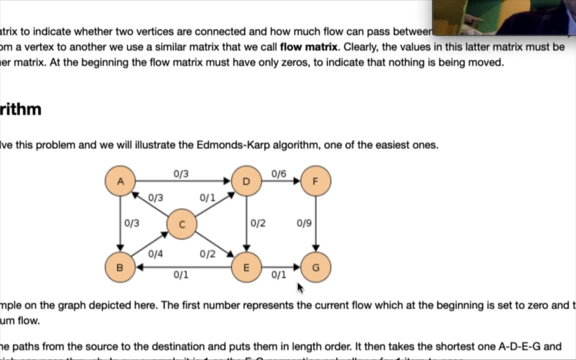 number of items which you can send through this path. through this path, only one, because e to g is limited to only one, because e to g is limited to only one, because e to g is limited to one one one. okay, at this point you must. okay, at this point, you must. 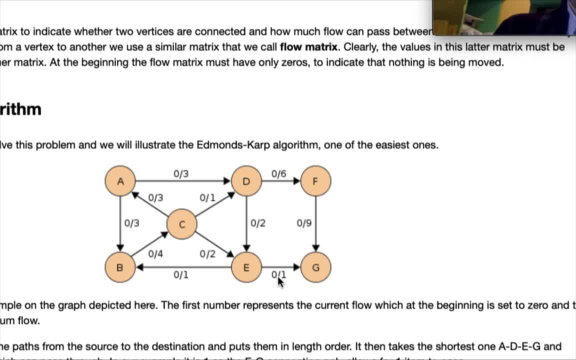 okay, at this point you must keep this, write this information, keep this, write this information, keep this, write this information somewhere, somewhere, somewhere, so you will have the usual adjacency, so you will have the usual adjacency, so you will have the usual adjacency, matrix which will tell you, matrix which will tell you. 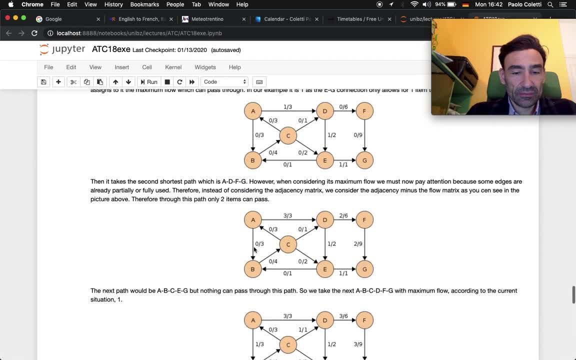 matrix which will tell you three, six, one, three. here it is three, six one. three here it is three, six one, three. here it is the usual adjacency matrix, the usual adjacency matrix, the usual adjacency matrix. it tells you how many items you can. it tells you how many items you can. 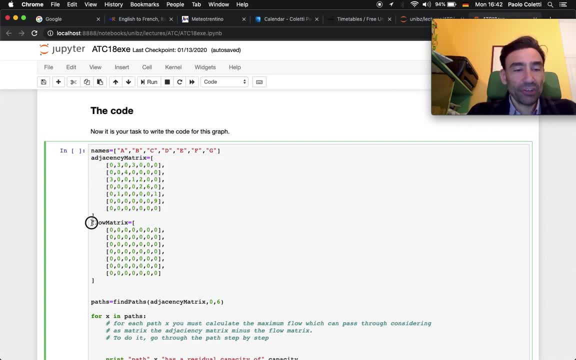 it tells you how many items you can send from a no from a vertex to another. send from a no from a vertex to another. send from a no from a vertex to another one. and the flow matrix. the flow matrix one. and the flow matrix- the flow matrix. 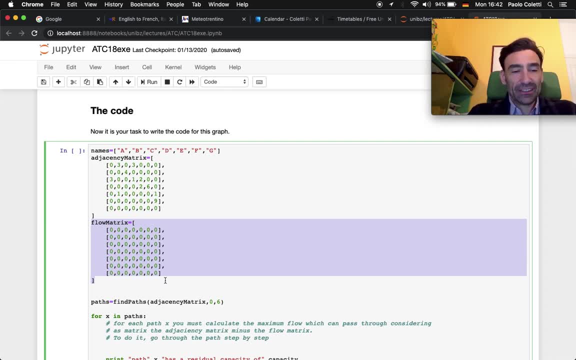 one and the flow matrix. the flow matrix tells you, tells you, tells you how many items are you actually sending, how many items are you actually sending? how many items are you actually sending at the beginning? clearly it's zero at the beginning. clearly it's zero at the beginning. clearly it's zero. okay, so you update your flow matrix. 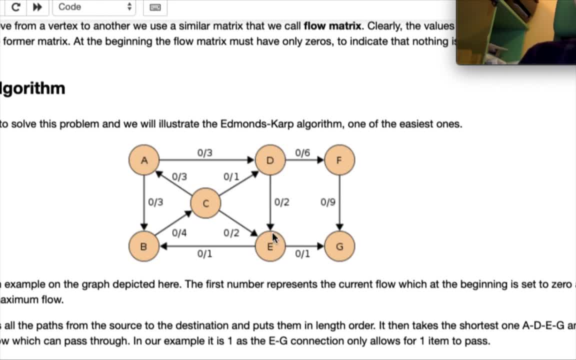 okay, so you update your flow matrix. okay, so you update your flow matrix indicating that from a to d you send one. indicating that from a to d you send one. indicating that from a to d you send one item, from d to e one item and from d to 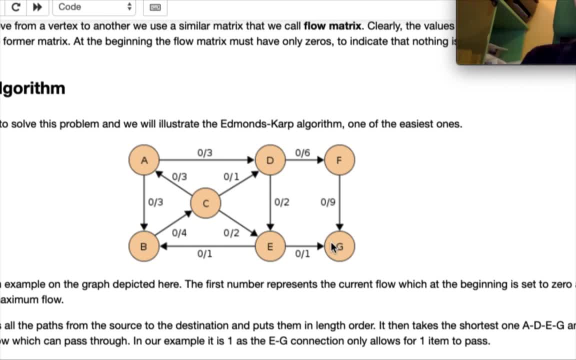 item. from d to e: one item. and from d to item: from d to e: one item. and from d to e to g: one item. e to g: one item. e to g: one item. okay, so you will have some ones in the. okay, so you will have some ones in the. 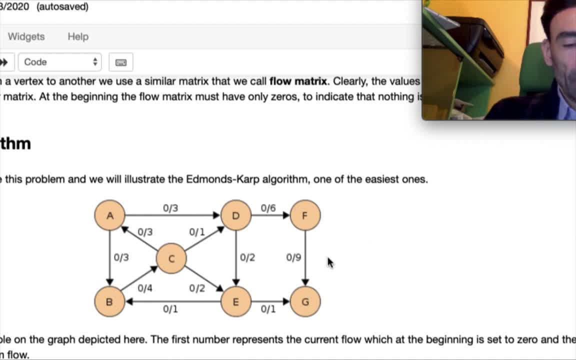 okay, so you will have some ones in the flow matrix, flow matrix, flow matrix. now second step: take the second longest. now second step. take the second longest. now second step. take the second longest. path in this case is at the same length. path, in this case is at the same length. 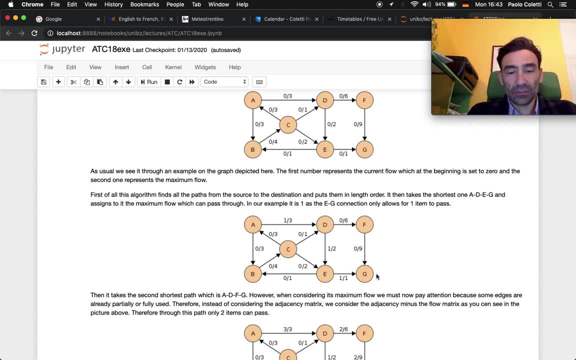 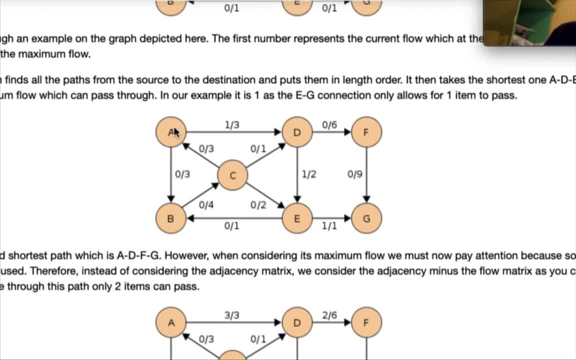 okay, the second longest path is a to d. okay, the second longest path is a to d, d to f and f to g, d to f and f to g, d to f and f to g. so how many items can we ship here? well? so how many items can we ship here, well? 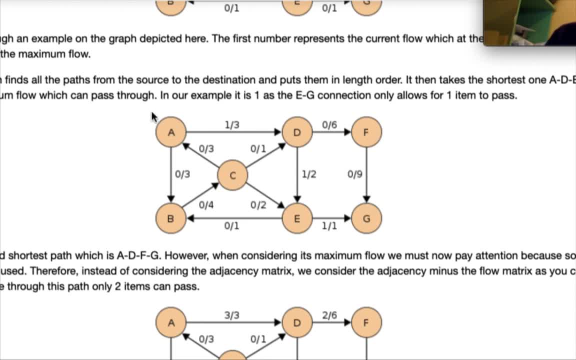 so how many items can we ship here? well, usually three, because three here six, and usually three, because three here six, and usually three because three here six and here nine, so usually three. however, one here nine, so usually three. however, one here nine, so usually three. however, one of the driver here, drivers here- is 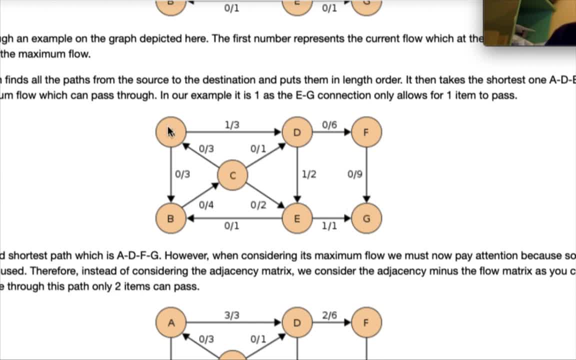 of the driver here. drivers here is of the driver here. drivers here is already busy, already busy, already busy shipping things here, shipping things here, shipping things here, so, so, so, unfortunately only two, so whenever you, unfortunately only two, so whenever you. unfortunately only two, so whenever you consider how many items you can send. 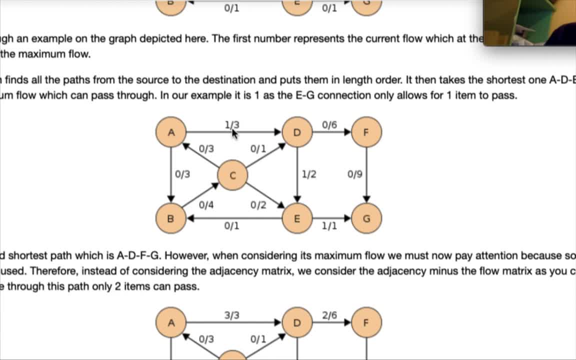 consider how many items you can send. consider how many items you can send through. you have to consider the fact through. you have to consider the fact through. you have to consider the fact that not only you have a capacity, but that not only you have a capacity, but. 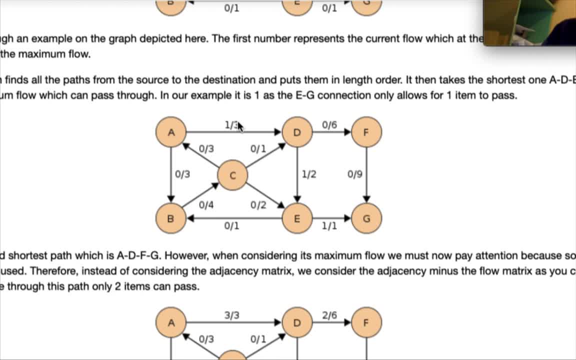 that not only you have a capacity, but this capacity may be partially busy. this capacity may be partially busy. this capacity may be partially busy at the meantime, as you can hear people at the meantime, as you can hear people at the meantime. as you can hear people are sending me tons and tons of messages. 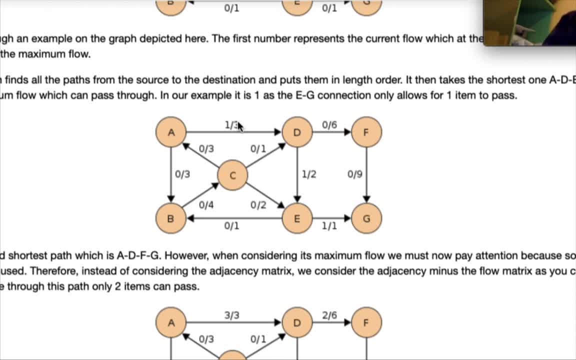 are sending me tons and tons of messages. are sending me tons and tons of messages. okay, this capacity may be partially busy. okay, this capacity may be partially busy. okay, this capacity may be partially busy. so, in order to determine what is the, so, in order to determine what is the, 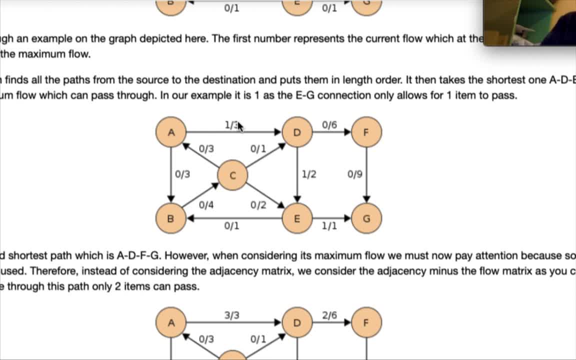 so, in order to determine what is the maximum maximum, maximum number of items you can send through you, number of items you can send through you. number of items you can send through, you don't have to use the adjacency matrix. don't have to use the adjacency matrix. 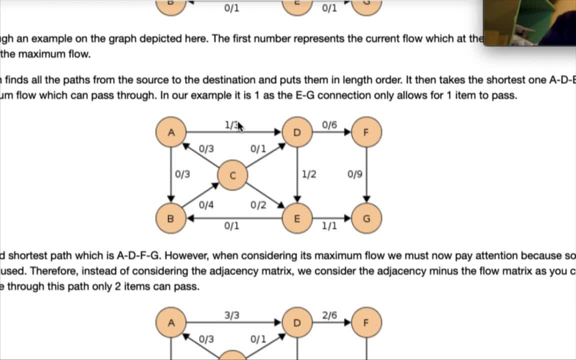 don't have to use the adjacency matrix as it is. as it is as it is, but you have to use the adjacency matrix. but you have to use the adjacency matrix, but you have to use the adjacency matrix minus the flow matrix. so three minus one minus the flow matrix, so three minus one. 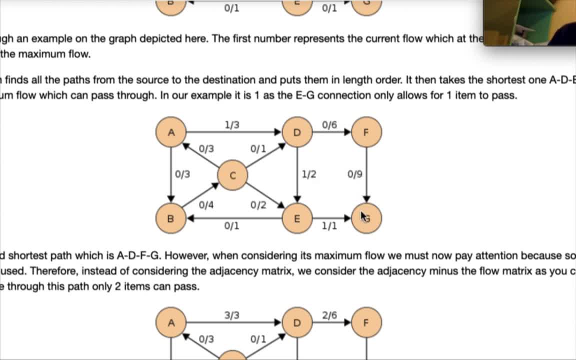 minus the flow matrix, so three minus one, six minus zero and nine minus zero. so six minus zero and nine minus zero. so six minus zero and nine minus zero. so here the maximum number of items you can here. the maximum number of items you can here. the maximum number of items you can send through is two. 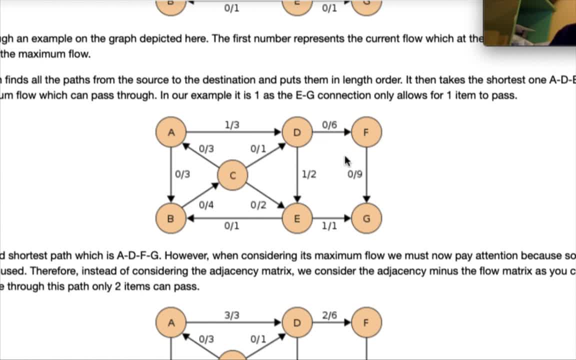 send through is two. send through is two. two here, two here and two here. you two here, two here and two here. you two here, two here and two here. you update the flow matrix and you get update the flow matrix and you get update the flow matrix and you get three, two, six and two nine. okay, so this. 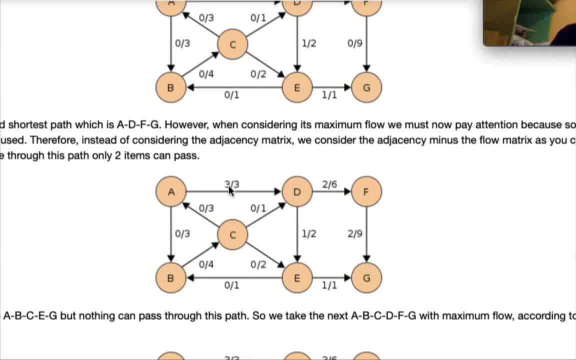 three, two, six and two nine, okay. so this: three, two, six and two nine, okay. so this is your current situation on the left of. is your current situation on the left of. is your current situation on the left of? the slash, the flow matrix on the right. the slash, the flow matrix on the right. 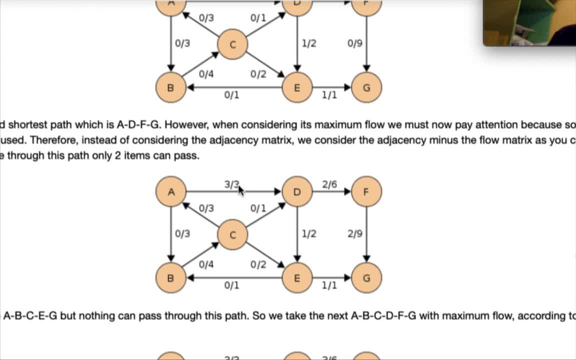 the slash, the flow matrix, on the right capacity matrix, capacity matrix, capacity matrix. let's see now another path a- b. let's see now another path a- b. let's see now another path: a, b, c, e, g, c, e, g, c, e, g, a, b, c, e g is a wonderful path. 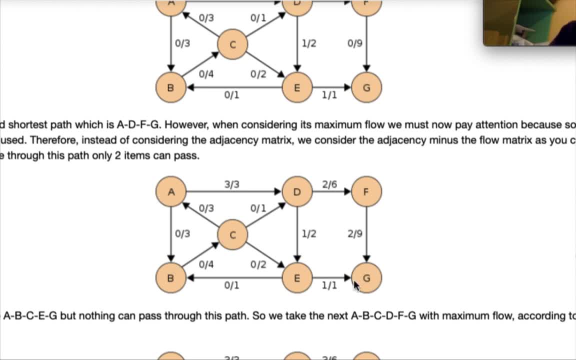 a b c e g is a wonderful path. a b, c e g is a wonderful path. however, a b c e g has a potential flow. however, a b c e g has a potential flow. however, a b c e g has a potential flow of zero, because here you can send three. 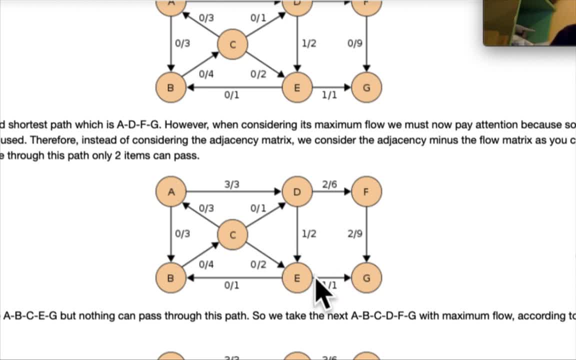 of zero, because here you can send three of zero, because here you can send three items here for items here for items, here for here two, but here none. here two, but here none. here two, but here none. to zero. you can send no items to this to zero. you can send no items to this. 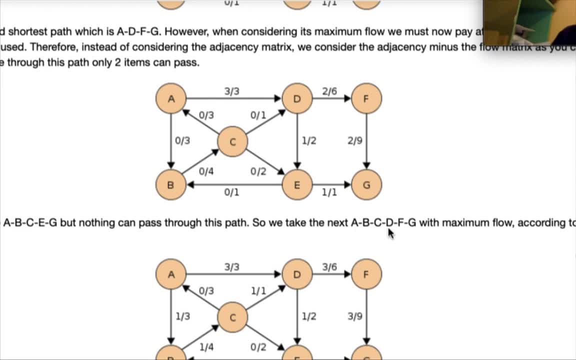 to zero. you can send no items to this path. path, path. so let's see another one. a, b, c, d, f g. so let's see another one. a, b, c, d, f g. so let's see another one. a, b, c, d, f g. a a, a, b, c, d, f g. 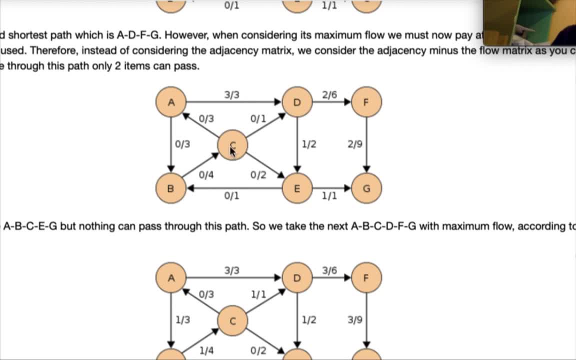 b, c, d, f, g, b, c, d, f, g, a, b, c, d, f, g, a, b, c, d, f, g, a, b, c, d, f, g. let's see three, four, one. let's see three, four, one. let's see three, four, one, four, four, four, seven. yeah, we can send one so you can see. 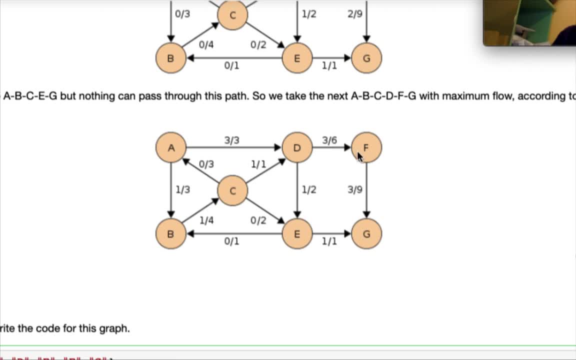 seven. yeah, we can send one so you can see seven. yeah, we can send one so you can see updated one. one, one, one, one. okay, we don't have any other valid path from a to g, and so the algorithm is over. so, at the end, this is what the algorithm must, what your, your best product allocation. send one item to b. 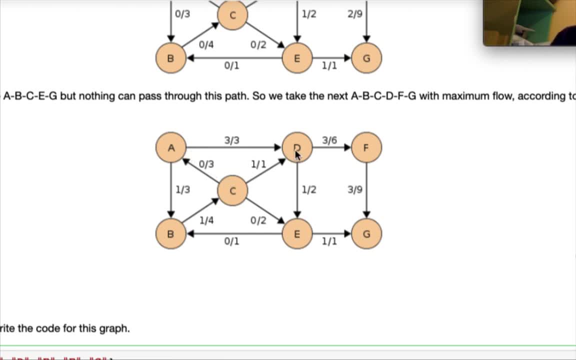 nothing to g. clearly you can't: three items to d. from b one item to c, one item to d. from d three items to f, one items to e. from e one items to g and from f three items to two to g. so you have four items coming out from a, which they correctly arrive to g. so four is the result and this is the. 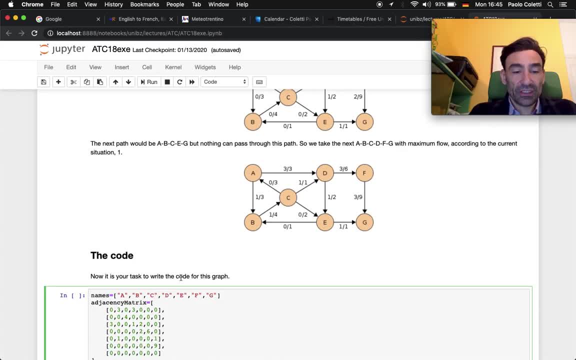 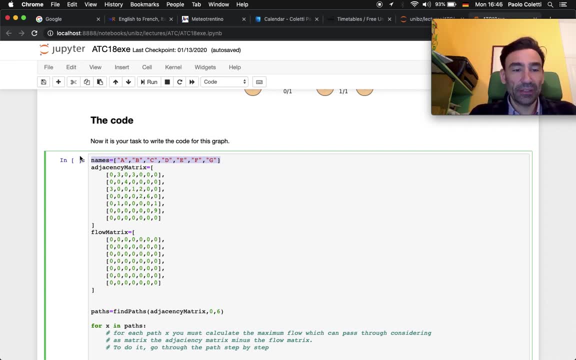 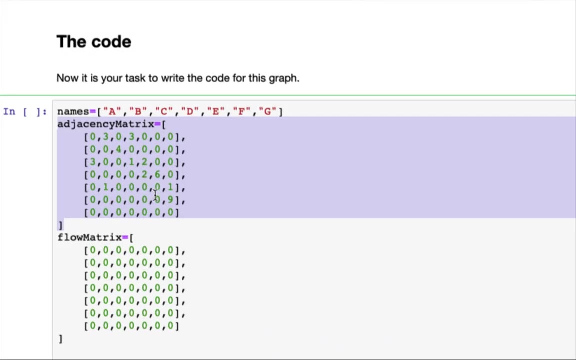 optimal path allocation. let's see the code for this graph. here i assign. i give the names because i will ask you to write things in human readable way. the adjacency matrix, this time is not symmetric, as you can see, still has zero on the diagonal, but it's not symmetric and it contains the maximum capacity. so the number of drivers that you have at 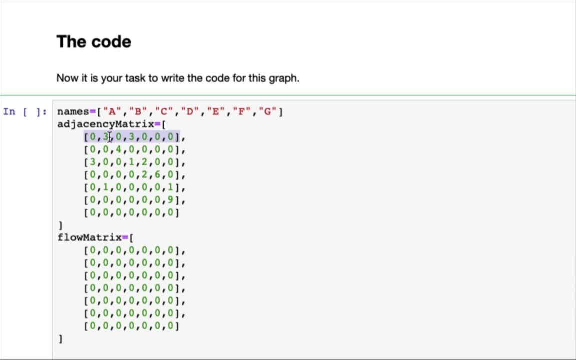 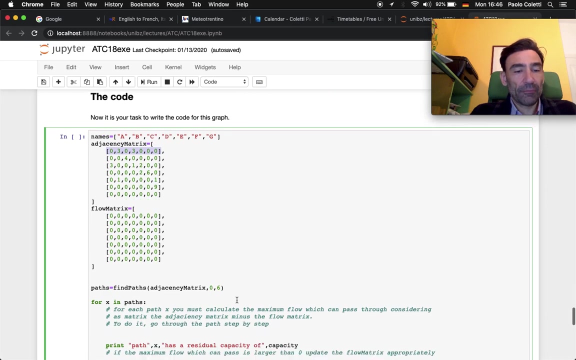 each node. for example, at node a, you have three drivers which can go to b and three drivers which can go to d. at node b, you have four drivers which can go to c, is it correct? yeah, okay, the flow matrix which starts with zeros at the beginning. you don't send anything. can you see? first step. 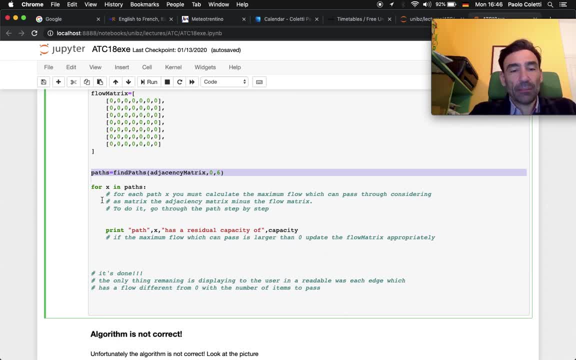 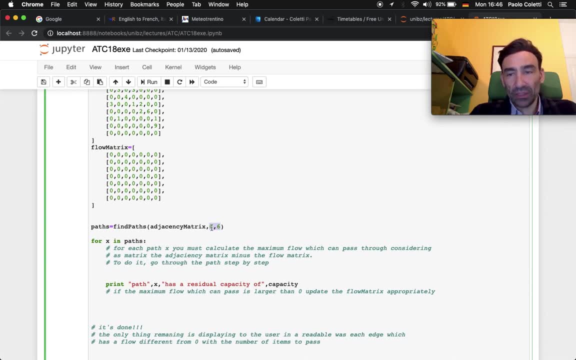 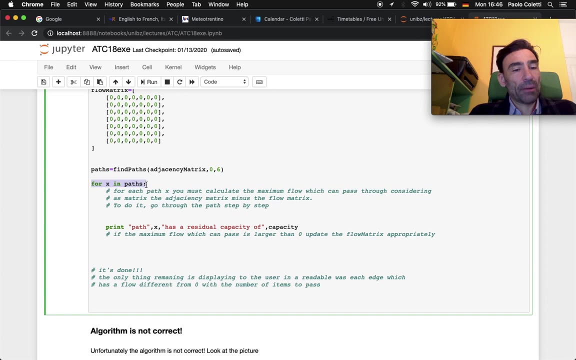 i get all the possible paths and then from zero to six, so from node, from node a to node g. i must speak pythonic here and i go into path. okay, then i loop on all the path for x in path. for each path, you must calculate the max, the maximum. 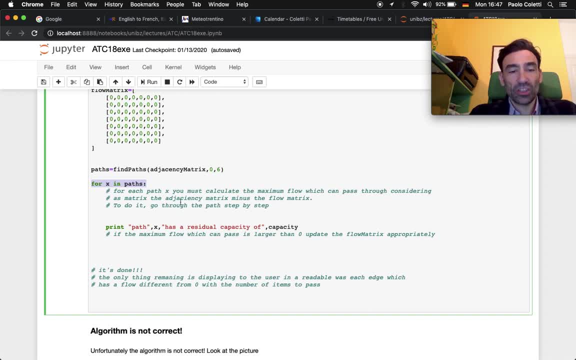 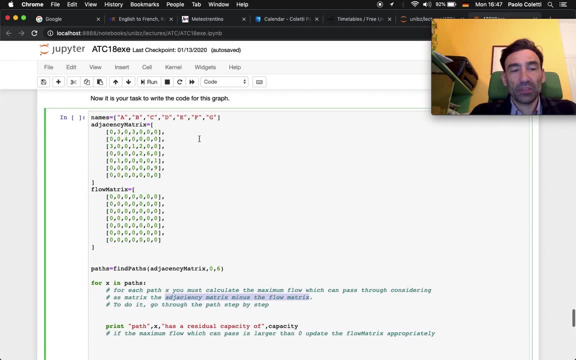 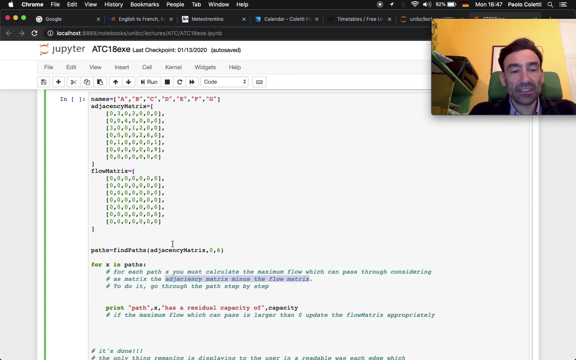 flow which can pass through, considering, however, as matrix the adjacency matrix minus the flow matrix. so you consider the adjacency matrix, but you can directly make the subtraction. i think, however, you can make it element by element if you prefer. this matrix minus flow matrix at the beginning is the first step, is not necessary because flow matrix is full of zeros, but when you will have 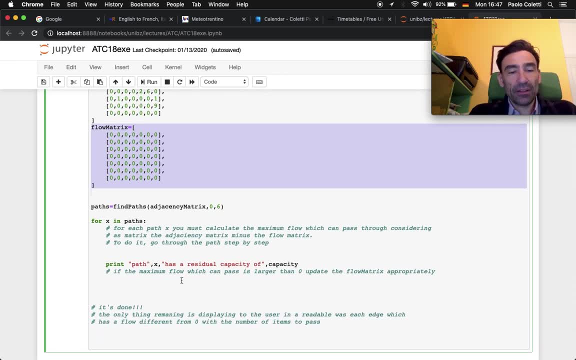 some flow. okay, so considering this step, okay, you take the path, you go through all the elements of all the steps of the path and you check in the adjacency matrix minus flow matrix, how much can you send through? you can find out the minimum of all these numbers. okay, and this: 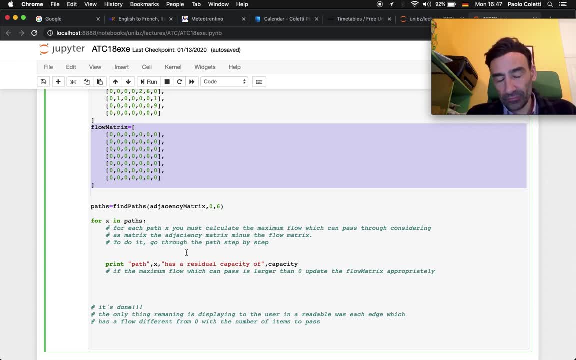 is how much you can send through the the path. okay. if this minimum is zero or even negative, well stop, you can't use that path. if this minimum is positive, okay i. i write this for debugging purposes. path x has a residual capacity of. okay, if this minimum has some capacity, so larger. 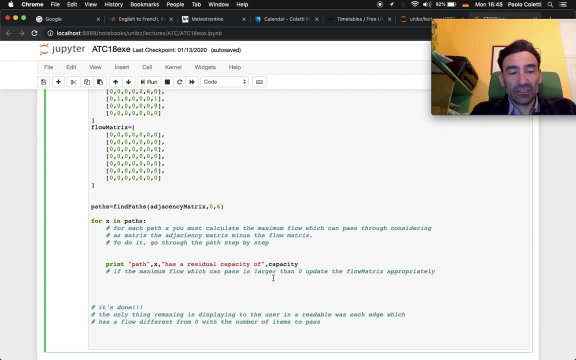 than zero. very well, you will consider it okay and just update the flow matrix. you don't need to remember it. you just update the flow matrix in the corresponding point, you go to the path and you add the number to the flow matrix. it's done. you will go through here, all the path, done, nothing else. 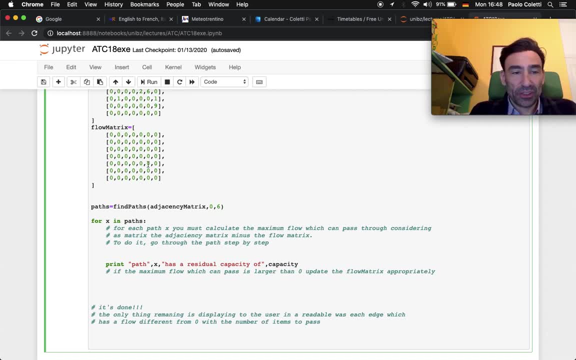 the only thing remaining is displaying the output. so you will display the flow matrix. please, i ask you a human, readable format. so whenever it's zero, don't tell me anything. if it is not zero, right from node this one to node that one, send dot items okay. however, i have to tell you a very sad thing: target is wrong. 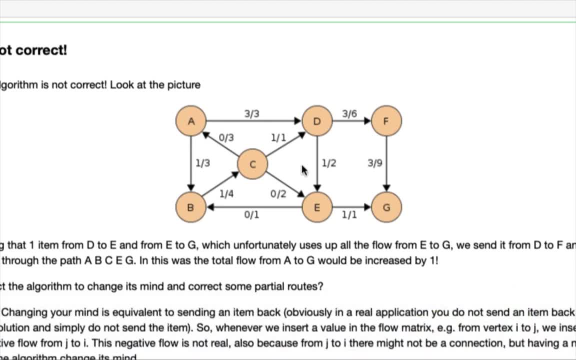 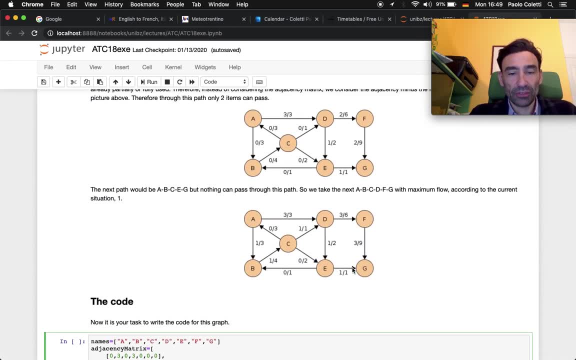 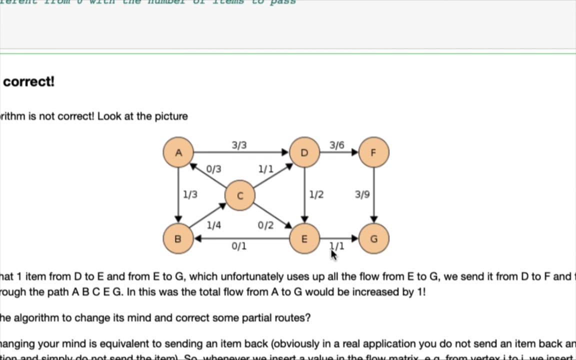 look at the picture. look at this picture. this is ours. look now. look and compare it with our solution. look in our solution, not three, four, yes, okay, now, this is our solution. of course it's our solution. okay, okay, it's our solution. however, imagine that if this item, which goes to: 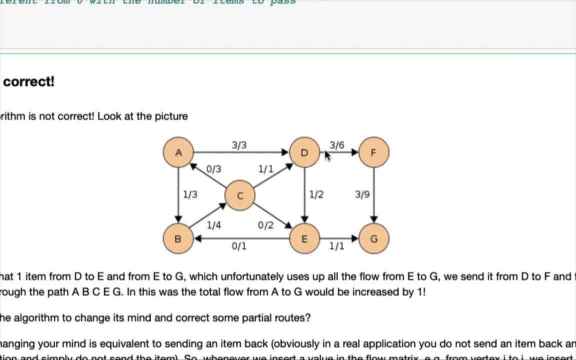 e and then goes to g. if i send it to f and then to g, if i send it to f and then to g, this will be four, and this will be four, and this will be zero, and this will be zero. in this case, with this one zero, i. 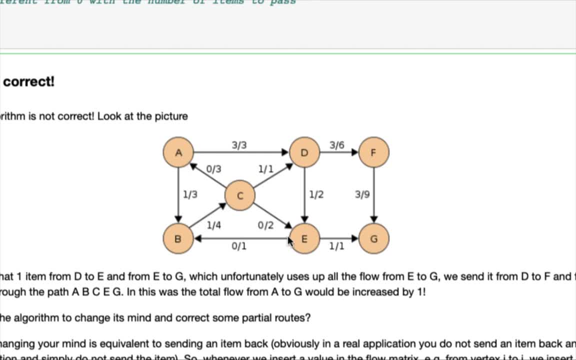 send an item to a, b, c, e g, a, b, c, e, g. so if this were zero, i could send an item here and four items will arrive in g. so if this item which goes from d to e, i send it instead to f and then to g, it will. 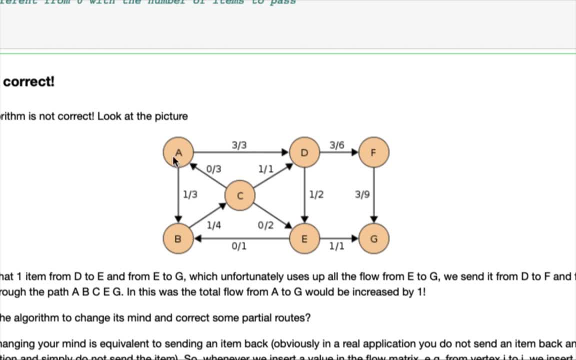 free this slot here and i could send a new item a, b, c, e, g. so this is not what the solution is going to be. we found is not the best one. why it's not the best one? because the algorithm that we have built is not able to change its mind, so to certain way correct itself to send the item back here. let's. 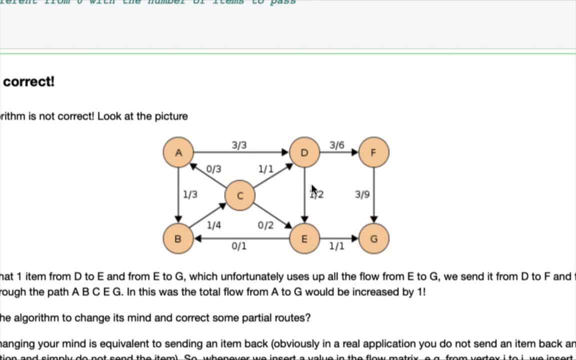 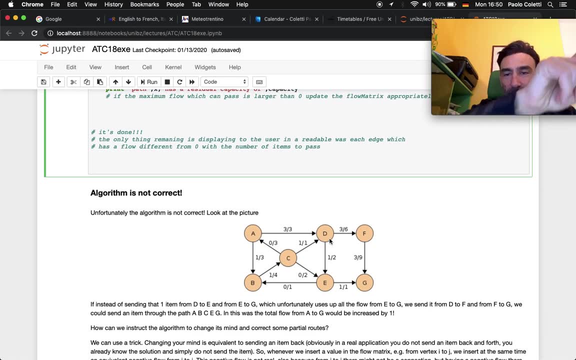 say: it would be nice if, at this situation, we could take this item, send it back to d, back back. okay, send it back to 2d and go through f and g. okay, in practice you don't send it back, you simply don't send it at all from d to e. so, if so, the concept. 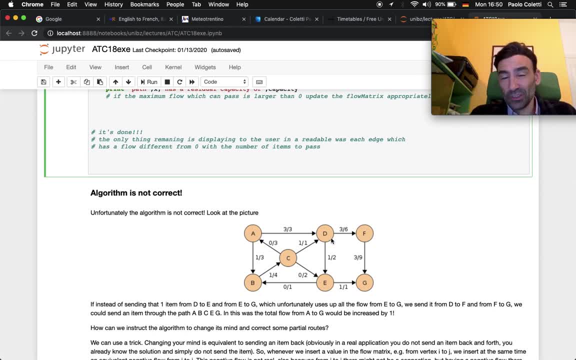 of sending back is just height for herself. practice: you don't say you don't have the driver going forth and then when he comes home he carries back the item. no, or especially because it's impossible, it's not allowed to send back. so in practice, sending back doesn't mean that the item is effectively sent back. it means simply that time 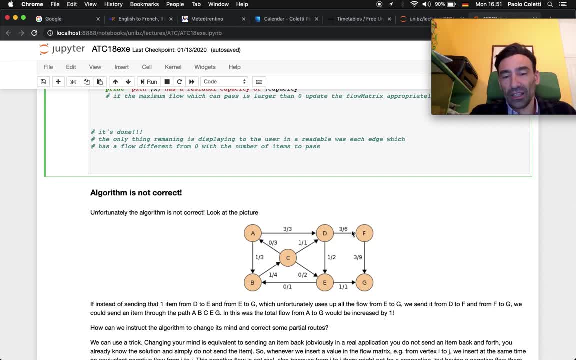 is never sent from d to e, stays in d and must go through another route. if the algorithm could correct itself in this way, it would find the best solution in this case and i can guarantee there is a mathematical theorem that tells you that it will find the best solution in all cases. okay, how? 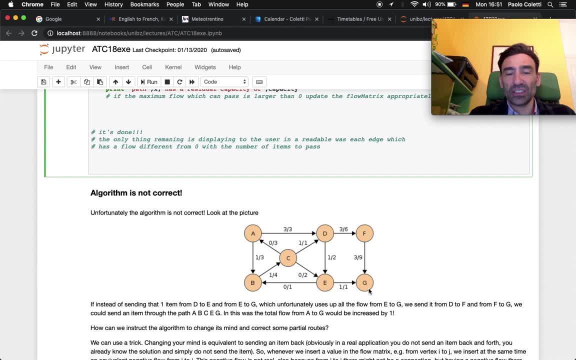 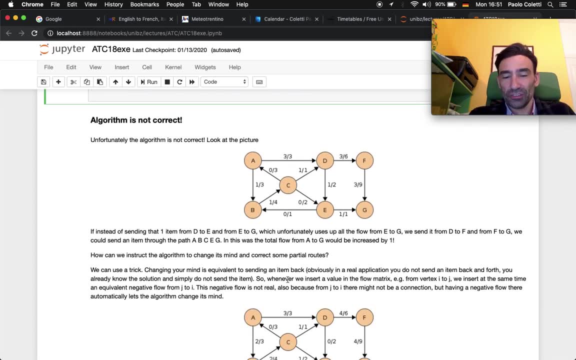 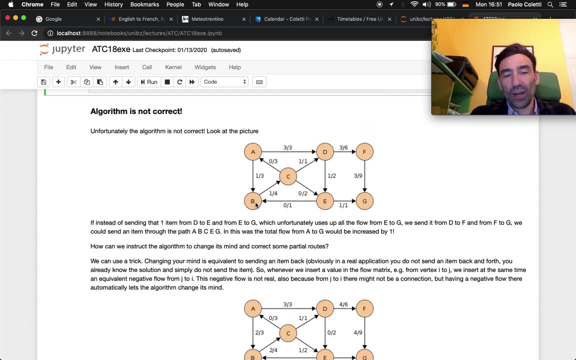 can we modify the algorithm such a way that is so intelligent that sends things back? well, it may seem strange to you, but there is a little trick which, when i saw it first time, i say doesn't work, but it works okay. whenever you send something, for example one item from a to b, you insert in the 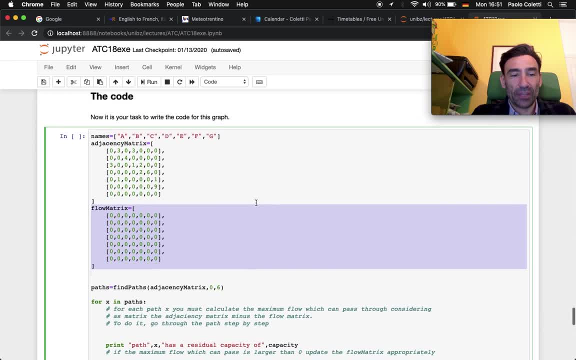 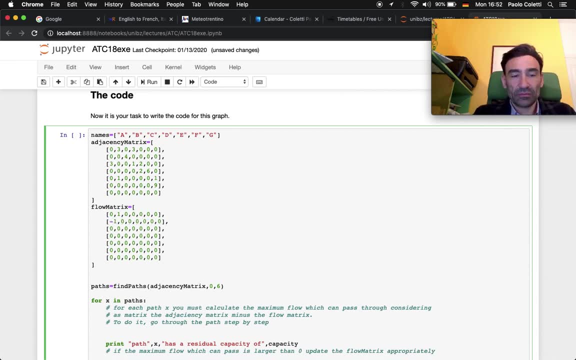 flow matrix correctly that you have sent one item from a to b and you insert in the flow matrix a to b. so here okay, but you also insert here minus one. it's just for technical reasons. if you insert that minus one, i can guarantee that the algorithm written exactly as it is. so you just 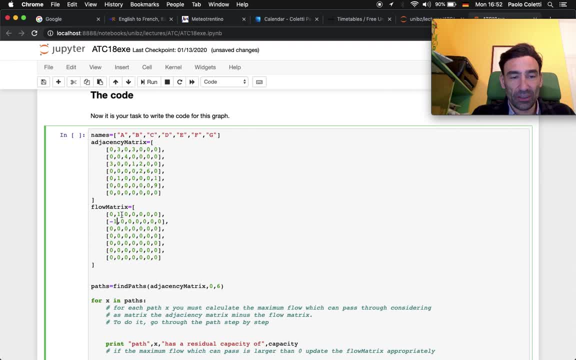 need one line of modification. so whenever you insert something in the flow matrix, if you add a plus three here, for, for example, you automatically add a minus three here in the symmetric position, if you just this little modification, you the algorithm will be able to correct itself, because 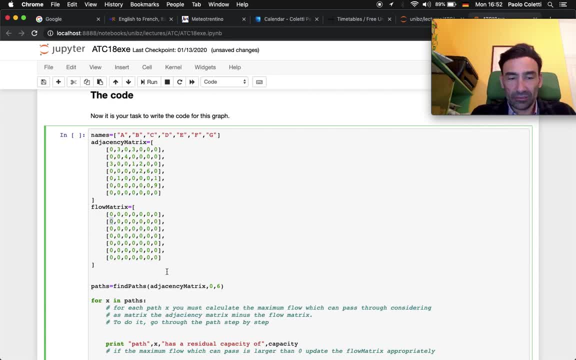 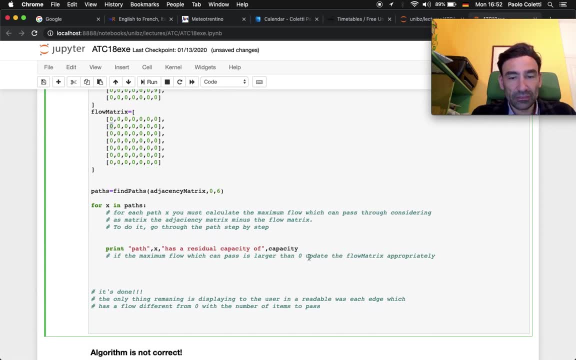 it finds a minus one and will be able to send items back. okay, we'll be able to find. so just one line of modification here. where is it here? when you update the flow metrics appropriately- the items- the algorithm will be able to find the correct solutions every time. so we'll be able to certain. 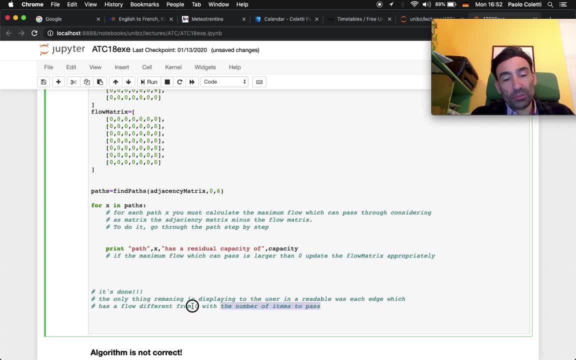 point of view correct itself. Obviously, when you print a solution, please don't tell me also the negative flows, which are there only for technical reasons. Just tell me the positive flows. Okay, Okay, That's all, Goodbye. Late addition. 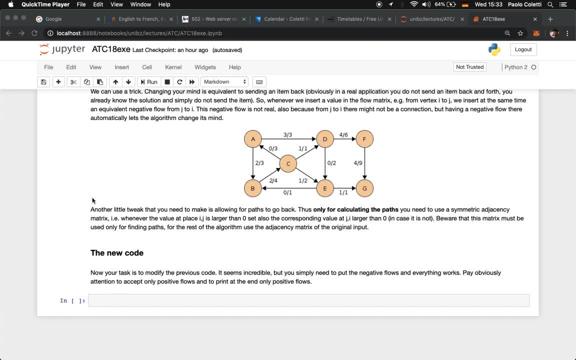 Well, it's not enough that you just mark any flow also with a negative sign in the opposite direction, because you must allow also your algorithm in a certain sense to go back. So you must allow also your algorithm to push back some items. Okay. 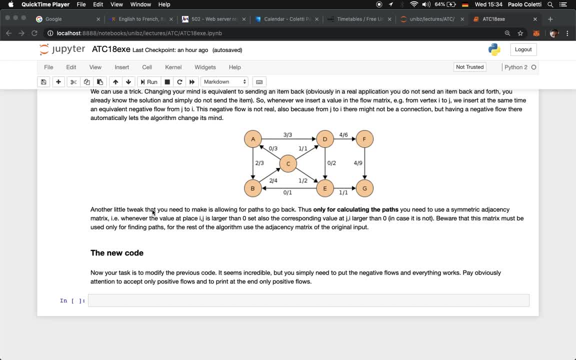 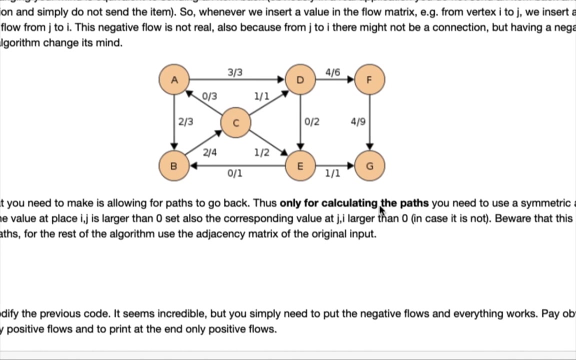 So this means that you need another little tweak, only for calculating the path. Okay, And only for calculating the path. you must build a new adjacency matrix which is symmetric. It means you take your original adjacency matrix. Whenever an element at ij is larger than zero, you set also the corresponding value at ji larger than zero, in case it is not. 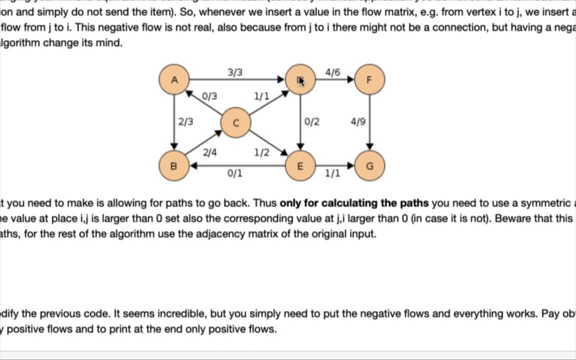 Okay, In this way, for example here you usually allow a flow from D to E. Okay, This way you will allow Also a counter flow from E to D, because you need to push the items back. also, I repeat, in real life applications it's not pushing the items back. 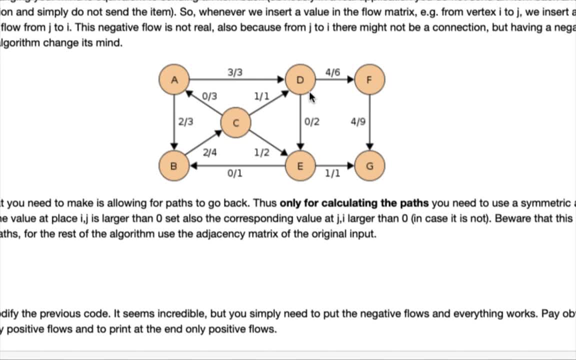 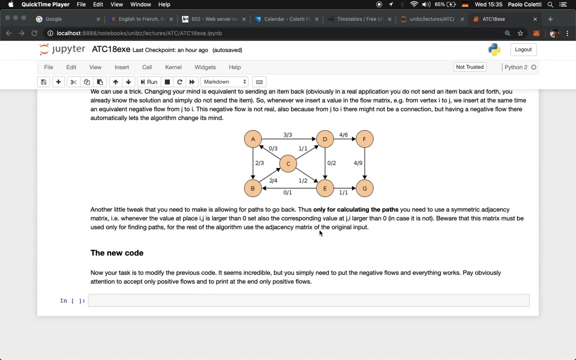 Well, unless you have a really bizarre logistic. but it's simply not shipping the item. So only for calculating the path. you need also another little tweak: Change the adjacency matrix, the adjacency matrix and make it symmetric. Okay, Calculate the path and then, for the rest of the algorithm, use the original input adjacency matrix.